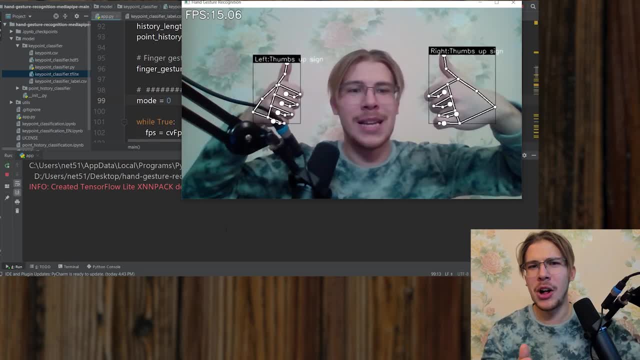 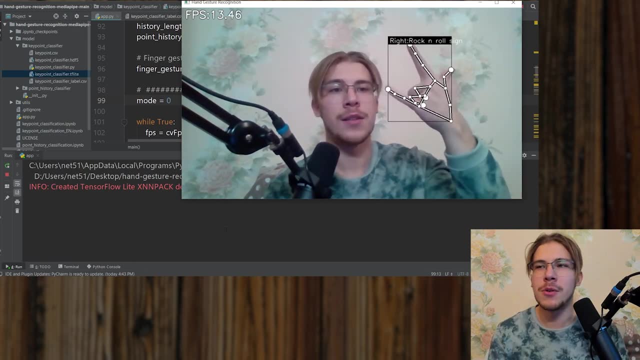 but yeah, I mean it's, it's gonna be pretty interesting and, above all, I would say like it's a- and we are really really beginner friendly video. so if you have like a project for I don't know, for college or whatnot, and and and you're, or like it's just like a personal thing, you're learning more, I'll keep. 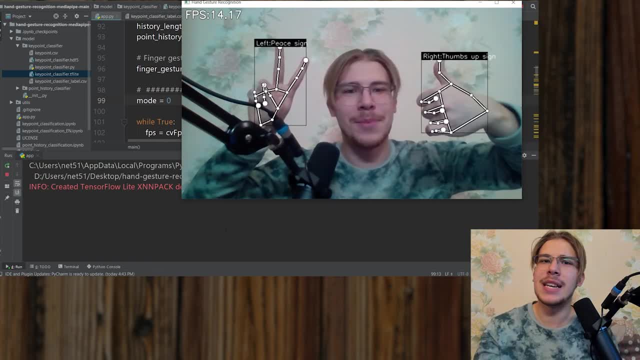 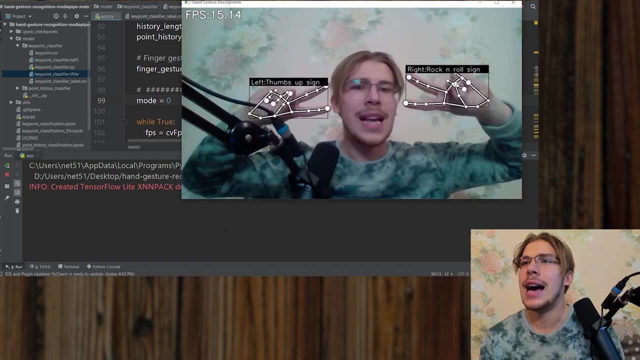 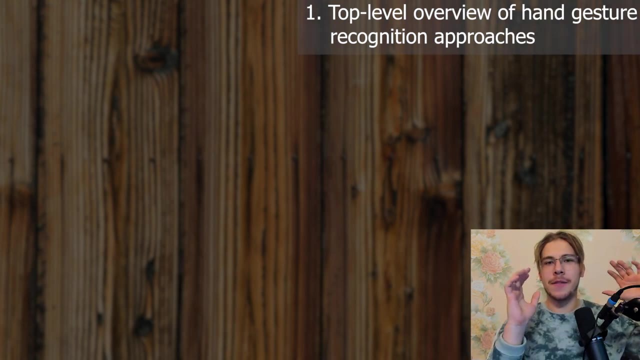 it like very beginner friendly and as long as you have like basic knowledge of Python, like basic knowledge of how to like install modules and do things like that, I think it'll be good and yeah, so now let's talk about the structure of what's going to be in the video. so the first 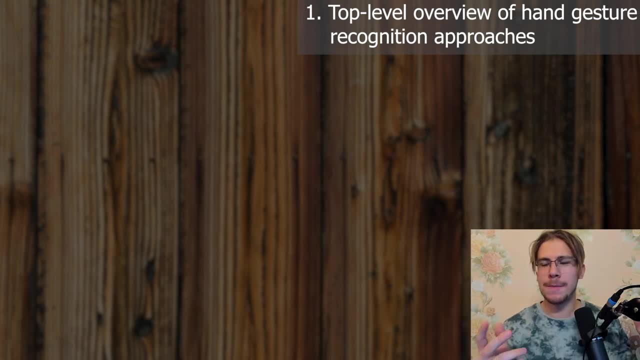 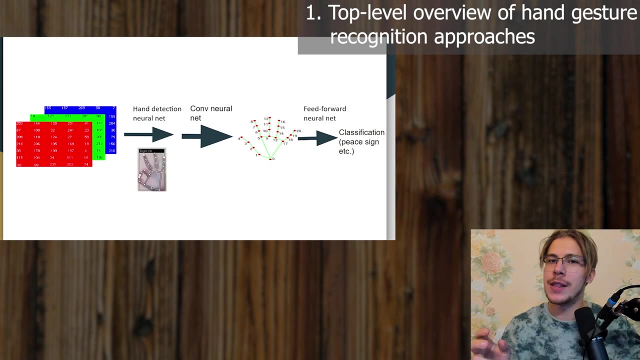 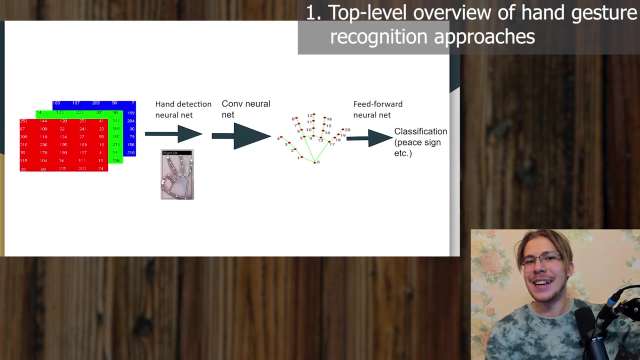 thing we'll talk about is kind of like the top level overview of the, in my opinion, like two main approaches that that you can take when performing hand gesture recognition: the pixels first approach and the landmarks first approach. uh, we'll do that in like a very fancy google prezo that I've put together in like 10 minutes, but it's gonna be. 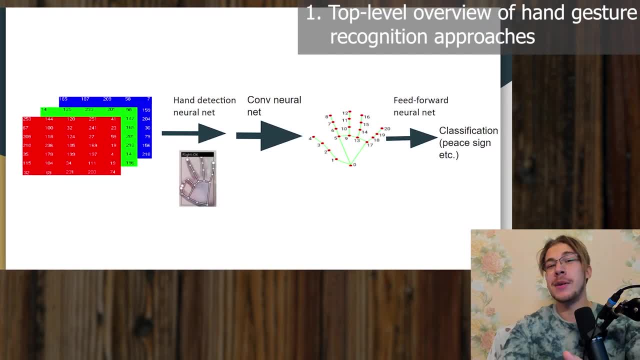 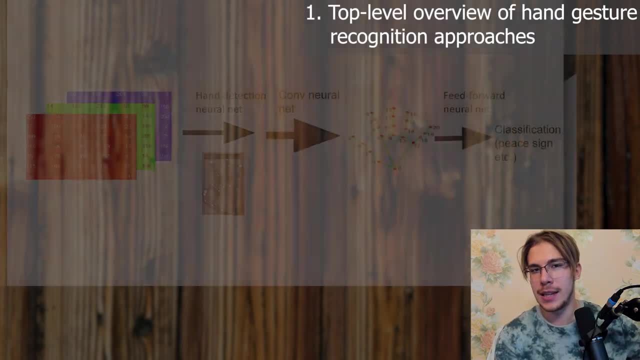 good, we'll kind of cover all the main like ideas that you need to know. so that's like when we jump into code, if you're like, uh, you know that you have a way of understanding why things are like organized there the way that they are, then once we have that sort of like top level understanding, 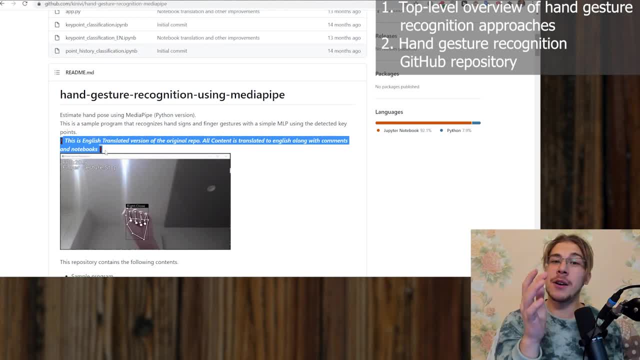 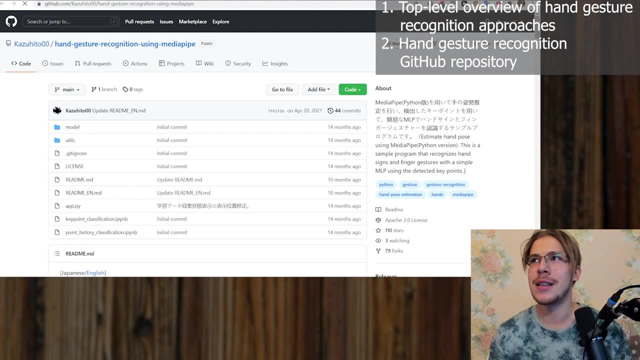 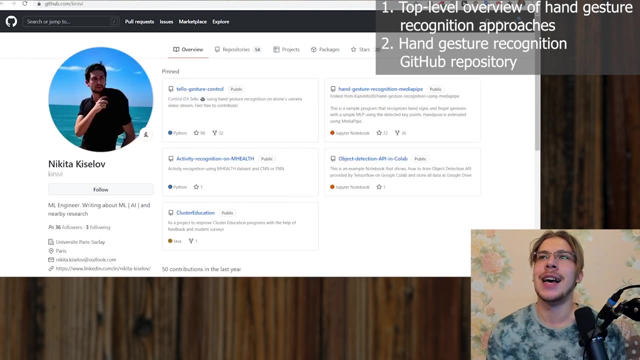 of the different approaches there are and stuff like that. I'll show you like a really cool repo that I found in its english translation that makes it really easy for us to get started with hand gesture recognition and training something uh on training it- training like a neural net and custom hand gestures- and that repo uses google's media. 5. 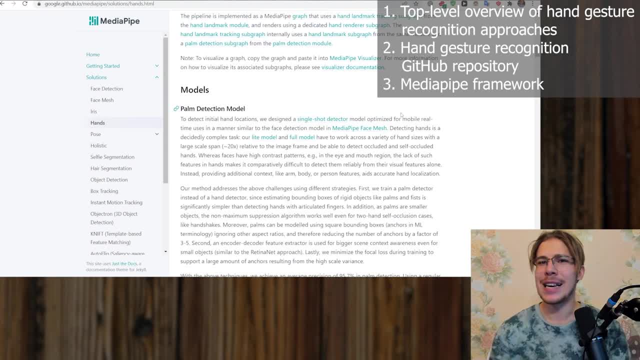 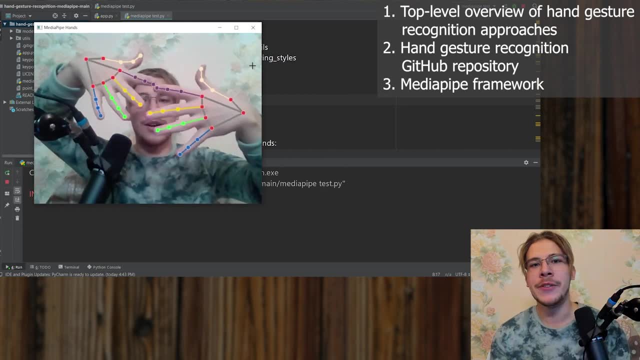 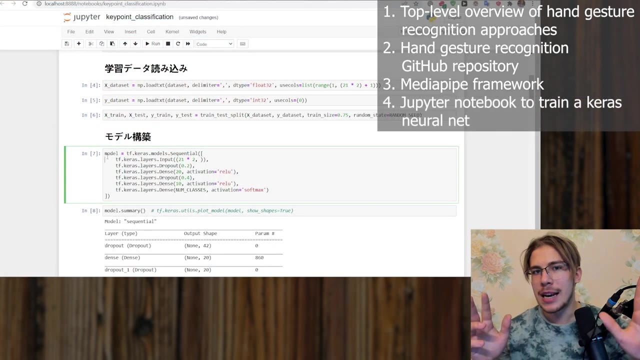 framework and that's like a framework that you people install in python and it has like all sorts of really nice things that make it really easy to get started with. you know, this type of like computer vision tasks, and then on top of google media pipe there's like a really really simple carousel network. that that takes like hand. 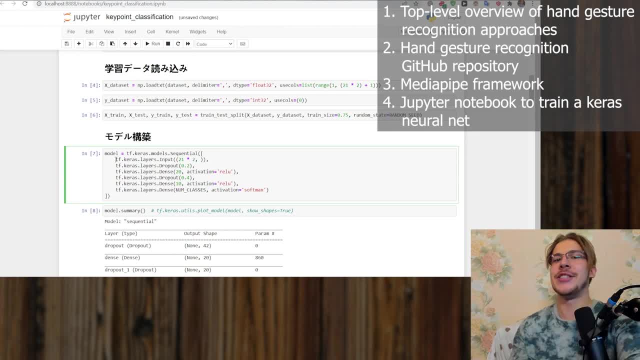 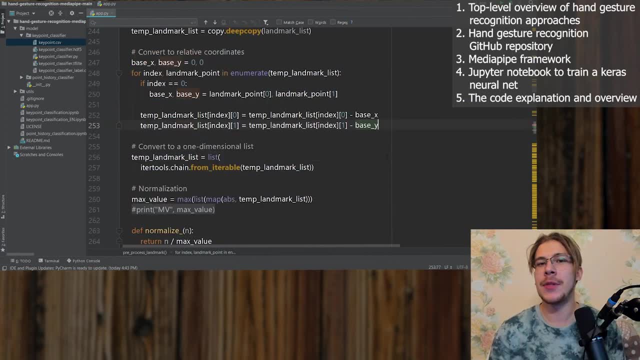 landmarks and uh classifies them into their actual gestures, which we'll. we'll cover all of that and then we'll look at the code and how we can like use the repo to train something on our custom gestures. but all but I'll also like walk you through the, at least like the interesting parts. 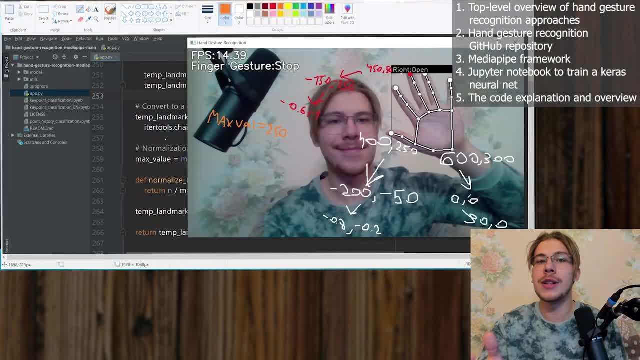 in the code that it might be useful for you to know. if you want to like take this thing and like modify it and build it, build it into some of your own projects or maybe build something like completely new, it might. it might be useful to kind of know. 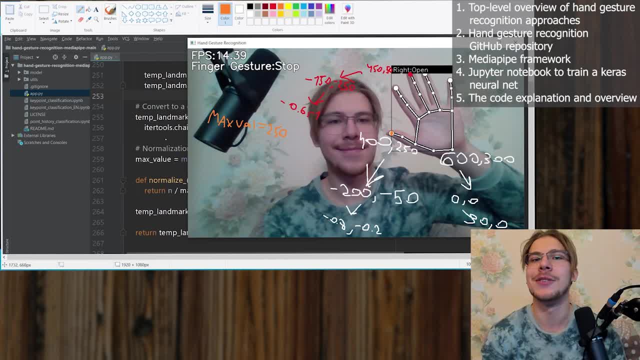 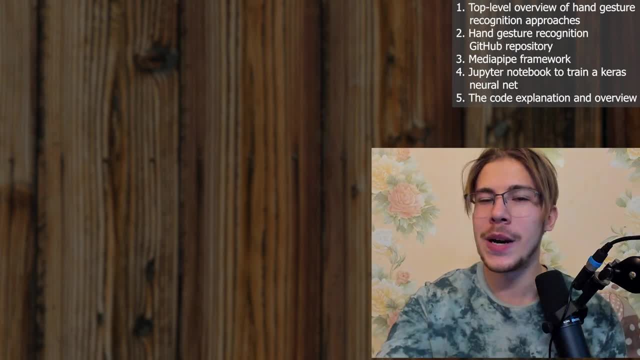 where some of the like main magic is happening, so to speak. so, um, if you're excited, you know, smash that like button. um, consider subscribing to the channel if you like it and, as always, like if you have any questions throughout the video comments: what whatnot? just like? leave them in the comment. 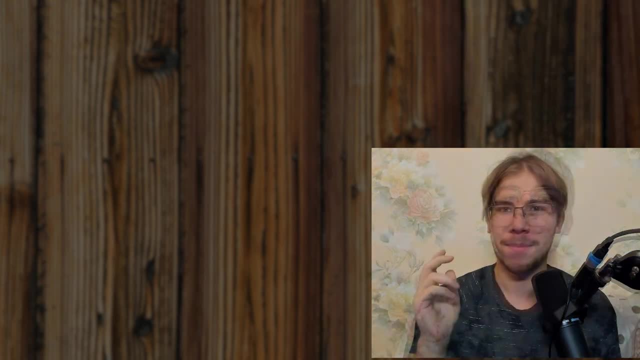 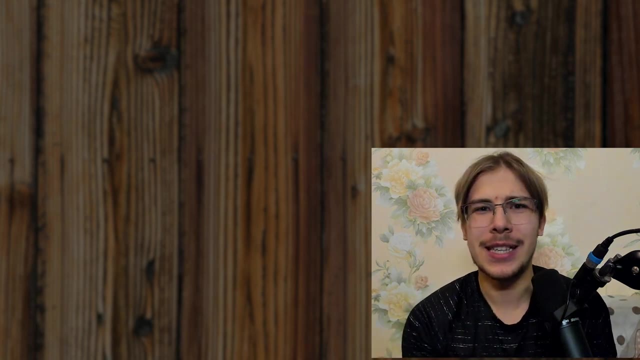 section down below and let's get started. hi again everybody. um, it's Ivan from the future, actually to tell you two things, and the first thing is that like it's gonna be a slightly longer video than usual, but like I really enjoyed the like in-depth, like in a coding- explanations and the 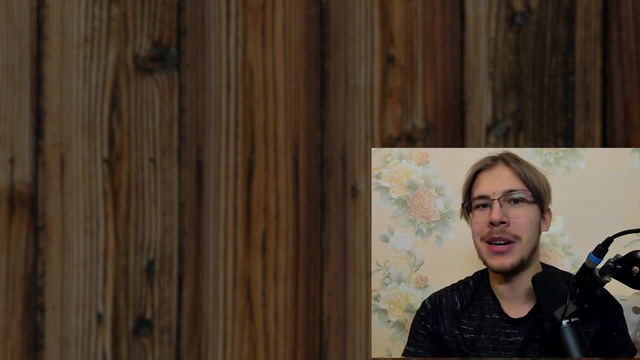 training explanations. we'd have to, so hope you'll enjoy it. but, like, if you want to skip to any specific part of the video, I'll leave the timestamp. so like, feel free to jump around that. that, that, uh, I always find that useful, so hopefully, like you'll find it useful too. and then there's like: 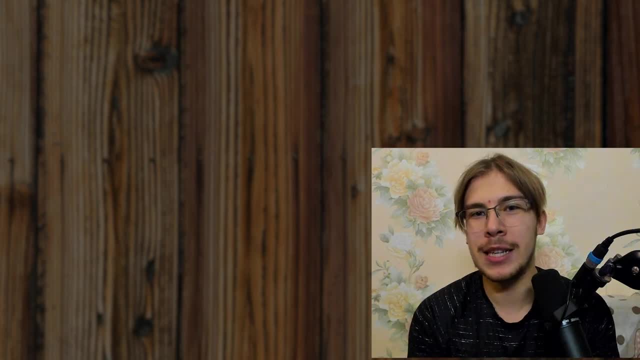 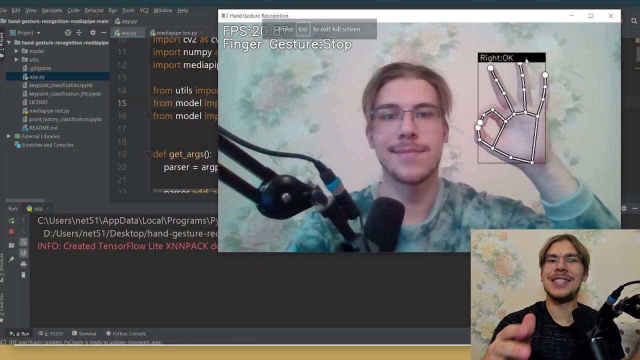 this little fragment where I explain the top level of how everything works and get recorded properly. so I'll just like quickly record it and then proceed normally with the video. so so let's talk about the top level understanding of how things work in the repository and how we can approach building such a system that you know. 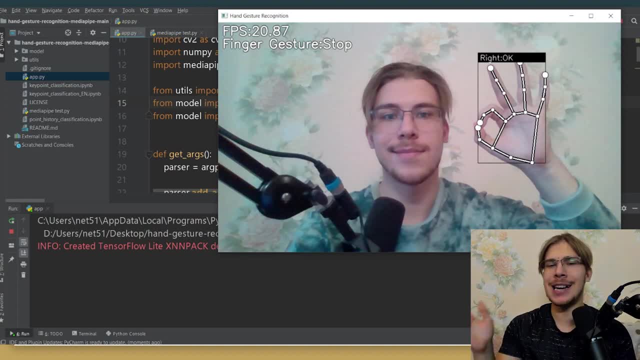 grabs the frames from the camera and recognizes the hand gestures in in those frames. so the first kind of part that needs to be handled is like the actual part of grabbing frames- like in my case it's from the webcam, uh- and grabbing them in a way that we can like interact with them and work with. 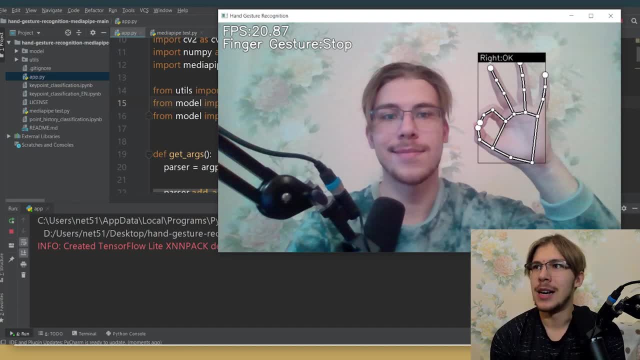 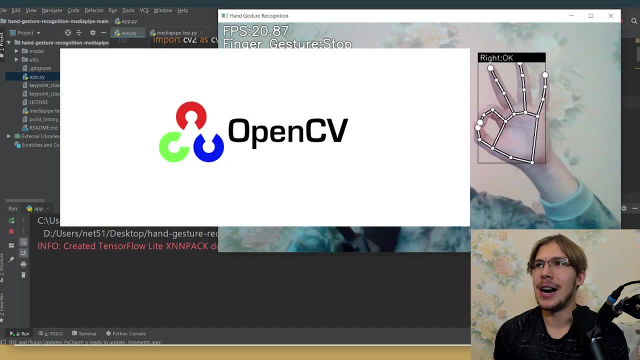 theляется in� using the original project and the LEO, which we saw in like ducks să and lost in the repository by really powerful, really cool uh, I enjoy working with it a lot. uh, A library called open CV or like open computer vision, um, which is like, which is like also kind of you know, good news. 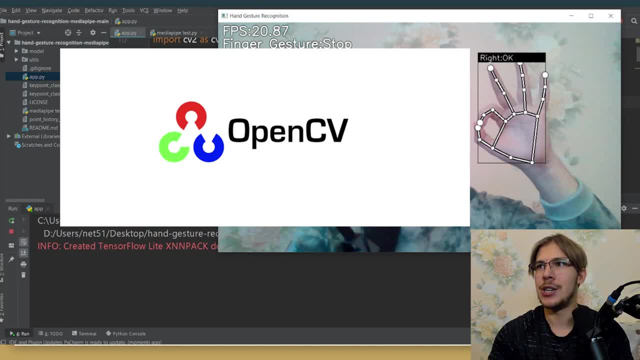 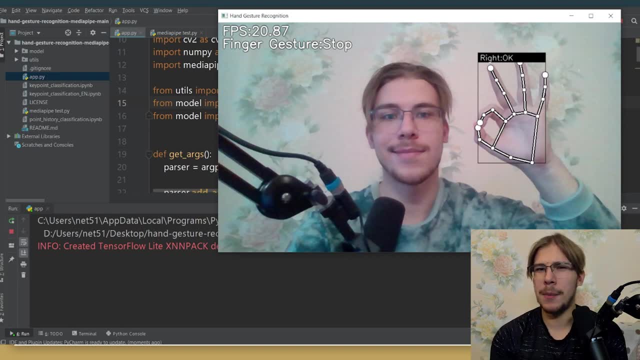 that it's using that because it's gonna, you know, be pretty easy for you to build it into your own page projects, because it's like such a widespread kind of such a such a massive library, used in so many places, really powerful, really cool. know building such system to recognize certain hand gestures, like you know, like the peace sign. 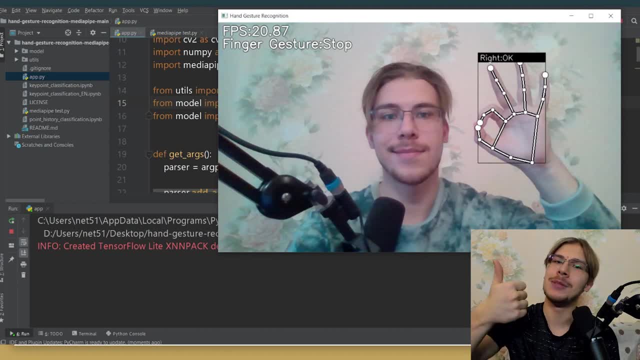 or the i don't know the okay sign, the thumbs up sign, i don't know, i just did that, uh, but i know way, uh. or like the um rock and roll sign, or something right. which i wanted to say is just like, if any of these gestures like don't mean to you exactly what they mean to me in some part of 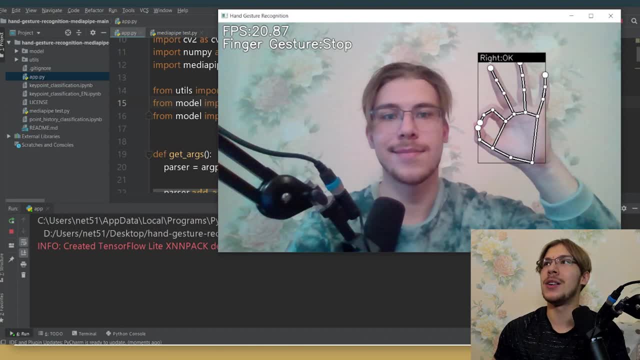 the world because, like i know, they can mean different things around the world, kind of, yeah, it would be funny. uh, just let me know. pretty sure it shouldn't make anything do crazy, but yeah, like let me know if some of the gestures that i'm showing, like if they mean something differently. 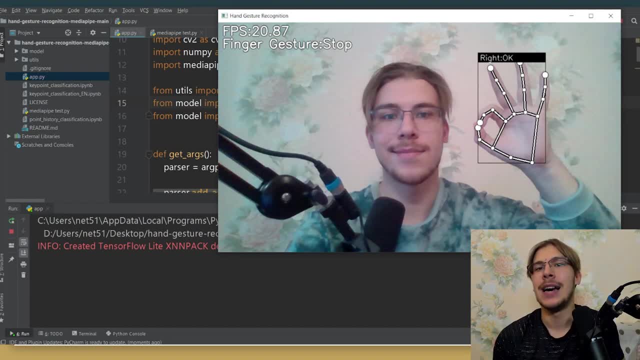 i think it would be like a nice educational thing. i guess um so cool now that we talked about like kind of this first part of the system that's grabbing frames, you know, uses open c for that- um, how do we actually build like the, the main kind of crucial system, system that's capable of 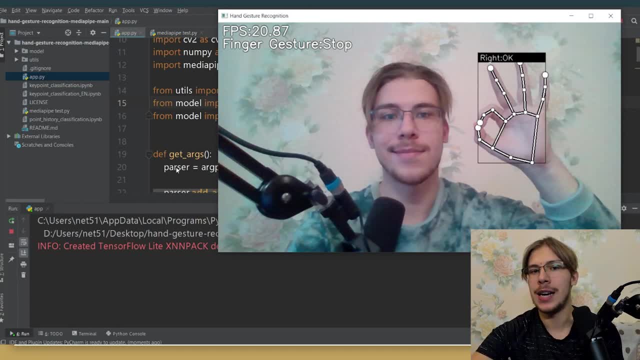 you know, taking, taking, you know some of these frames and actually like, like all the drawings, like all this, like little pointy, like dots here, like labels that that's open cv. how do we actually handle? this? is the system that's recognizing the hand gestures. um right. 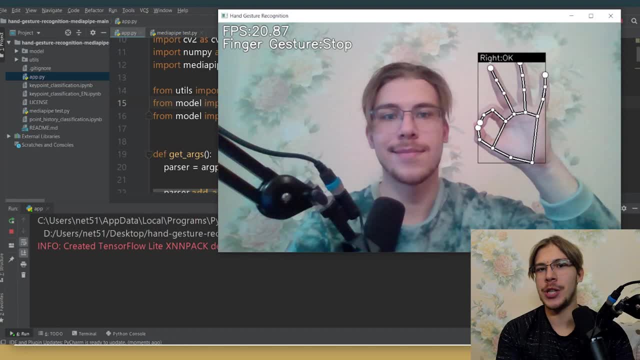 so the first kind of hint that we can take at how we can approach solving this problem is by thinking, like you know, we had frames with with hands right, like hands can be all sorts of different shapes, gestures can be all sorts of like different shapes and different. you know, i don't know. uh, people can. 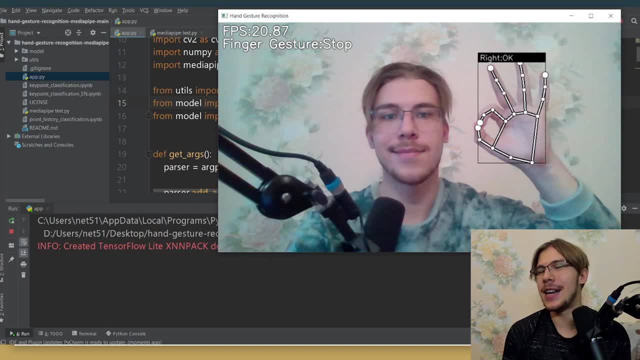 have different hands that are doing different hand gestures, with different slight variations and different slight, you know specifics. backgrounds can be different, lighting can be different, like all of this is kind of hinting that it would be really, really difficult, if not impossible, for a human being to write like a comprehensive system, uh, like just purely algorithmically, with. 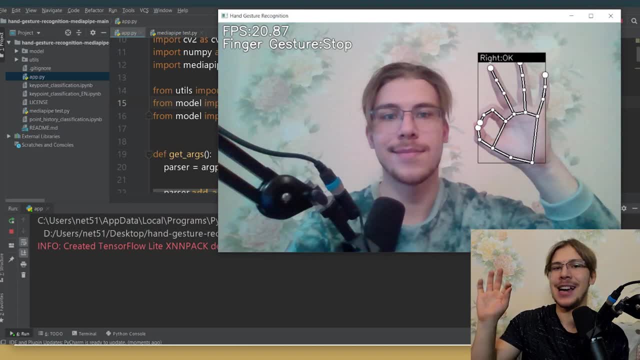 code that would be able to tell us exactly which hand gesture it is right. so, this being like such a broad task, with like different ways that the gestures can be presented, different backgrounds, it's kind of hinting that we should use a machine learning approach. or you know, as we'll soon talk, 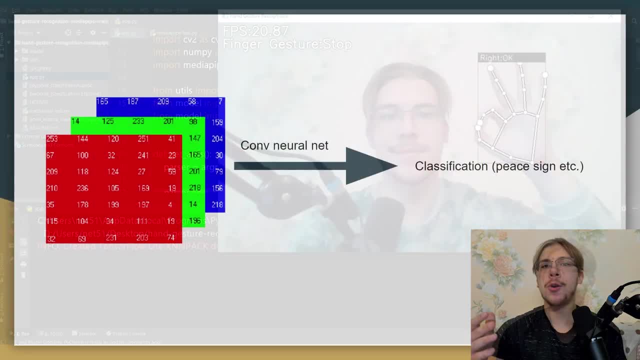 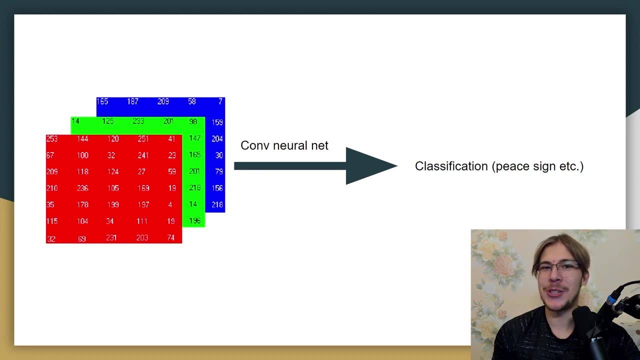 about like a deep learning approach, like in specific, so the first machine learning, or, as we've talked about, more accurately like deep learning, because it uses, like, uh, deep neural networks approach is something i would call pixels, first approach, uh, and that's because we're grabbing, like, uh, we were taking the rgb matrices, which rgb matrices like it's essentially, you know all of the 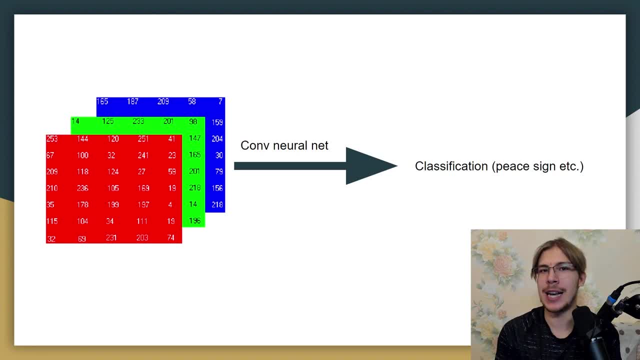 frames, uh, all of the frames that we're using and we're taking the rgb matrices and we're taking like all the like images are represented in computers as matrices, at least, like you know, it's a very like, well-known format of like an rgb, rgb matrix, um, and we pretty much can get that by. 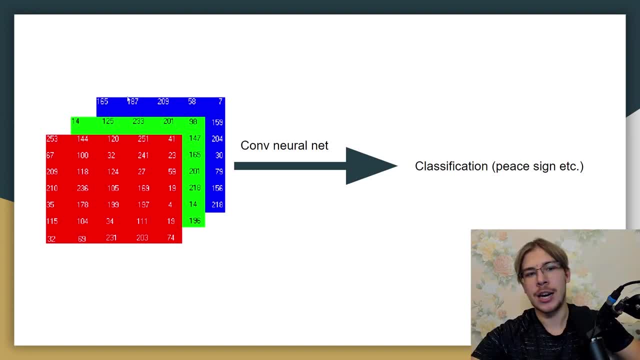 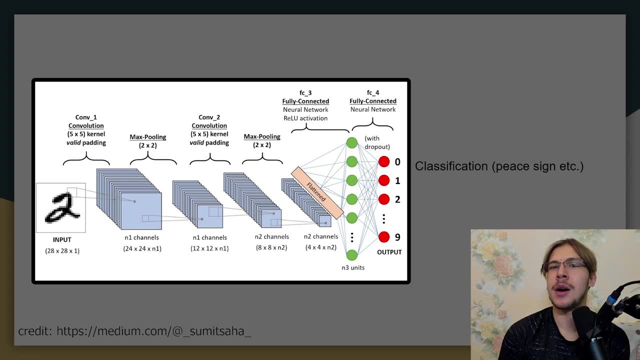 with openc by like grabbing frames from the webcam. so we get like this rgb matrix which you know contains pretty much all the information that's in the image. we pass that through a convolutional neural network, which is a special type of a neural network that's optimized to work specifically well. 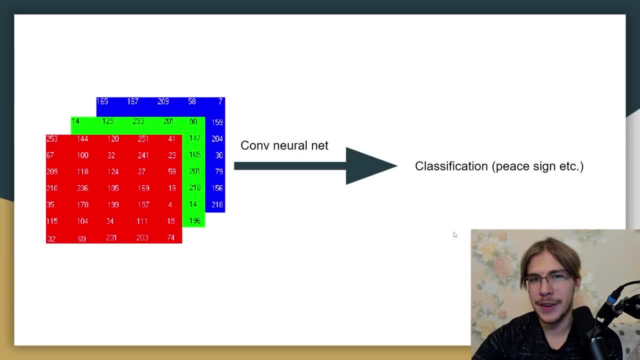 for images and we get the rgb matrix, which is a special type of a neural network that's optimized, some sort of classification, so that would be like the pixels first approach. okay, and that's the part where i hand it over to the ivan from the past to continue with the video, and so that's approach. 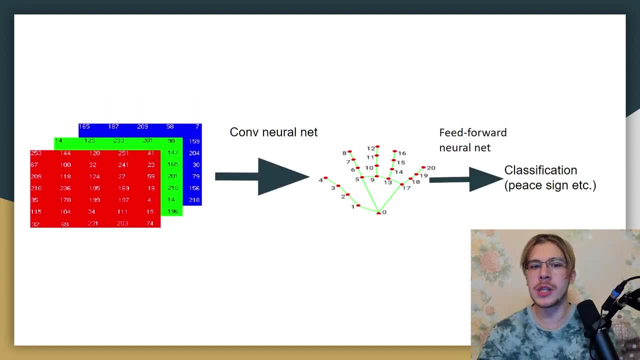 number one um. the second approach is: it's a little bit more multi-layered, but it starts off very similarly: we take um, grab the frames from the camera and pass them through a kind of network, but but this neural network is different. this one is not supposed to give us the definitive like. 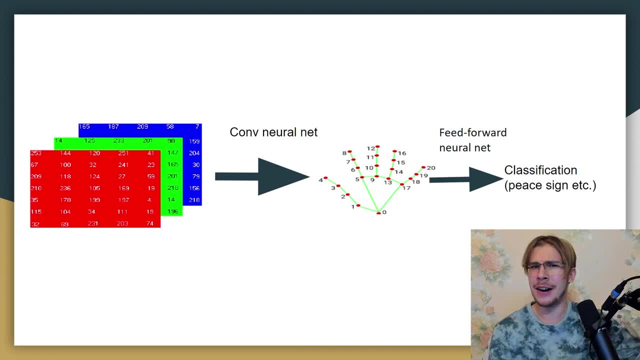 answers to what gesture they have to do. so we're going to use the rgb matrix, which is a special type and the hand in the frame is showing, but it's supposed to extract um hand landmarks like this kind of pointy um skeleton looking thingies of the hand, uh, and then we take those landmarks and 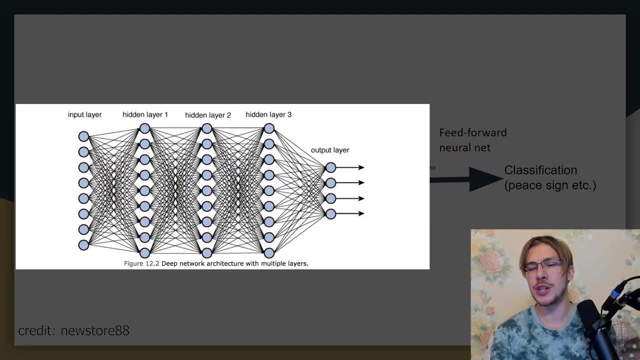 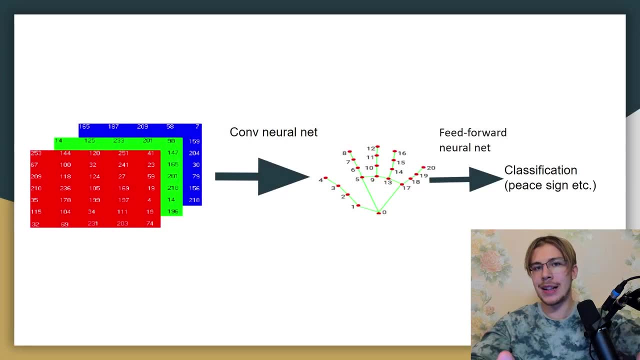 we pass them through another, much, much smaller and much, much, much, much simpler, um neural network architecture, like a feedforward architecture, and that one gives us like the final classification, like what sign the hand is showing. so the main like drawback, the main like disadvantage of this approach would be that, like training a neural network, 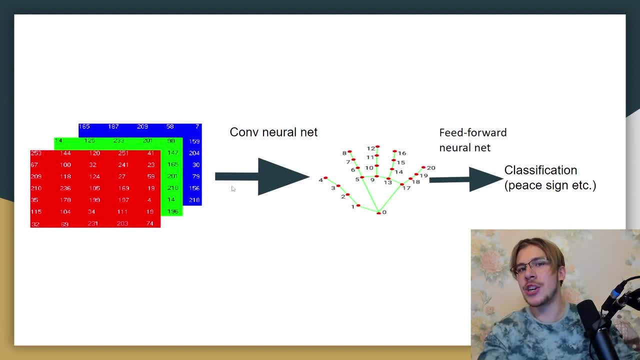 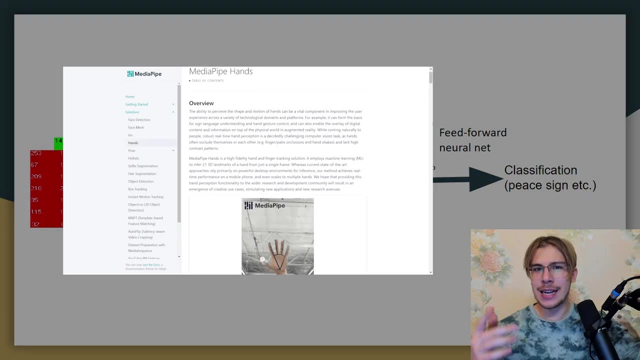 to, like you know, extract this embeddings is like much harder of a task, but, you know, we actually don't have to train it since, like it's a pretty well-known problem and there's, you know, they're- they're like pre-made, like ready neural nets that we can use for this task and that's where, like, 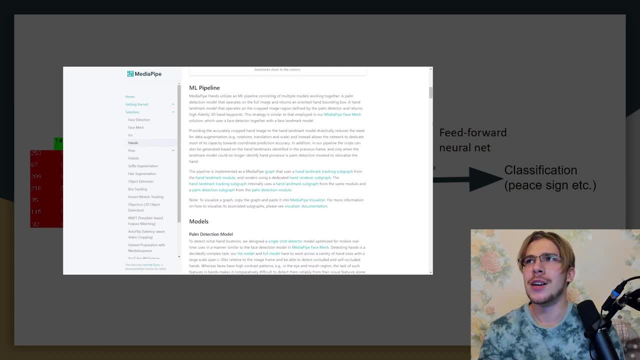 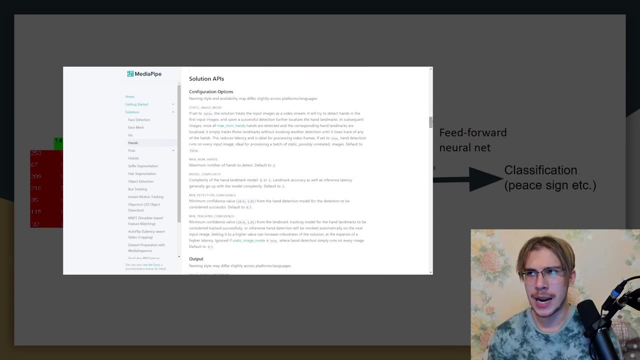 google's media pipe is going to come into play in just a few moments, uh, and so, like, if the whole, like we don't have to train it, we can use it for this task, and that's where, like we're going to train this thing is not a problem, right? um, then we can actually start looking at the like. 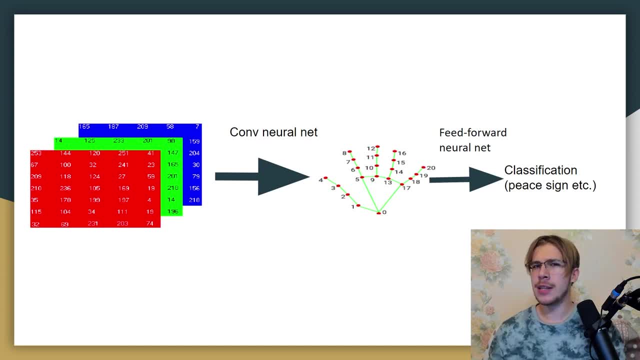 advantages of this approach, and the main advantage is that we have this like really cool, really reliable neural net that's capable of like extracting hand landmarks, um, like training a neural network on this, on like hand landmarks, to recognize gestures, is a vastly, vastly, vastly simpler task than training it on pixels, because, as i was saying, 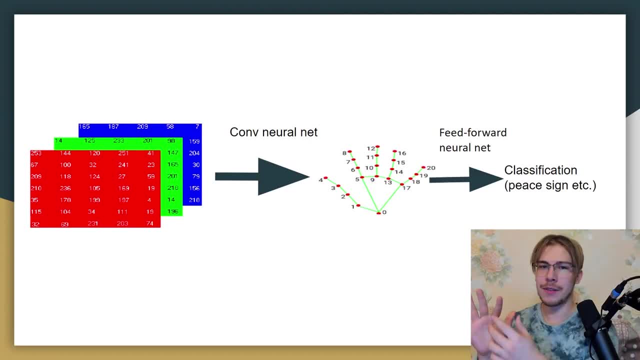 hands can be different shape, they can have different like finger lengths, they can have, like i don't know, different skin color, different um, i don't know. like just really really, they can be really really different and lighting can be different and the cameras can be very different. 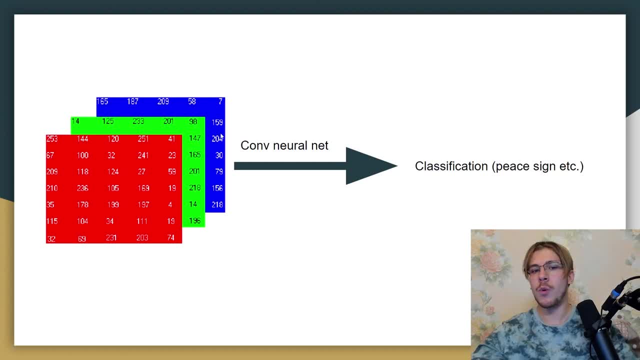 and so for us to train like this simple system, we need to collect a lot of training data, like we'd need, hands that are on this type of like fancy flowery background that i have, but also hands that are like on i don't know, like a blank, like white wall background or on the like brick. 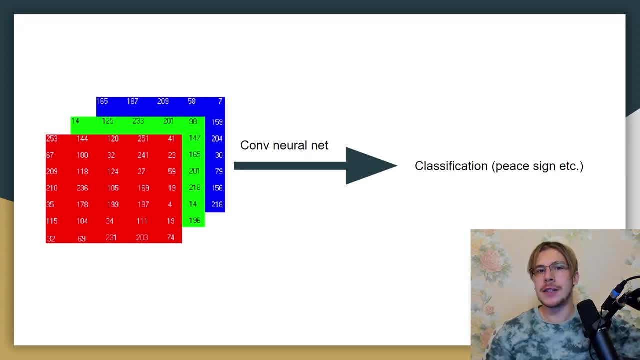 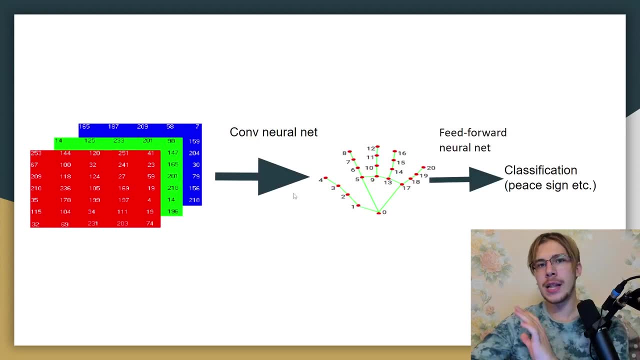 wall background or on, just like the countryside, forest background, if you want. if you want the system to be really, really reliable like that, right, but with hand landmarks kind of all, like heavy lifting ends up being done, but it's like uh kind of country neural net that's extracting the 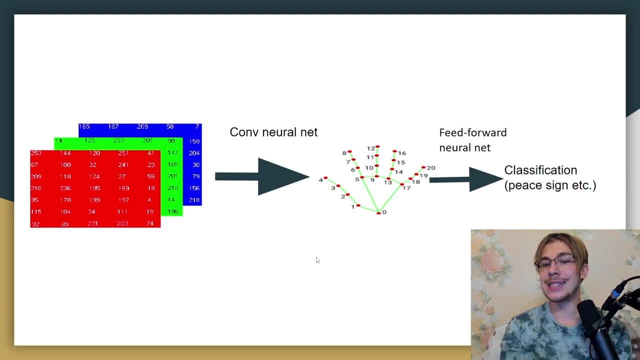 this like landmarks and once once it's extracted the landmarks, it's pretty much all the data that smaller neural network needs in order to do like a classification. so leverage this like really powerful pre-trained neural net that's extracting these embeddings um to be able to train a much. 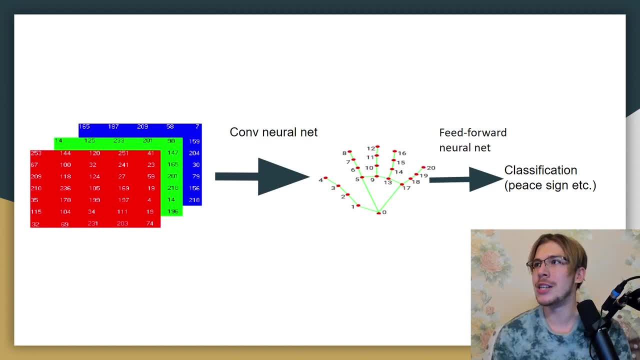 smaller neural network that's much lighter, much easier to train and that that requires a lot less training images. so, for instance, if you want to train it to recognize a peace sign, instead of me going and like collecting, you know, peace signs and all sorts of like different, you know. 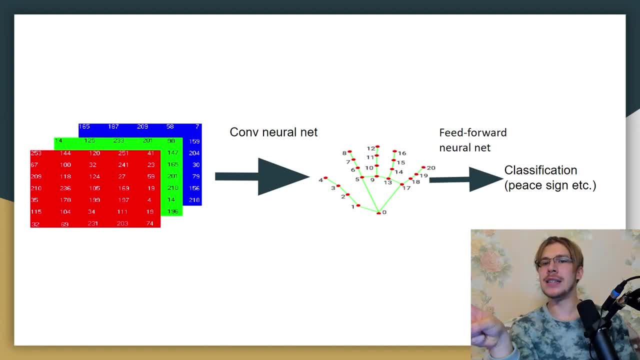 backgrounds. i can just show, like the peace signs, maybe in different, like couple different orientations and a couple different like i don't know uh, ways that you can show it or whatnot. like uh, and that'll be enough, and like that, that's the uh, that's like. 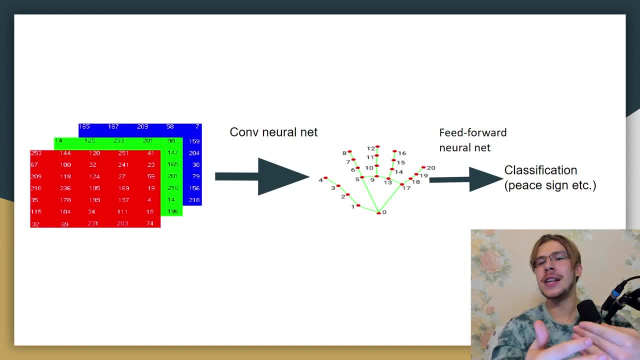 that's like the power of this approach that we're leveraging this like cool pre-trainer on that, to extract the, to extract the landmarks so that, so that that we can train a much smaller, much simpler neural network to perform the actual classification. so now that we've talked about this like landmarks, 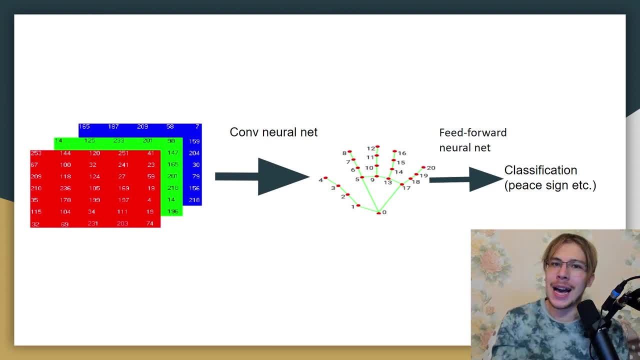 first approach, you can train a much smaller, much simpler neural network to perform the actual. you might notice that one step here is missing, um, and that step is that, like the neural network which extracting this hand landmarks and subsequently the neural net that's classifying the hand gestures, it doesn't really need to look at all of the frame like it doesn't really need. 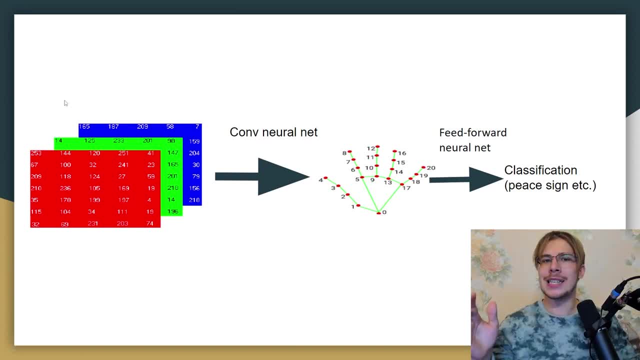 to look at every single pixel in the frame to recognize a hand gesture. as you may guess, it really only needs to look at the actual hand, which means that, like all the like background and all of the like, i don't know, like the other part of my hand or the other. 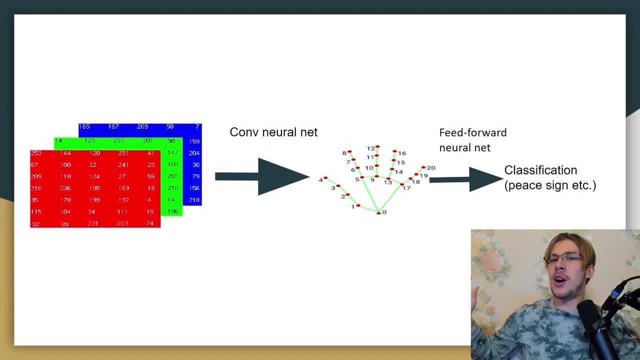 i don't know, like me, the background, all stuff like that is like it's not important. and so we can make the whole system a lot more reliable by first cropping the hand like the, the, the area in the image where all of the data that we need to make the prediction as to what hand gesture that, that. 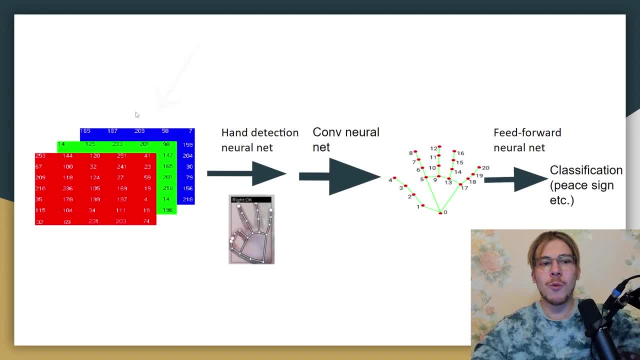 area is showing is contained, which looks something like this: we grab the frames from the camera, starts off the same. but then we pass those frames from the camera through a hand detection model which you know pretty much detects the hand image and like crops it. and then we take that. 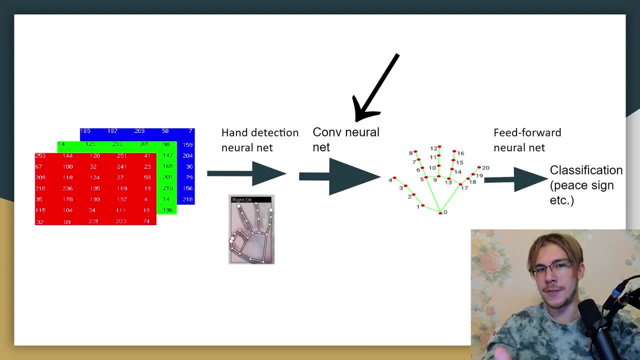 cropped hand image and we pass that through that like powerful control net that gives us the hand landmarks, and then those hand landmarks we pass through a feed forward neural network that performs the classification. so that's actually like i would say, you know, if not the most effective. 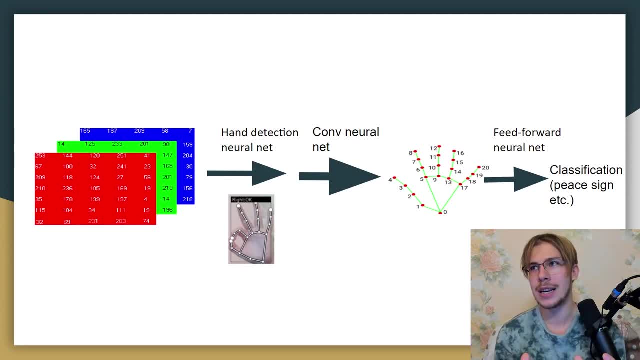 then, like in the context of what we're talking about, like it's definitely the most like effective, efficient way of recognizing hand gestures on a single hand. now, looking at this approach, it might look a little bit complicated and as if it would be difficult to implement, but like i actually kind of assured 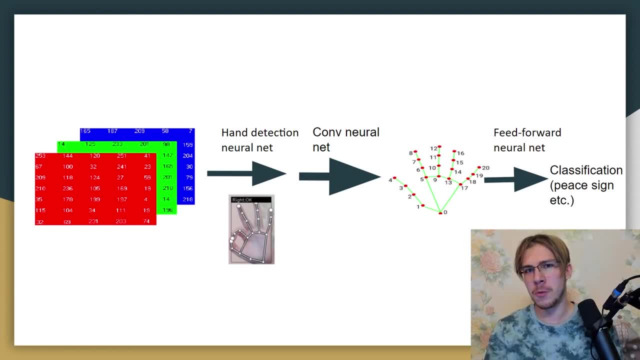 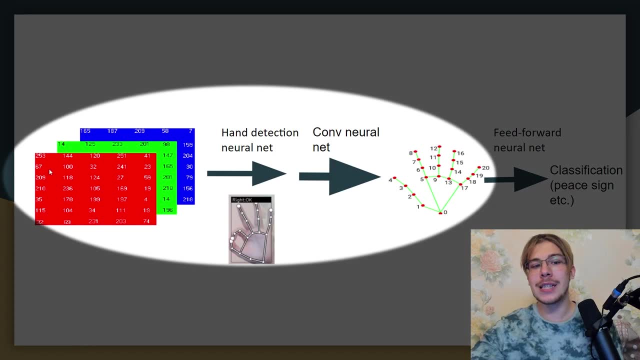 you that it's going to be really easy to implement for one main reason, and that is that a lot of the work has been done for us. so, for example, this stage with hand detection and landmark extraction is is like handled really well by google's media pipe framework, and so, as i'll show you like a cup in a couple moments, we pretty much 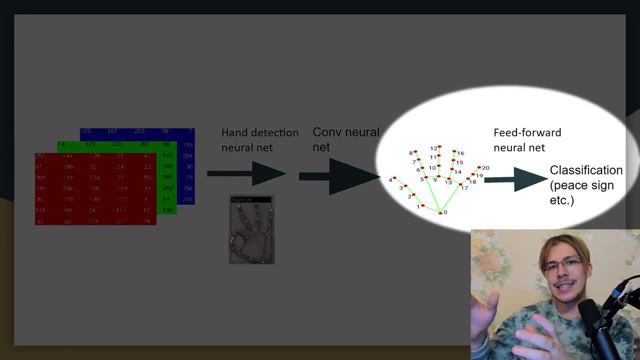 just like run some python code and it's detecting the landmarks. and that second stage, which has to do with the training of like a smaller feed forward neural network and the collecting training images, and all that stuff is handled really well by the repo which i'll show you in also a couple moments. 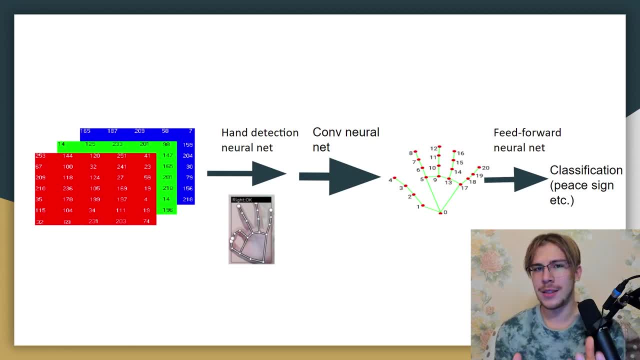 so so that's like the top level overview of how things work here, and so right now we're on the web page and we're going to be talking about how to implement this, and we're going to be talking about how to implement this and we're going to be talking about how to implement this. 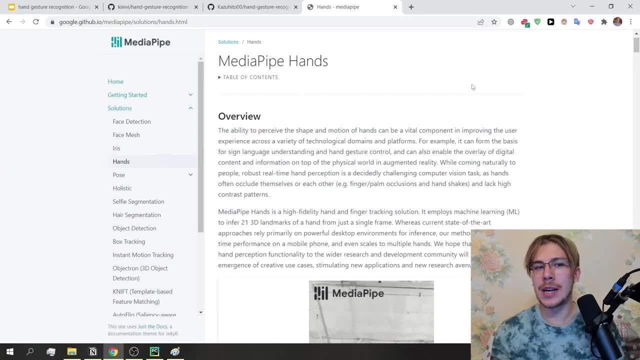 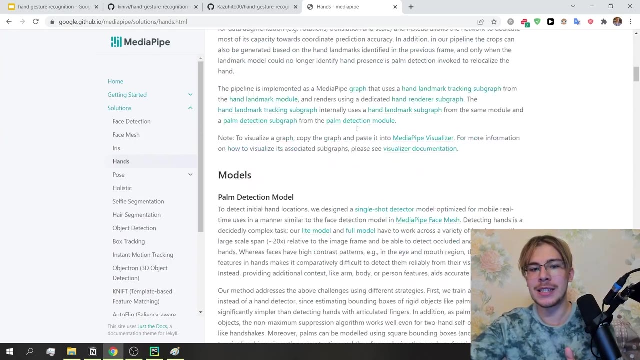 online with the word protection collaboration, but we're right now on this, like on that page, where it kind of explains what's it doing and here we can see, like the models that are used, is the palm detection model, as we've talked about here. that detects the increases, the profesionalness of my video. 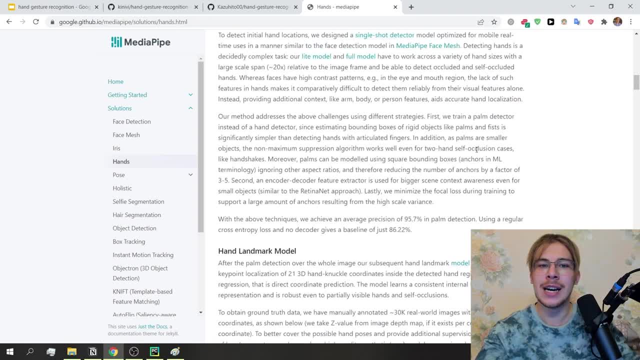 and the next model is the hand landmark detection model, which takes the um, crap palms, that cropped palms entity right here and it's built seriously. that makes it so. it's just a pretty little different neighborhood, so looking a little bit faster with them the camera and, uh, developing a lot of Cooler In today's videos, which means we're going to put some technical 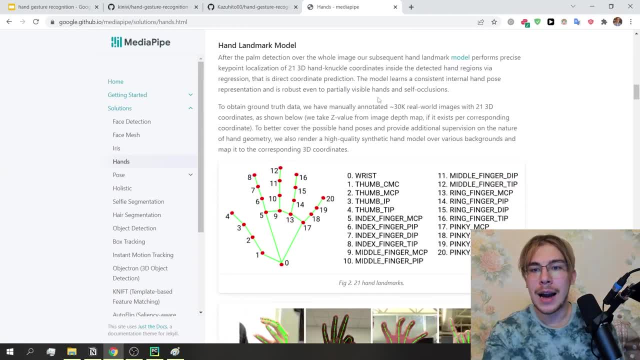 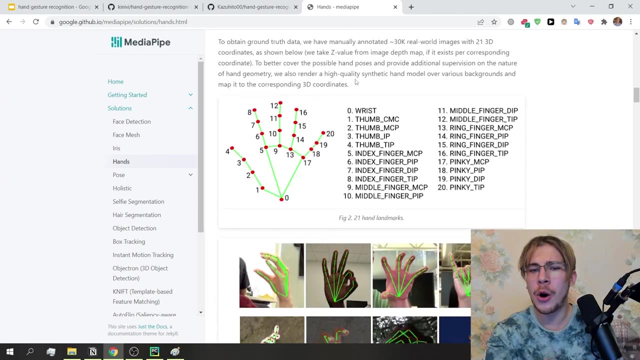 hand images and uh and performs precise keypoint localization of 21 3d hand knuckle coordinates inside the detected hand regions via regression. regression, that is direct coordinate prediction. so all that is said, that it, you know, classifies the uh landmarks and here they provide offensive. 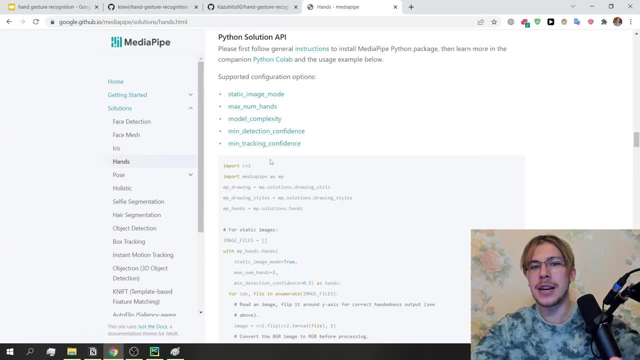 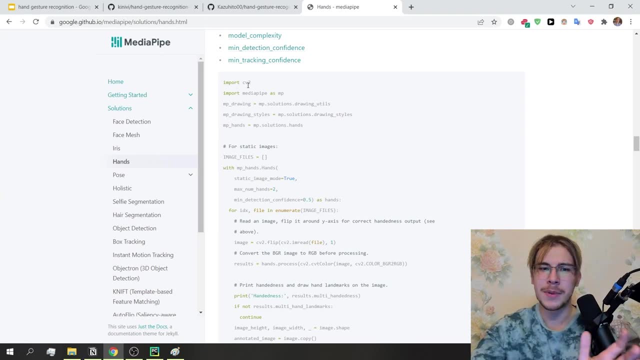 way to say that um, and here they provide like the python api for us to try it out. so all you need to run this thing is to have opencv installed, which is like really easy to do like just like through pip and stuff, and then install media pipe. it'll probably run like some tensorflow light and all. 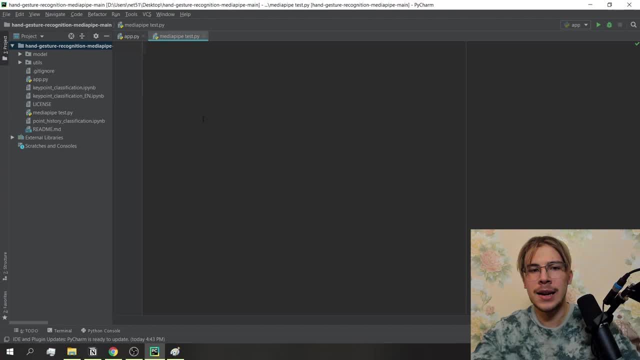 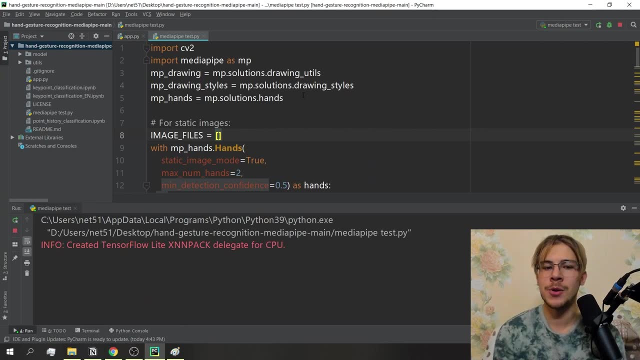 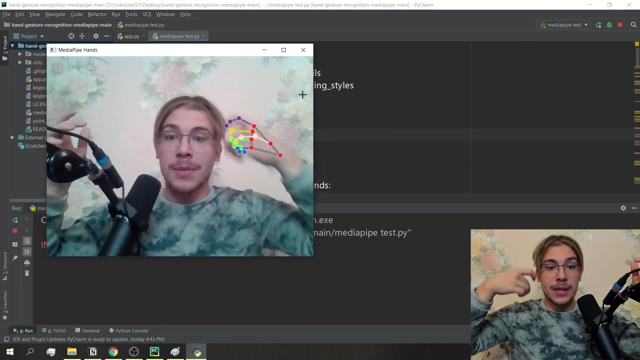 that's in the background but all of the running is done on on the, on the cpu and uh, it's like it runs pretty quickly. in my case, like i'll show you in a moment, i have like two webcams like this. this one it's it's the uh, uh, my kind of laptops like inbuilt webcam right here and as you can. 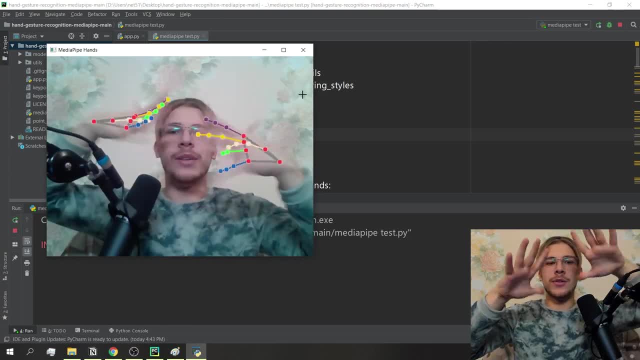 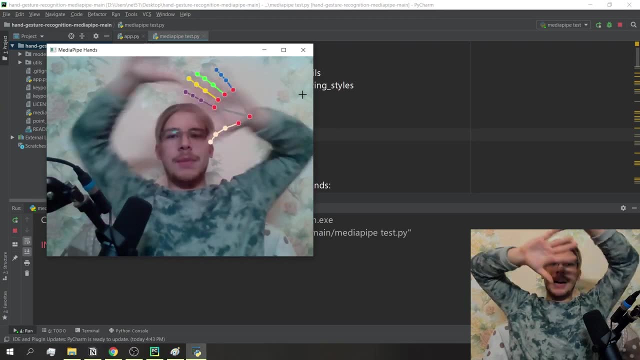 see like i run it and it's running like pretty fast all that on cpu and it's detecting the hand landmarks and it's. it's pretty cool how well it works right. like you know, my hands can be like all sorts of different like orientations i can like. they can even like obscure each other to a. 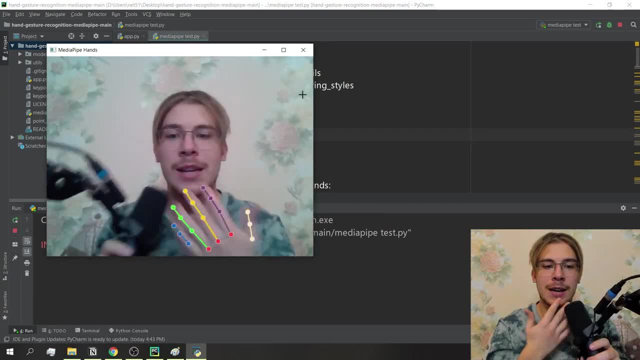 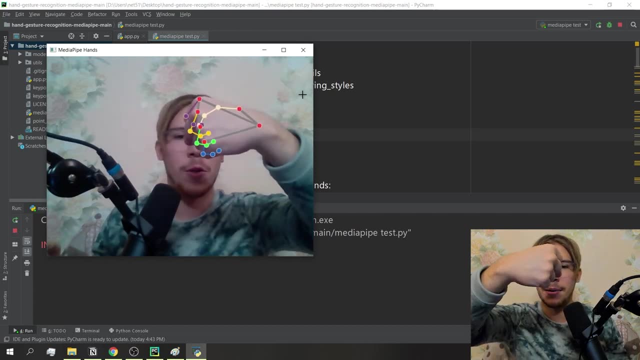 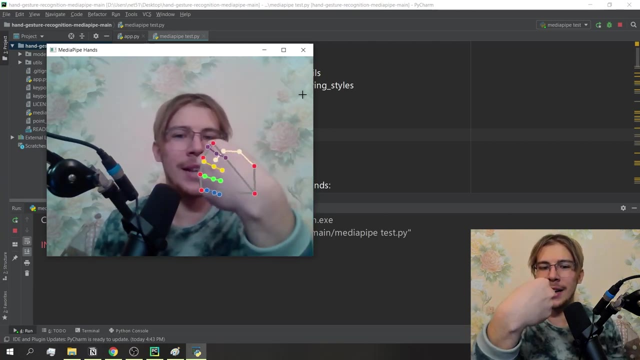 certain extent, you know it'll still be um, it'll still be working. uh, i can kind of- yeah, i can kind of like even hide my hand behind the mic and i'll still able to get the call picture and like for like um, you know, if your gestures are like operating, like on some sort of like close, 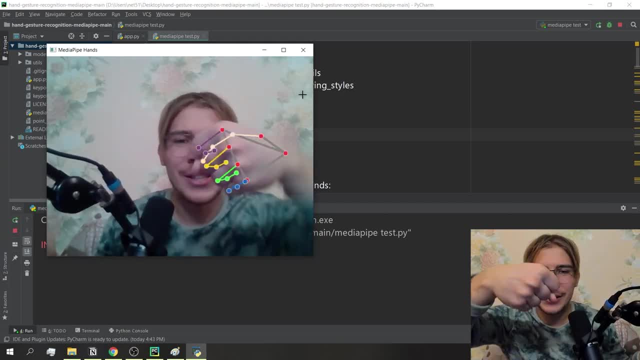 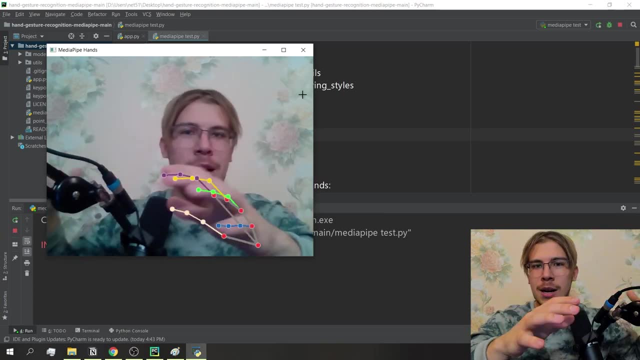 closed palm away, like. as you can see, it's also handling like that that quite well as well. um, so, so like that's pretty much like the simplest way that we can work with google as media pipe framework and kind of get it, get it to show us some, some results if it's giving you, like any. 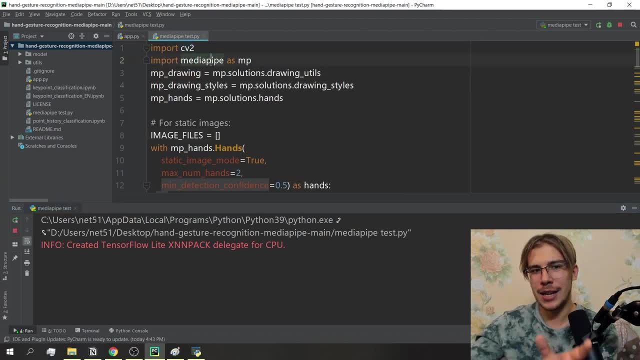 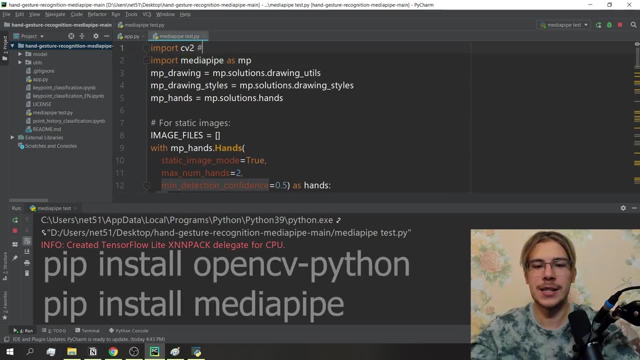 errors here, like media pipes not installed or like cv2 not installed, just like go and install. people install like open cv and media pipe, like that pretty easy to do, honestly. uh, for open cv, it's like pip install in the python console. uh, people install open cv. dash python for media pipe, just people install media pipe. um, yeah, just in case. 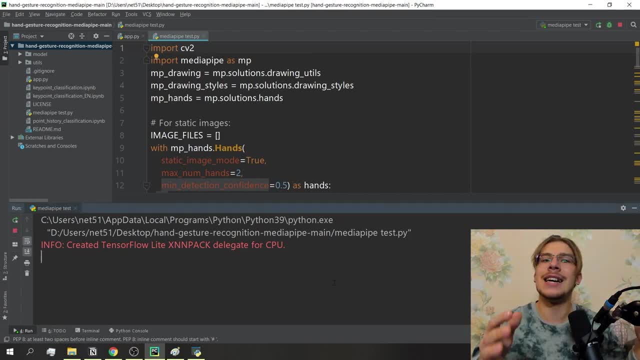 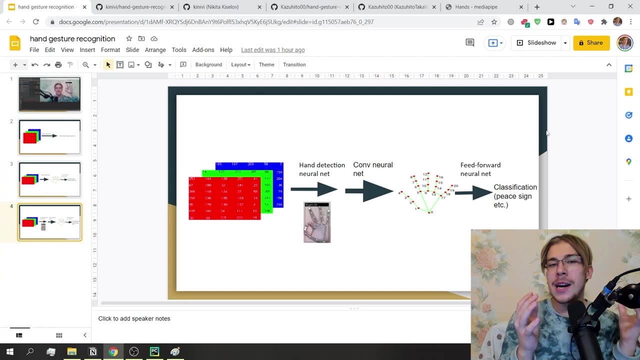 any of you have any problems here. so that's us testing, kind of like the basic um media pipe hand landmark detection application right here. so now that we have looked at the media pipe, part of the pipeline of our hand gesture recognition system and pretty much covered like the extraction of frames, palm detection and 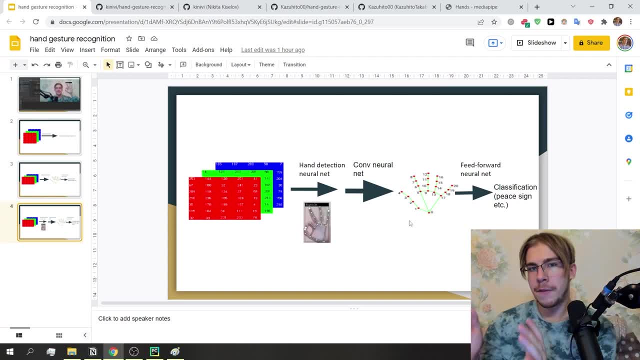 hand landmark detections using video pipe. uh, we'll fill in the remaining, um, pretty much the remaining kind of steps that are required to recognize custom hand gestures, which is like collection of of data and then training, like a smaller neural net, to perform that task using a really, really cool repo, and let's, let's take a look at it. so it's this repo that's that's called. 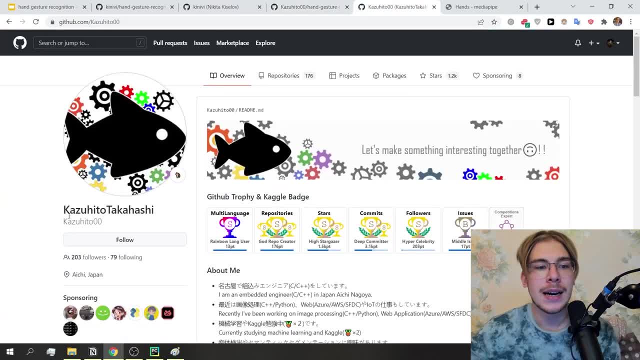 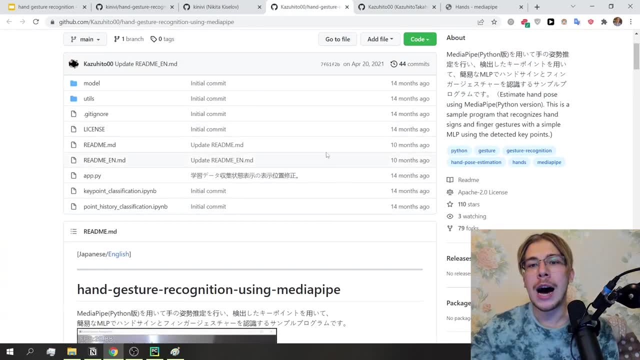 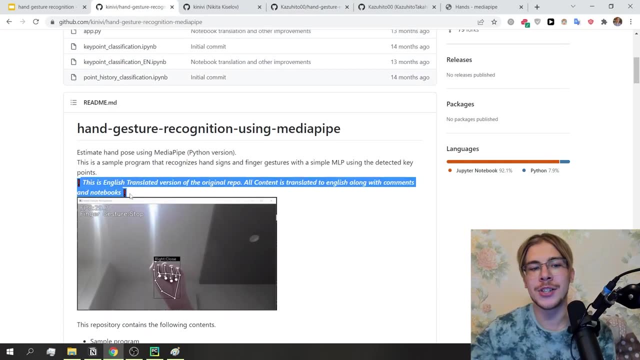 hand gesture recognition using media pipe: um by um kazuhiro uh, takashi um. so it's a, it's a really awesome repo, uh, and the one we're going to be using is not this one, though it's um, this one, which is just a english translation of, you know, of the like of the original repo. so so it's like. 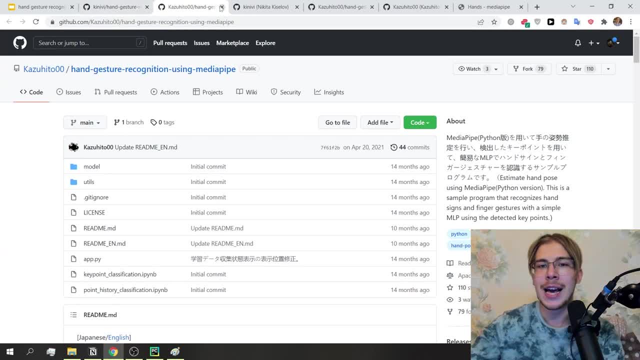 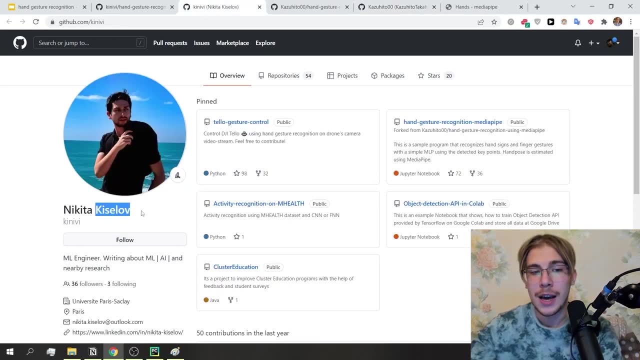 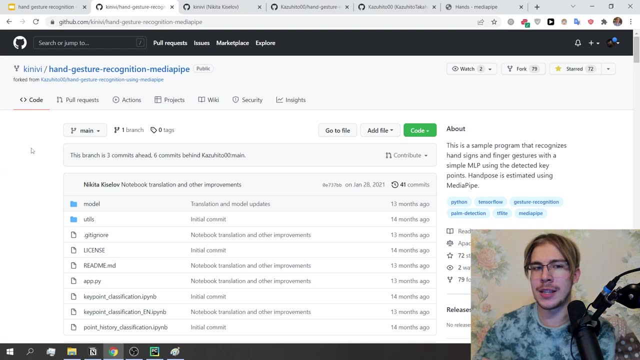 a fork of that original repo translated into english, and so the original repo is by kazuhiro and the translation is by nikita keselov. uh, right, here is the author of like this translated repo. so now, in order to get this repo, you can either git, clone it, um using this url, or just go here. 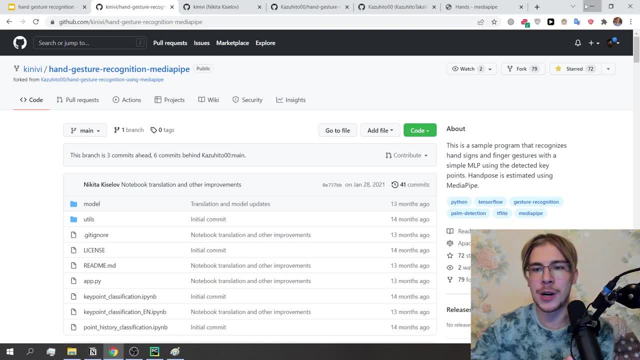 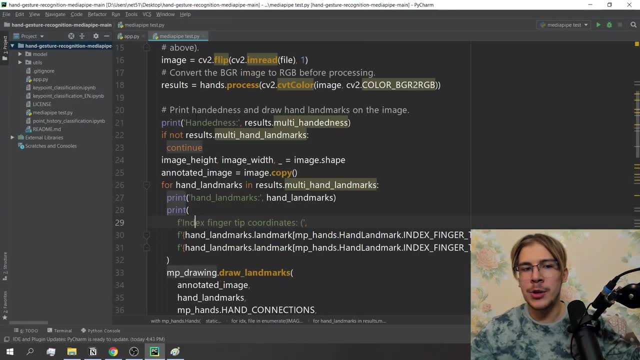 and download the zip file and just extract it somewhere. i've put it on my desktop right here and i have it opened in an id called pycharm, which is just essentially like an- uh, like a place where you can like write python in a nice way, but you can use like any id that. 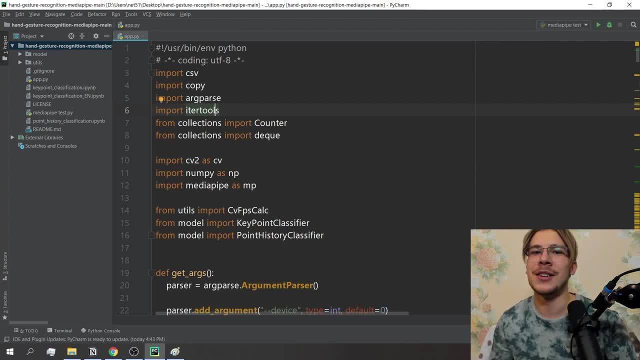 i'm keeping it like beginner friendly, but, like you know it, obviously you can use uh the whatever way that you like to write python. i prefer pycharm for these types of things. um, so now that we've git clone this repo, it actually shouldn't have this file because we just created that. i've just 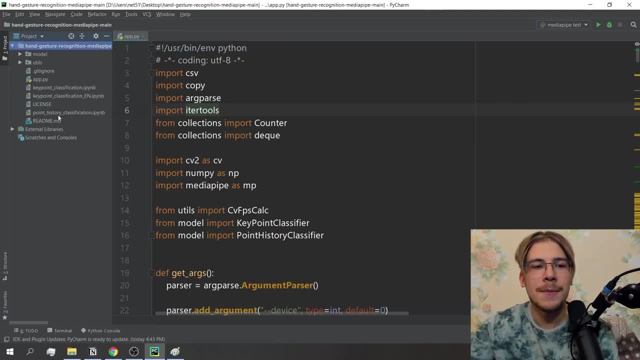 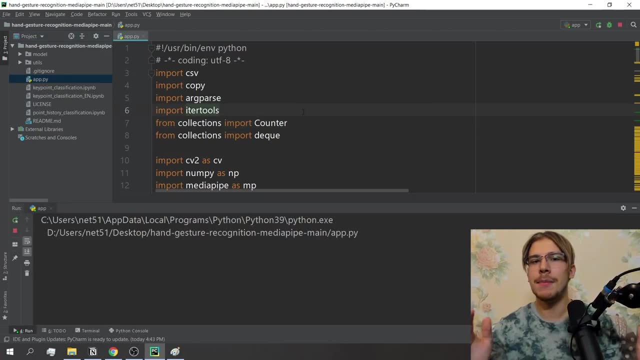 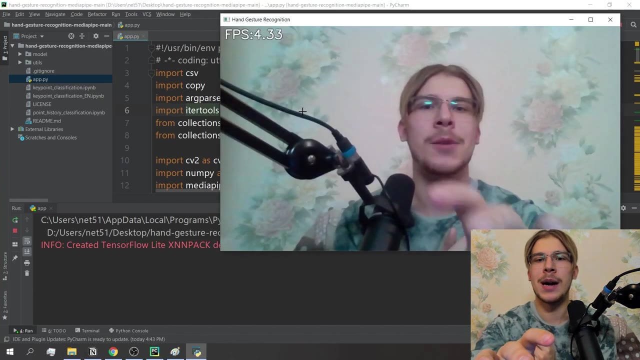 created that a couple of seconds ago, faced media pipe, um. so now we can go ahead and launch the update 5 file, which pretty much launches the, which is pretty much like the main file in this, performs inference in the frames from our webcam and processes them in a way where it detects hand. 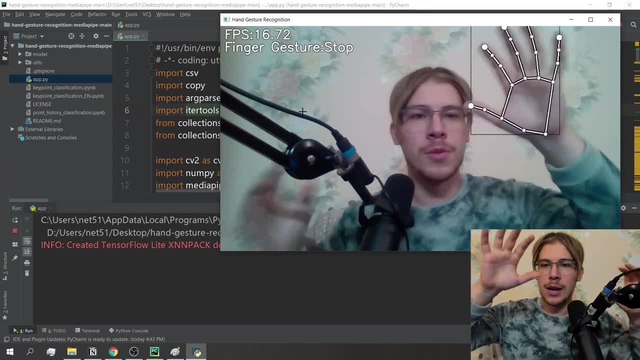 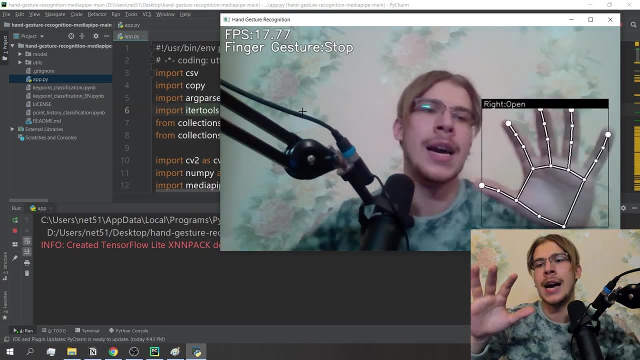 gestures. so now we can see that right out of the bag. it's able to attack the single hand. i'll show you how to like, enable, like multi-hand detection, in a few minutes probably. but it's able to detect the single hand and it has that, like hand gesture recognition, built in. in this case it recognizes. 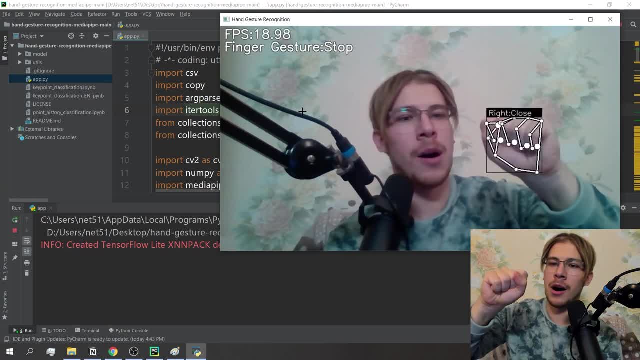 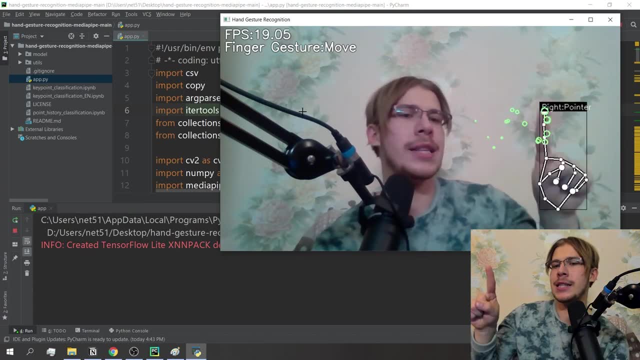 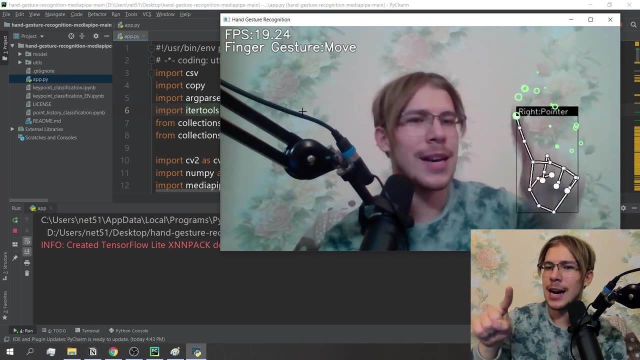 the open open palm like closed palm and uh okay sign and the pointer um. so there's also a part in this repo that deals with, um, like, recognition of, like this point history, you know drawings- uh, that's not what this video is focused on, but like, feel free to explore. 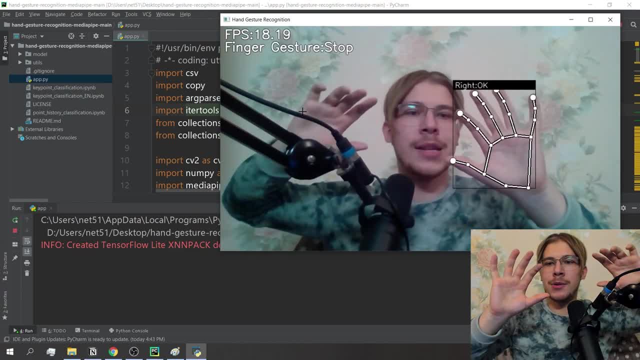 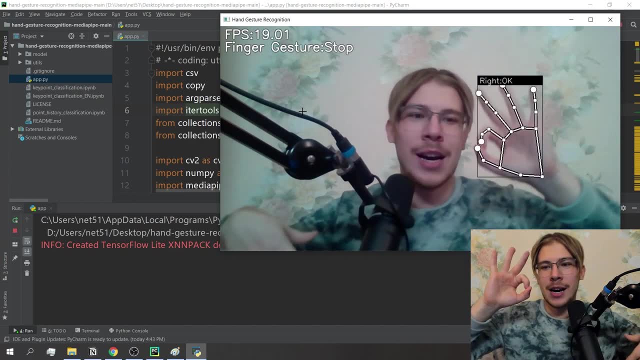 it. also we're focused on this primarily cool part where we, um, you know, recognizing like hand gestures, like this is closed hand gesture and this is like open hand gesture, okay hand gesture- and how we can like add some of some, some of the like custom hand gestures. so 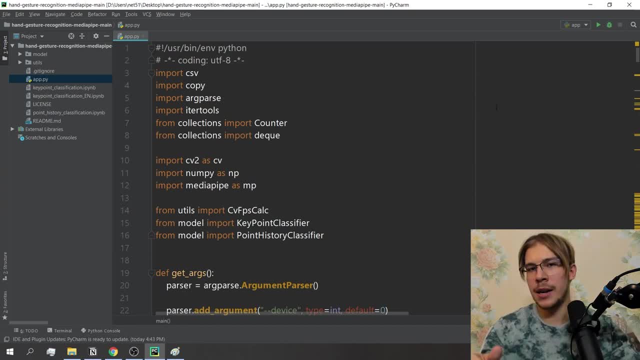 yeah. so now let's start looking at the code and maybe like tweaking a few things here and there. so the first thing is we've noticed is that it's only working right now on detecting like hand gestures in one hand. you may want to use it to detect hand gestures, maybe on two hands or on. 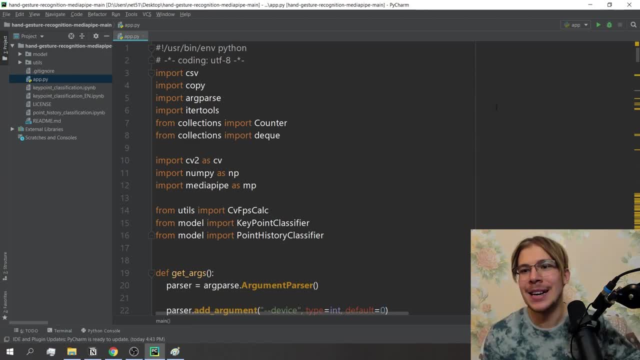 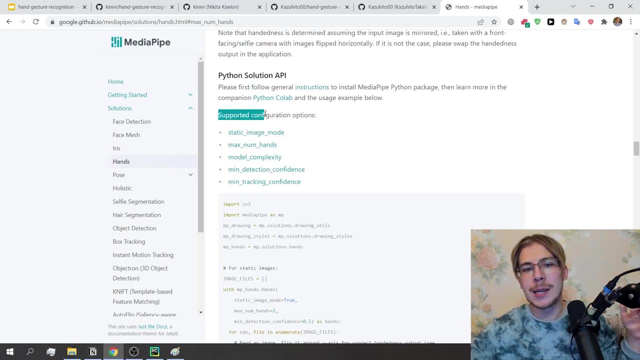 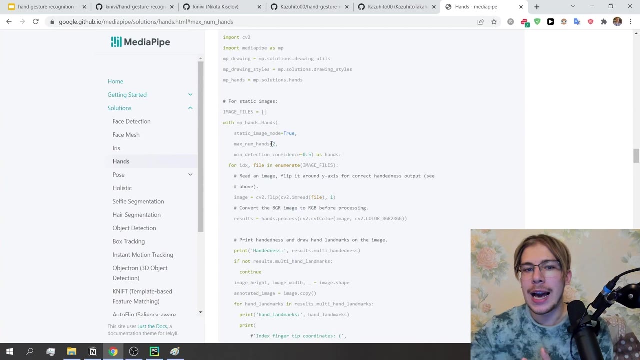 three hands, or i don't know how many hands you want to put into work here. but so now, if you look at the media pipe docs right here, we can see that there are several uh supported configurations options, and one of them is maxnet hands, which is defined in the python code here, and so in our case, if we find it in our code by 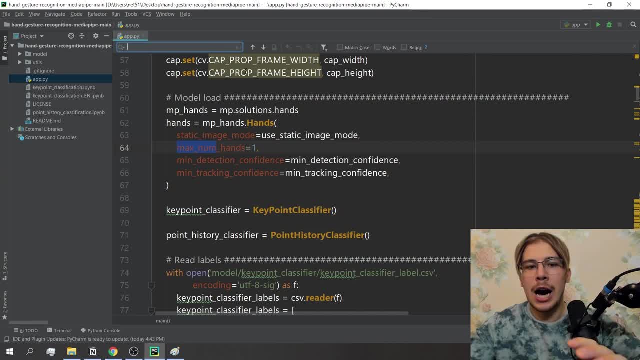 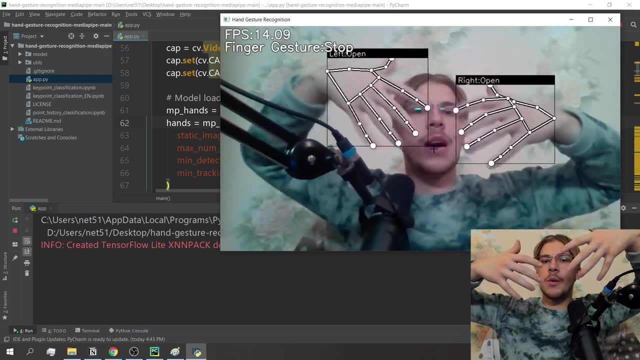 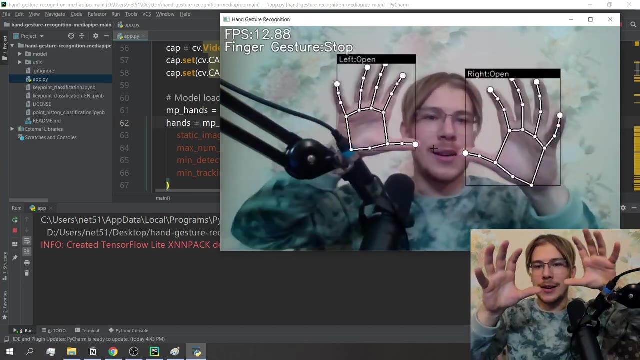 searching maxnam hands. it's set to one, uh, we can set it to two and it will be able to detect um, two hands, pretty much, yep. so now, if we look at, you know, at the screen right here, at the like this, like open cbo window, uh, which is like handling, like all of the like, displaying all 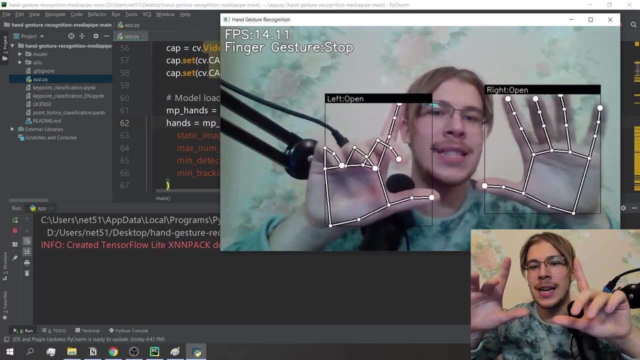 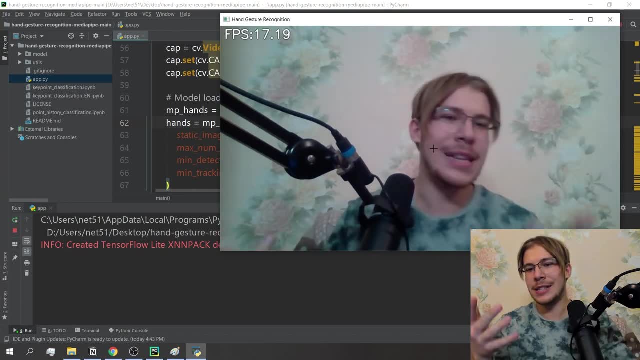 the drawings. i was saying you can see that, like the detection is happening on two hands. here's something interesting that i didn't notice, like at first, but then i was like there's got to be more to it, right, if it's doing that. so, as you can see, it's detecting. 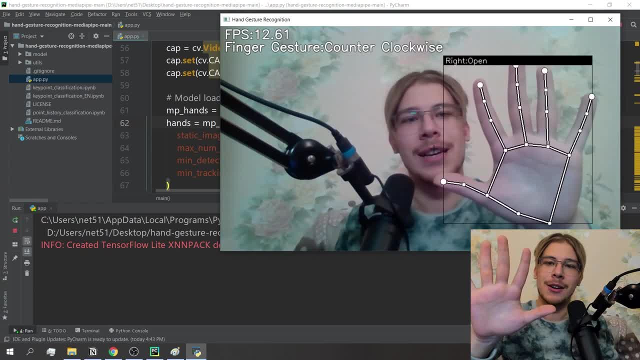 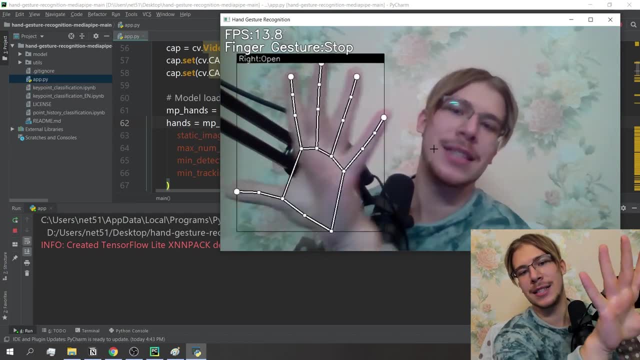 uh, like you know, for instance, here i have my right hand right, so if i flip it around, it's still the right hand. if i put it like on the other side of the screen, it's still the right hand. and if i flip it around like this, it's still the right hand. so um, same thing with the left hand. so it's like you. 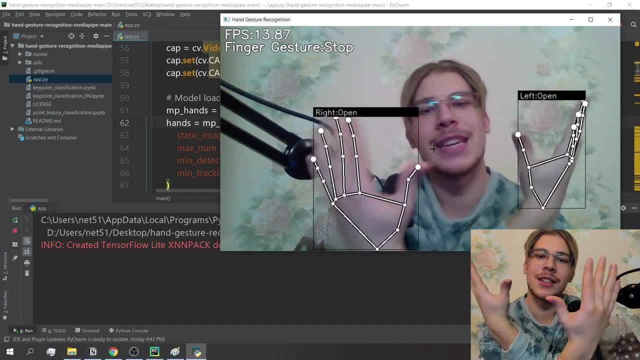 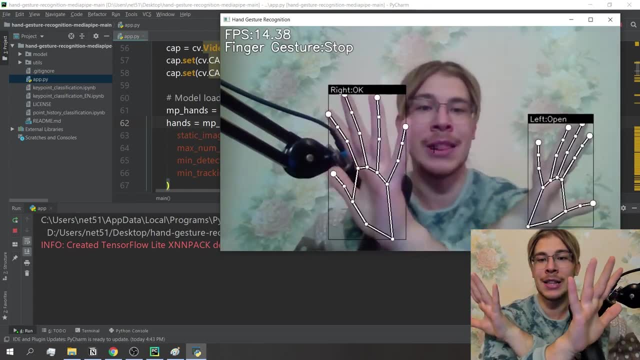 can't really fool it like, however, i want to like rearrange my hands- you don't know that- like this which it is, and this one's like the left hand, even if they're like completely swapped on the like, complete, like opposite sides of the of the like of the screen, pretty much so that tells us that. 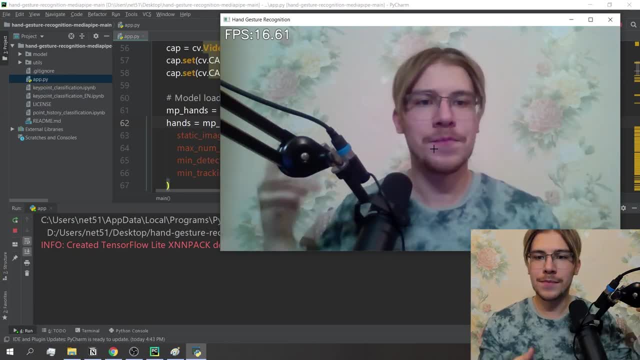 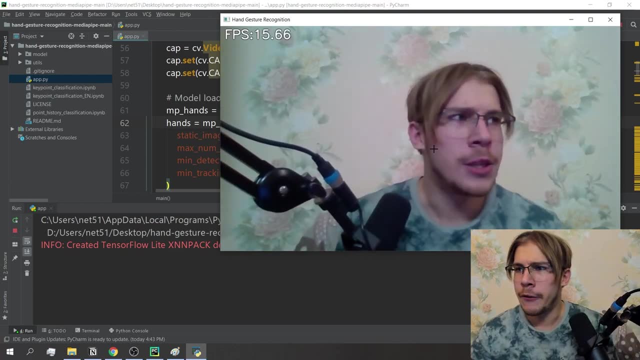 media pipe also has like an inbuilt way to detect the handedness of a handle, like whether it's the right hand, whether that's left hand. uh, one can not be useful. so, for instance, in the like example of like uh, the former student of mine that i was talking about in the beginning of the video, 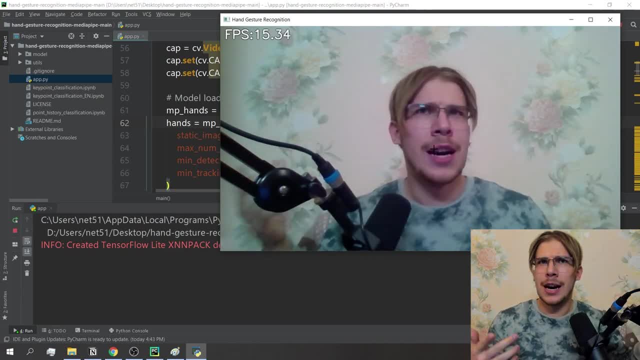 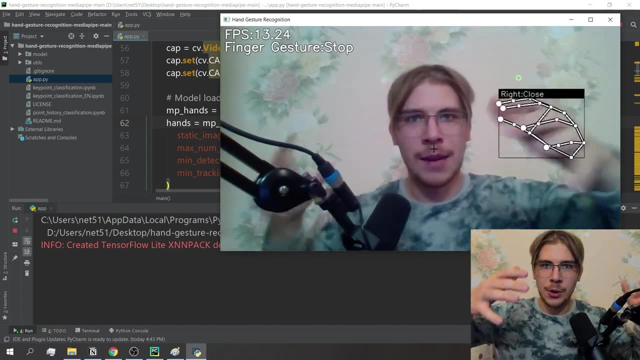 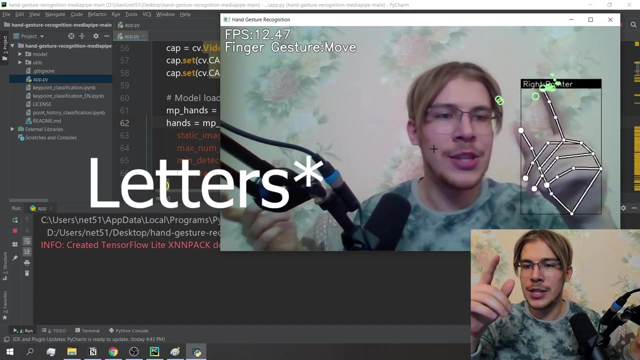 where she was training, like a system to record nice russian, uh, sign language letters that you can do like with one hand. she used, like this feature of media pipe which allows for, like multi, for the handedness detection to essentially, um, have always one hand be the one. that's like inputting the, the digits right, to be like that's doing something. 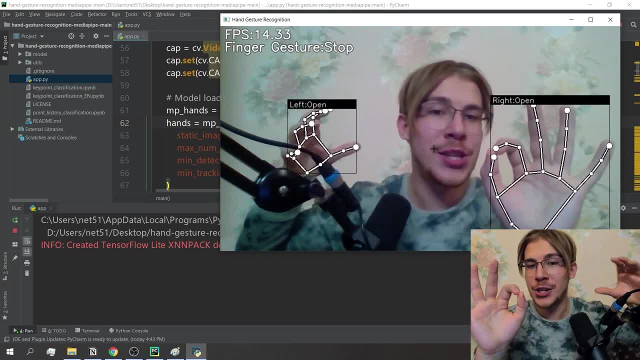 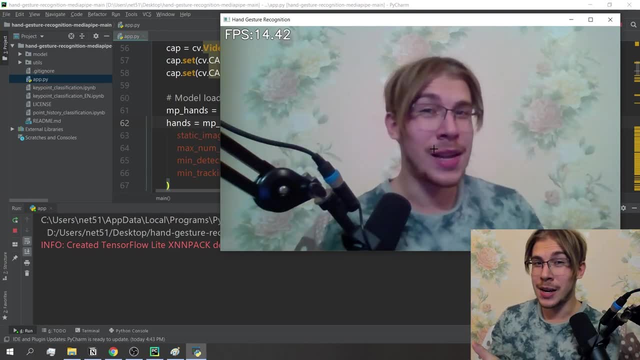 that's like from which we can read the gestures, and the other hand be the hand that's like controlling the inputting and the typing and all the other things, so like you can use this functionality to like separate. maybe from this hand you're detecting the gestures, from this hand you're detecting like different. 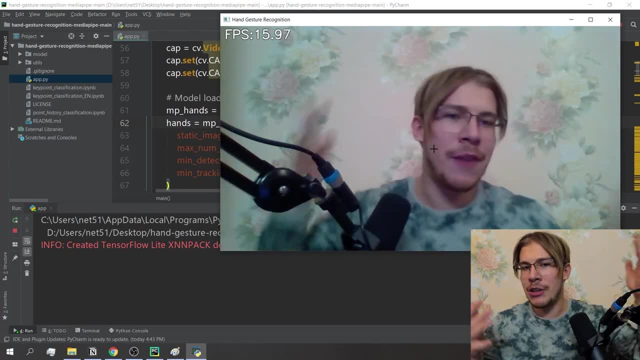 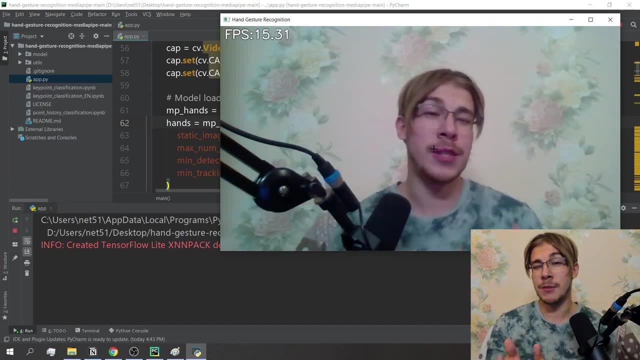 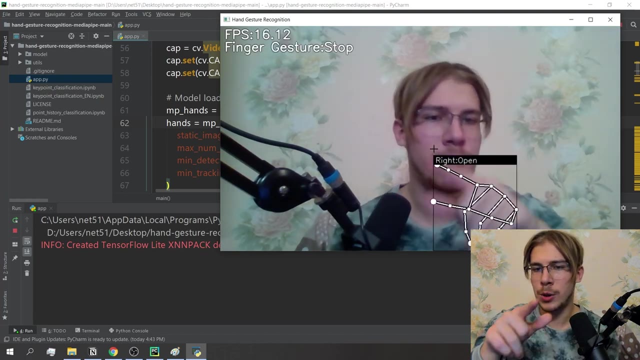 gestures and that's performing different actions in whatever the application that you can that you're working on. one thing to notice here: you can see that, like whenever i put like, so, for instance, right now, it's running at like 6, 17, 18, 16 fps, something like that, and that's because what's 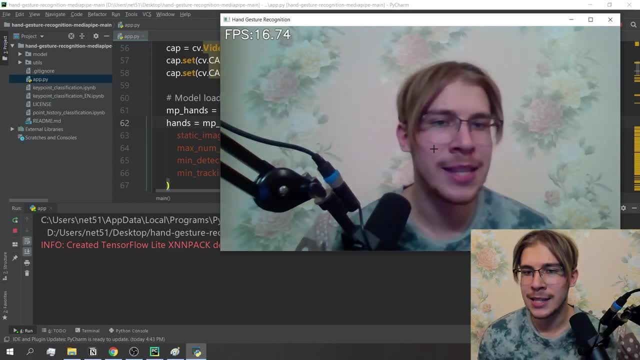 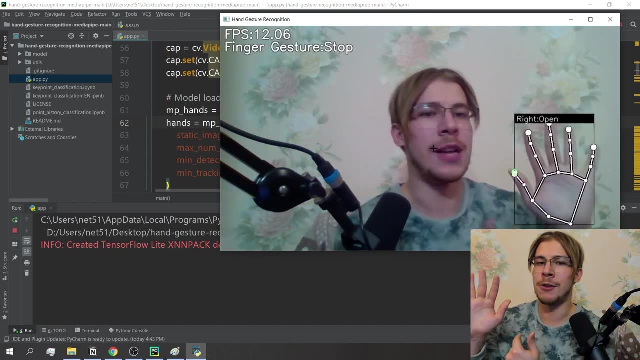 what happens right now, when there are, like, none of my hands detected, is that like all it's doing is that it's running the palm detection, the hand detection model that like detects palms and like grabs them and stuff on the frames. uh, but if i put in the hand, 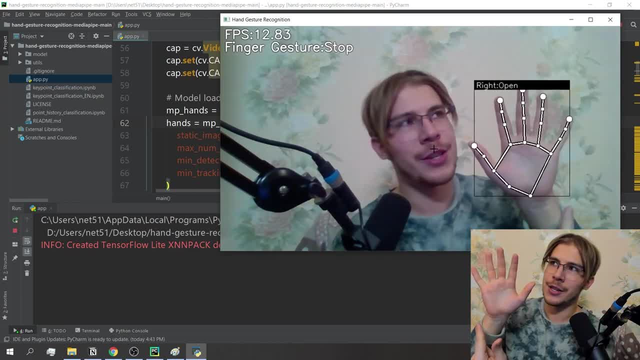 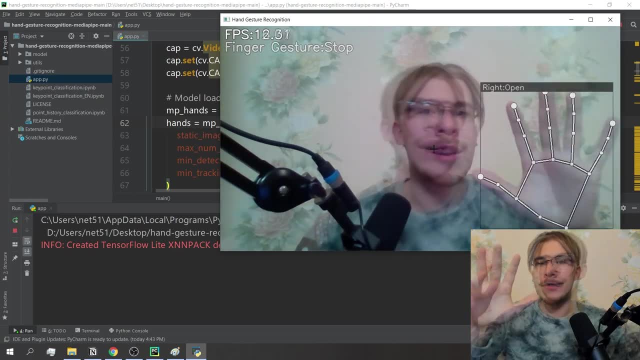 it starts to also run the like hand gesture recognition models in the landmark detection. that's like taking more of the processing power and as the frames per per second slow down, if i and like if i had another hand, and thus there's like a little bit more processing happening. 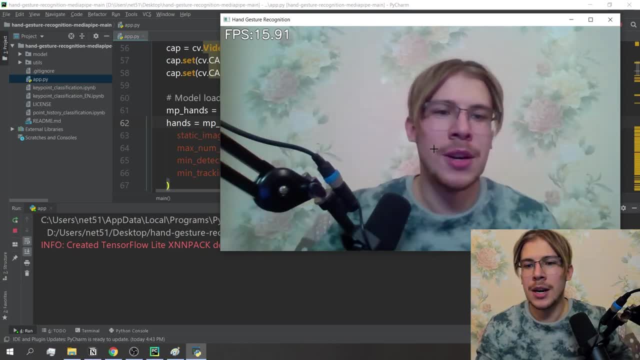 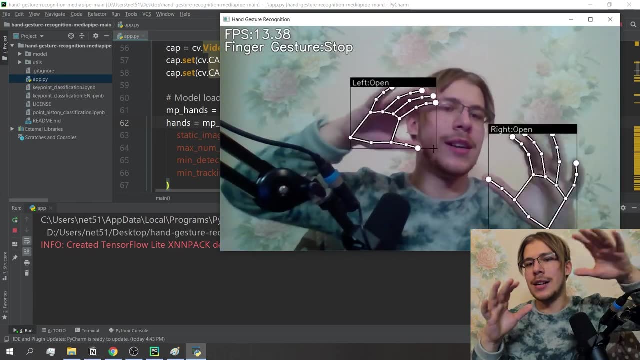 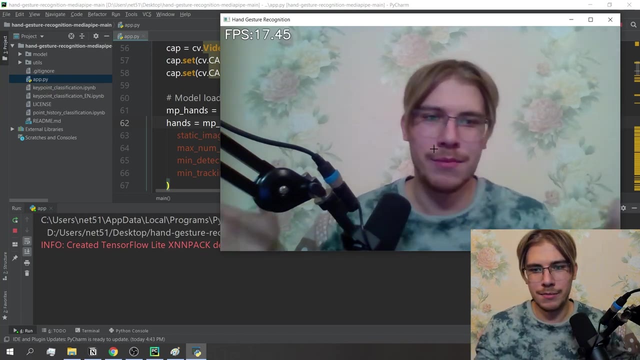 um also on on that on that front. so, uh, pretty much the only limitation for like running it on like a hand is is that, like you know, it might slow down the application. but, as you can see, it's like pretty remarkable um running on cpu running pretty fast, kind of doing what it pretty much needs to be. 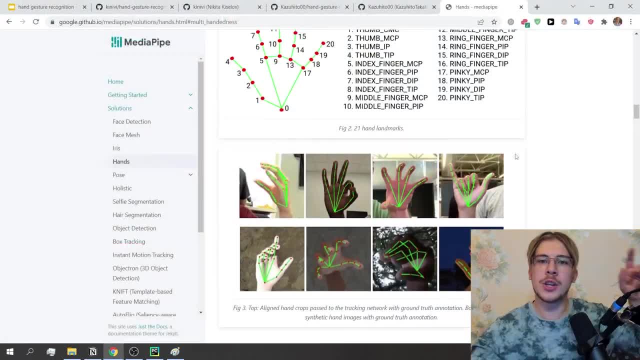 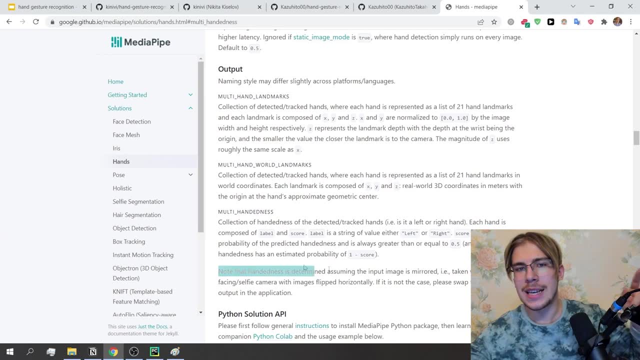 doing. um, yeah, and so here in the docs, in the like output section, it also talks about multi-handedness. um, i think that one note here is that is that, like, when determining the handedness of a hand, it's assuming that it's taken with like a uh front facing or like selfie camera, as it says here. um, 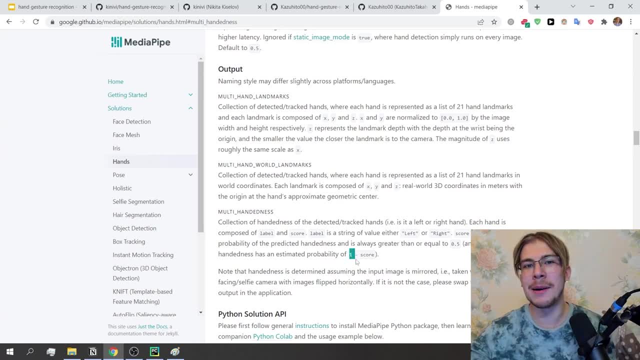 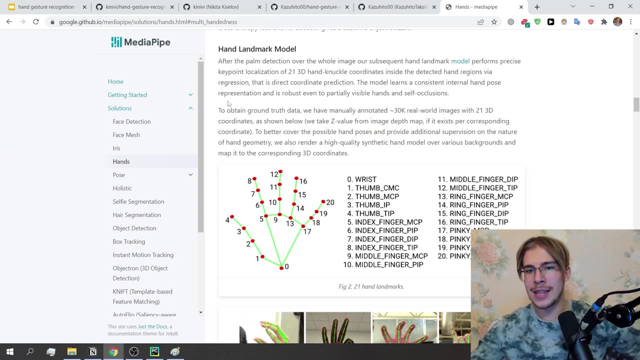 and if it's not the case, then you can like swap the handedness in the application. just something that i wanted to note here and, by the way, here in the docs they also said like how the hand landmark detection model was trained, and they say that it was like trained on, like manually annotated, like 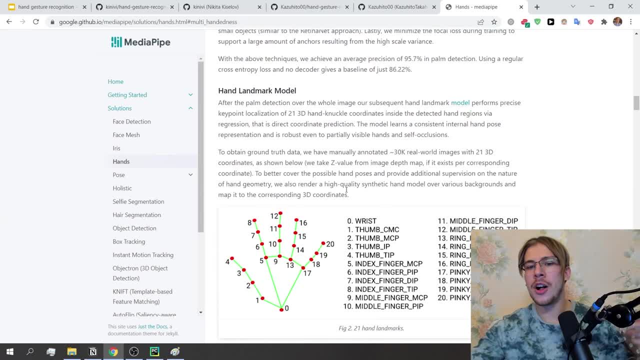 these types of images of people's hands and also on some of the like high quality synthetic hand models over various backgrounds, which also was fed into, like the training data. so now let me actually start giving you kind of like a walk through over like the main points. 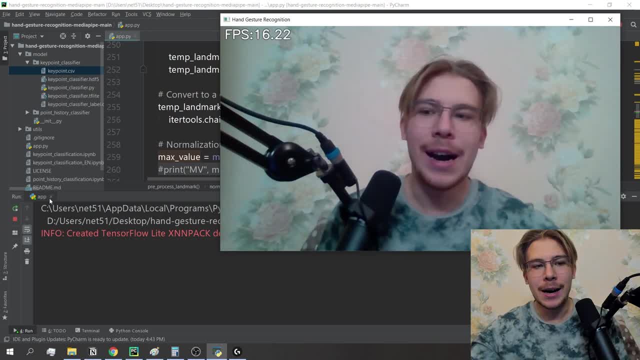 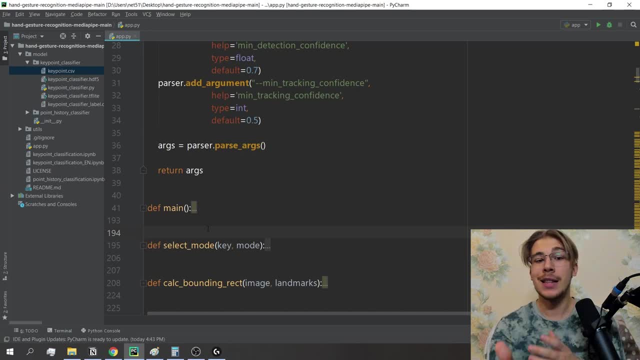 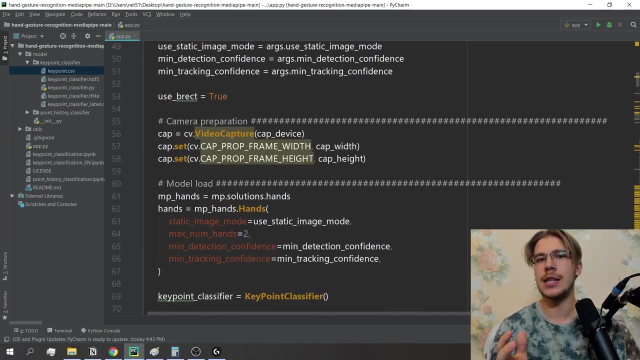 in the code, so that you'll have that understanding. um so, first of all, so the main kind of action in terms of, like, performing this type of inference and the frames from the camera, is happening inside the main function, and here again we'll first we'll focus, like, on the kind of opencv structures that 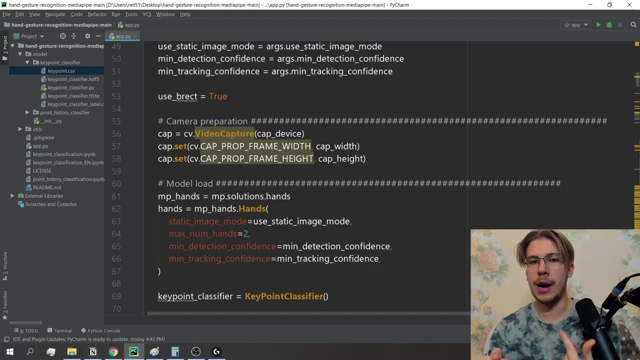 fit in the frames and uh, then there's three processing that that's performed on those frames. but uh, pretty much to anybody who's working on that kind of like opencv structures it's gonna be quite familiar. and if you haven't worked, you're gonna have like a series of cool. 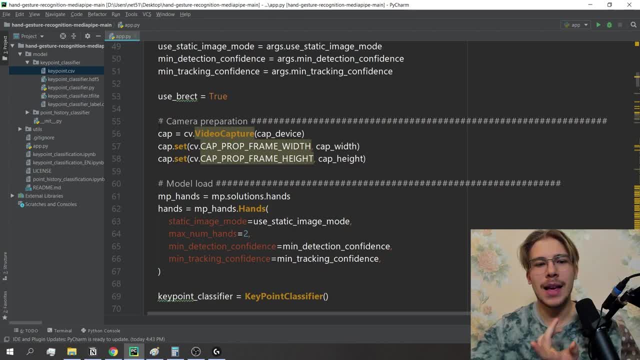 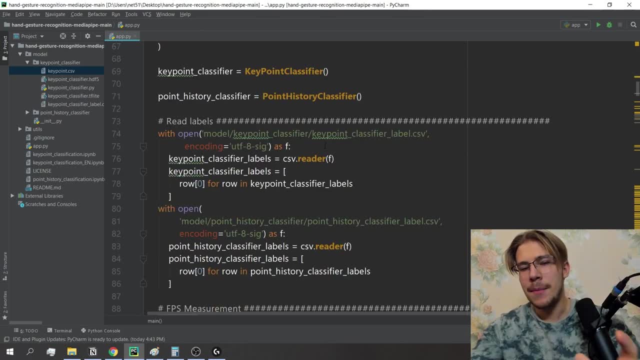 videos about it, if you're interested. um, the so we're defining the camera capture and stuff like that, which is like essentially the webcam that we'll be using for from which webcam to like grab the frames into the python code, stuff like that. um, then, then, then, and then this structure with the. 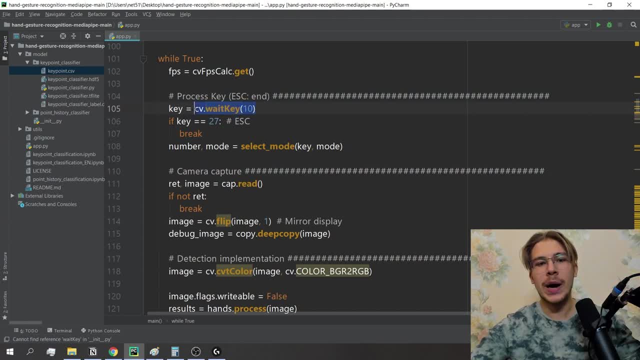 what am i doing? this structure- yeah, the structure with the while loop and the weight key inside of it, is something that's probably, like everybody who's worked with opencv will recognize- essentially way of creating this like while loop because, like, we're grabbing frames from the camera constantly, so it's like a while cycle where we're, you know, grabbing, grabbing and grabbing. 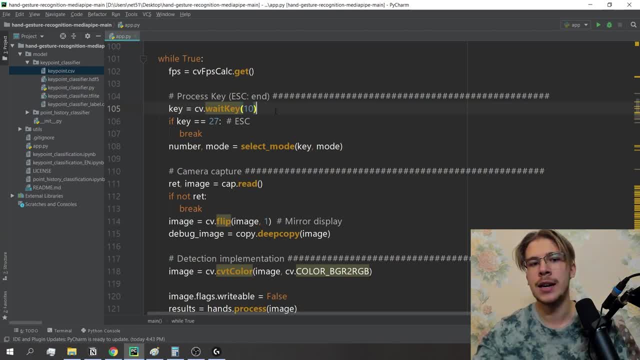 but for this type of loop to like work with opencv, there's got to be like a uh weight key command present there, uh, because like it has to wait for it to also input something into the window. i can kind of show like if we remove this line here, uh first like it'll crash um. 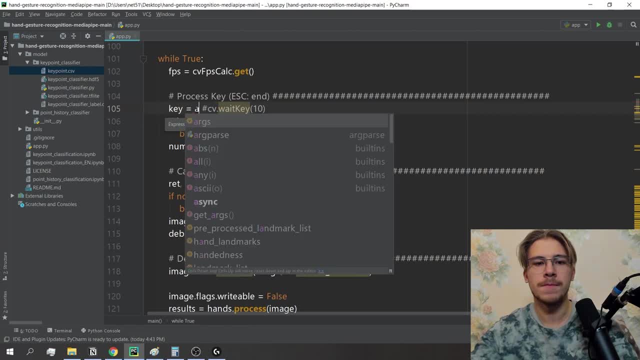 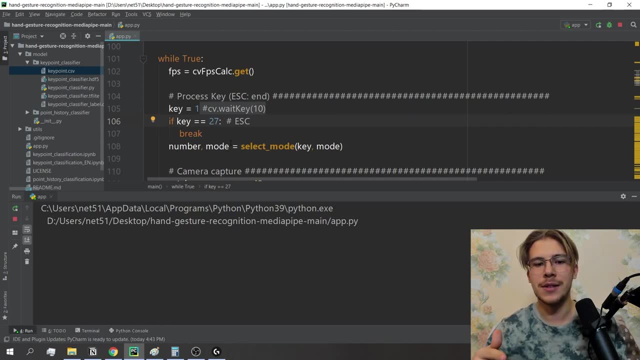 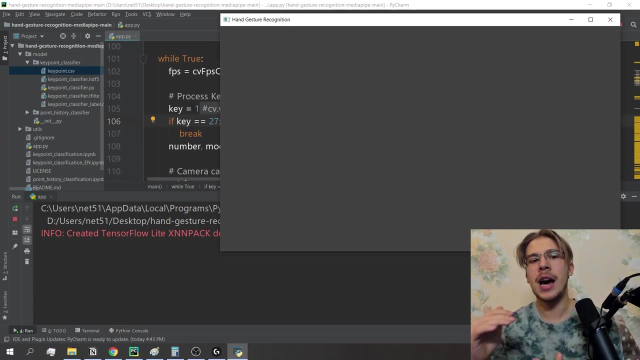 but if i say like, uh, you know, sound like that, um, if it doesn't have the white key, the window will just be like blank because it, you know, yeah, as you can see, like it's, it's completely like not working, because without a weight key, like home 2 is just, i don't know it the way it kind of adds the delay to. 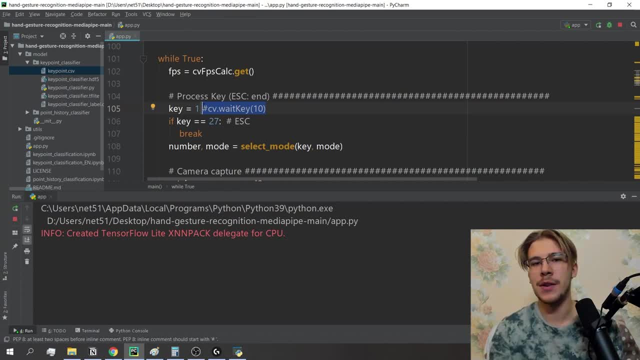 while looks so that like because there is a natural delay between the frames from the camera. you know it's not shooting in like a billion fps and it's also adding like that, that ability to like wait for user input there. but anyway, it's not so much an openc tutorial, i'm just pointing out. 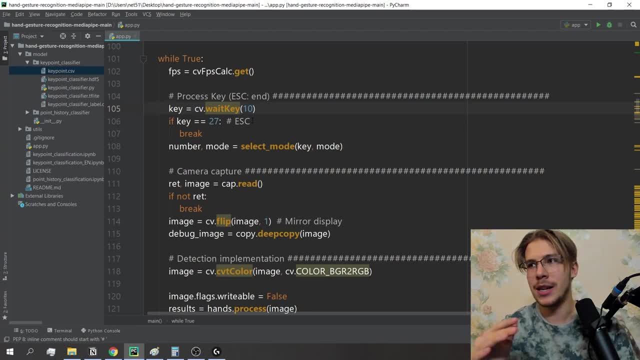 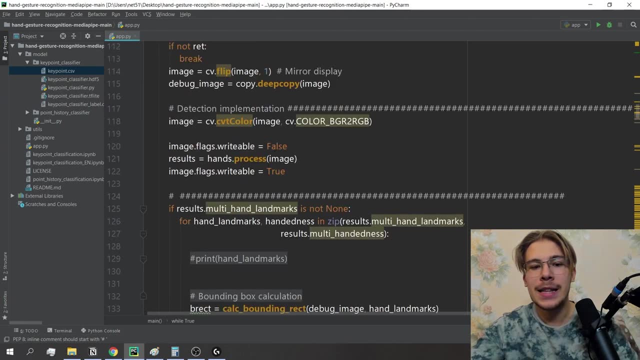 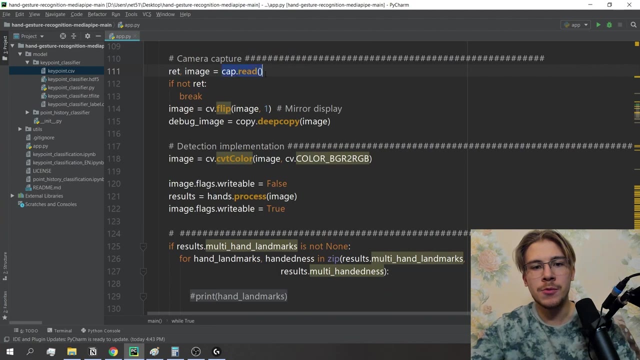 that like very general structure used in a lot of places, like very flexible in terms of how, how this thing's put together is what i'm trying to say. um, then and then and then and then we scroll back here, use here, uh, camera capture that read, uh, which grabs frames, and uh. so like this first element. 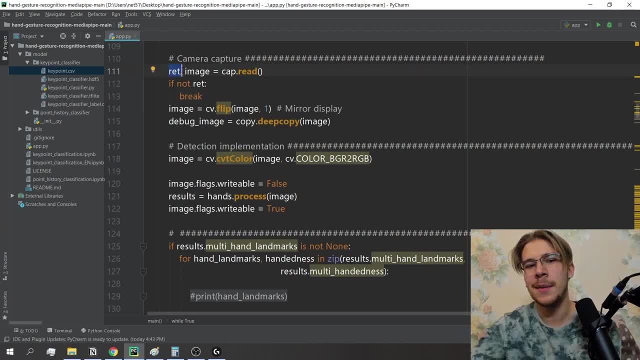 is like it's either true or false. it's false if there aren't any frames, since we're in the webcam. it's always true because, like, there are always new frames. uh, the image gets flipped and then converted from bgr to rgb because openc has its thing, but it 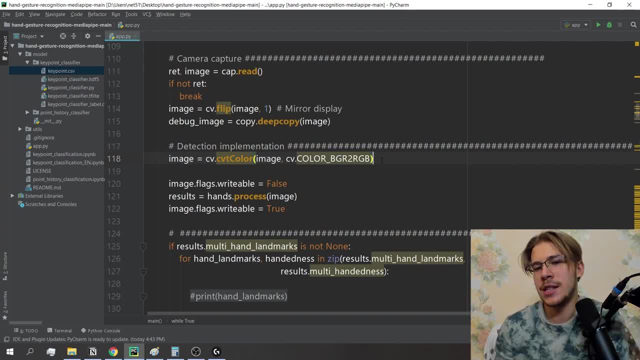 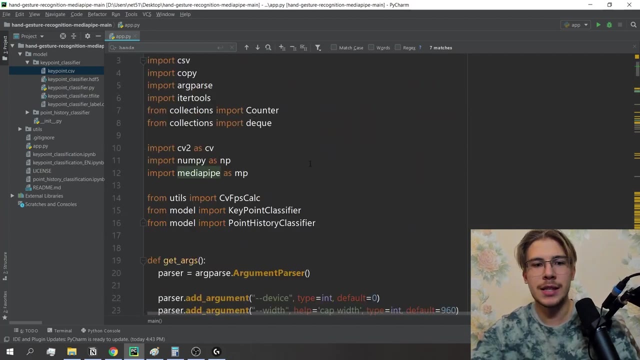 kind of prefers to have everything in bgr from from the get-go, but we can kind of convert it using this thing. then the interesting stuff happens. so, uh, this hands thing has actually been defined above and this hands thing is defined using. uh. mpmp is like a shortcut in this case, for 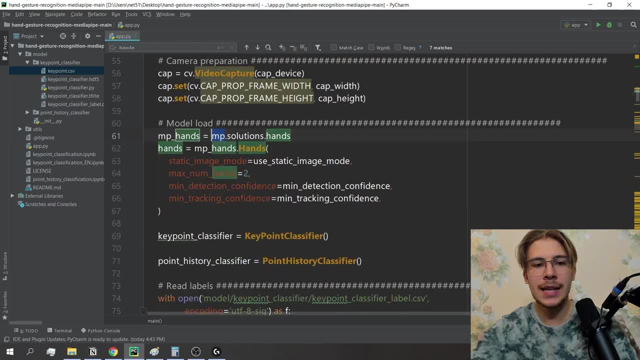 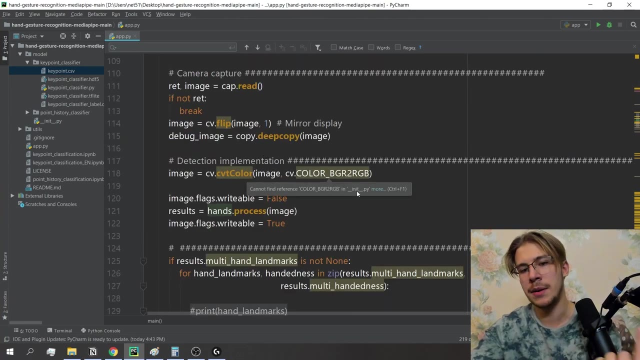 media pipe and so the hands variable here is essentially like a configured with like this hyper parameters media pipe application that's tracking hands and here in in this like openc code converting them to rgb, and then we just pretty much like passing our image through hands that. 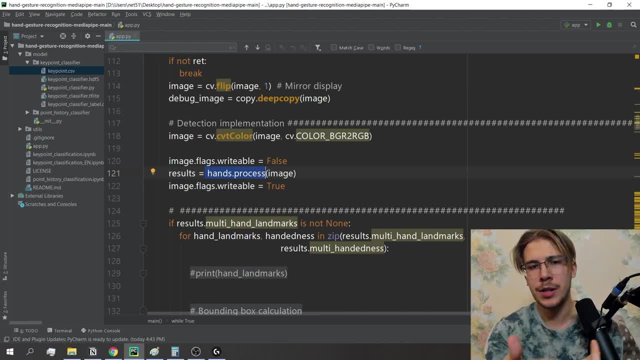 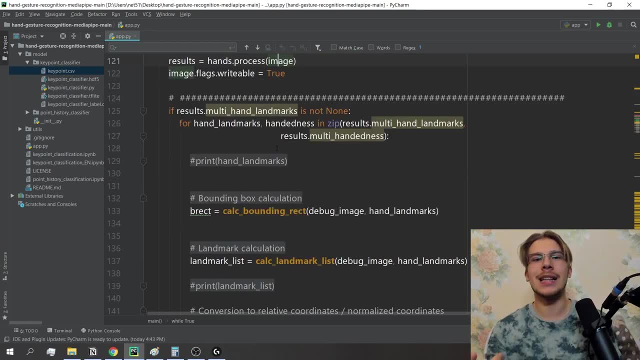 process and that in its turn, returns us the hand landmarks. um, i've added here a handful of the cool prints and what i want to do is, like it may get a little bit kind of a little at this point, but like i want you, i want you to kind of bear with me because it's it's pretty cool, i think. 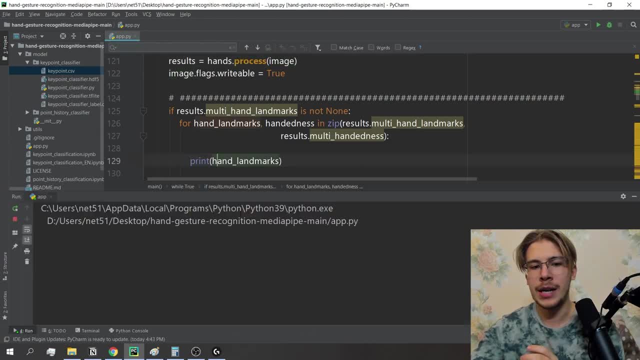 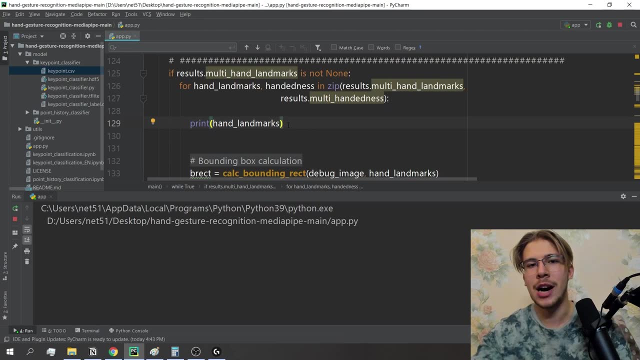 so we'll actually gonna go and start printing the landmarks, like this first print is gonna show us kind of how they're first being, how we first, like, are getting them from the from from the media pipe. um, as you can see, it's like a bunch of this points that has have x and y and z. 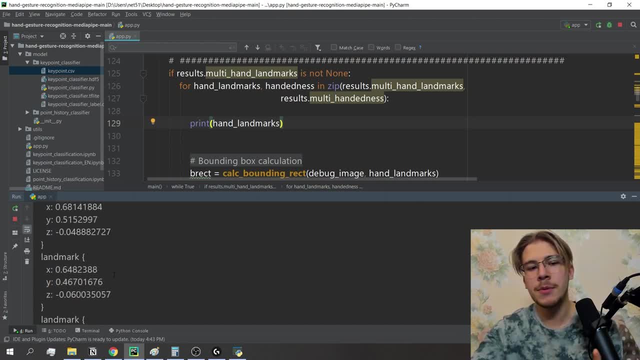 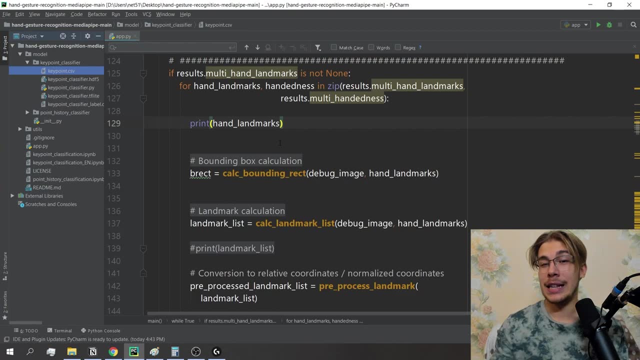 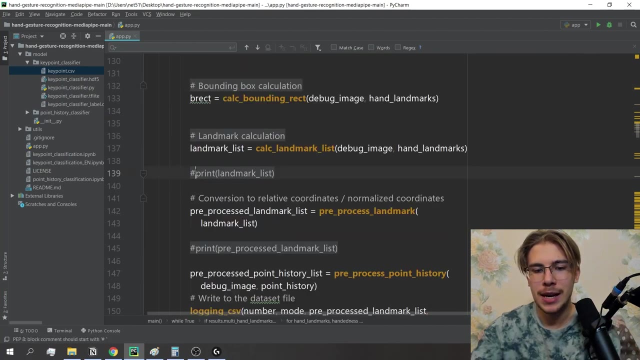 coordinates, uh, which is which is pretty cool, but that's not what we're ultimately going to be using. we're not going to need like a third coordinate for a point. we're kind of going to stick with that two-dimensional life, i suppose. so next print- and this one is a print after- after the hand landmarks get converted into a list. 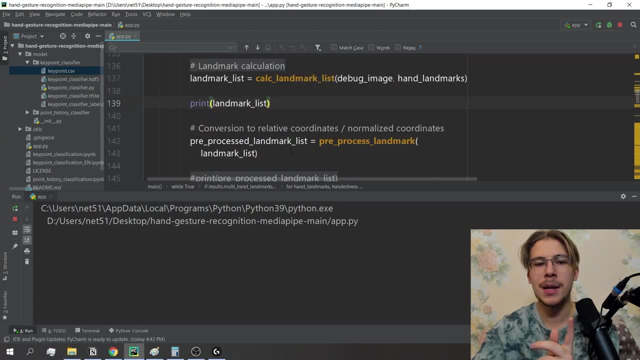 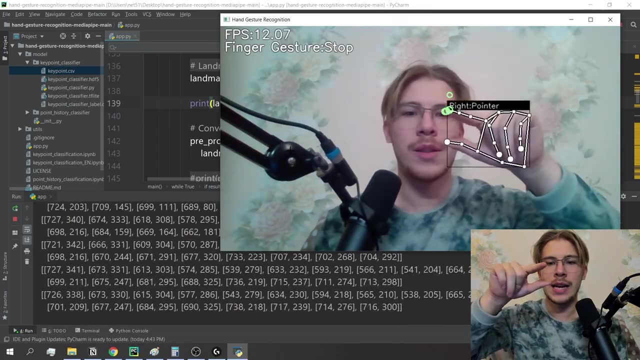 like a two-dimensional list, and this one's gonna be a tiny bit more interesting. let's check it out because, like, it's gonna be like closer to the what we're what we'll end up using. so now, that's what i'm talking about. so after that conversion, uh, we can see two main differences. so 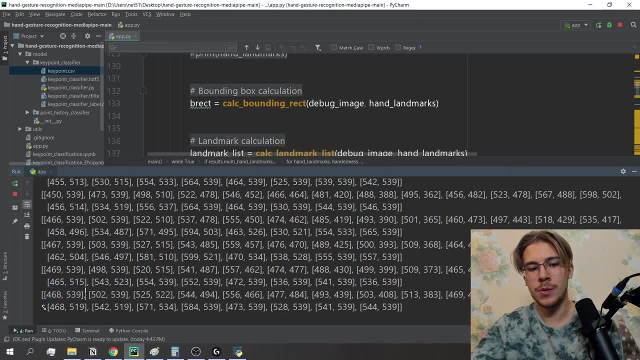 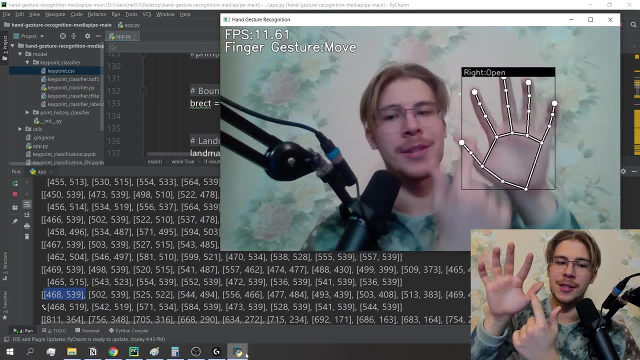 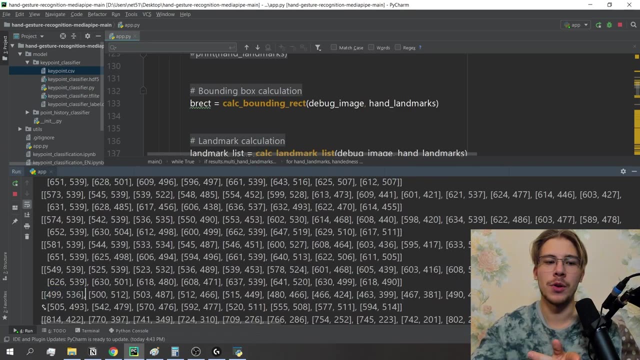 first. first of all, like as you can see there, there are just like two coordinates, x and y, pretty much per um, per point, which is also what's used to like draw them on screen and the values here are actual, like pixel values. so now let me show you kind of sound cool. so this um first point here. 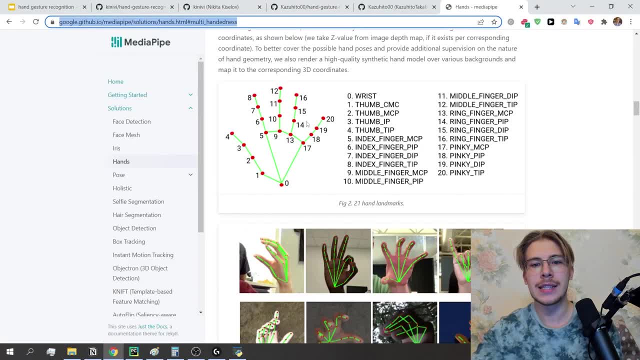 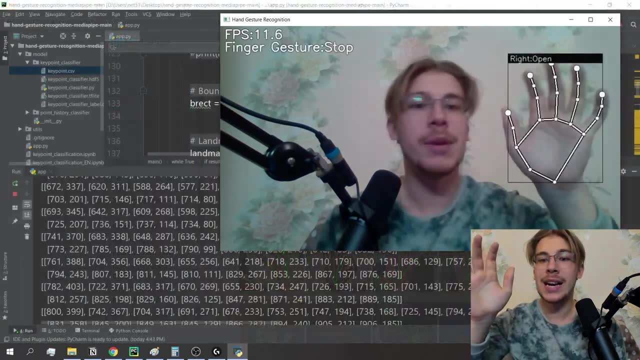 according to the media pipe docs is like it's, it's the wrist point, so like it's um, it's like this point, um, this point right here. and we can kind of see that like, for example, if i take my wrist and the closer my wrist moves, to like the 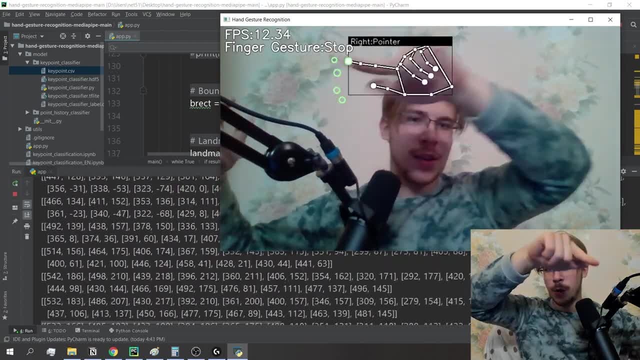 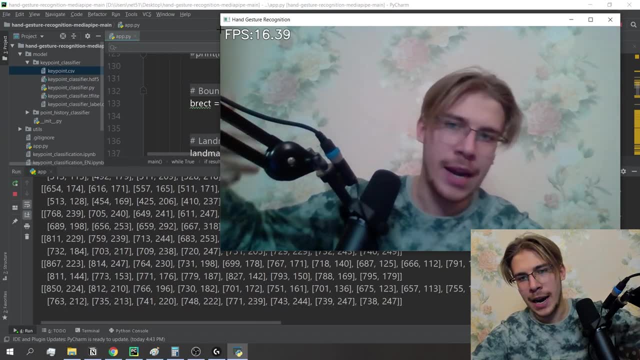 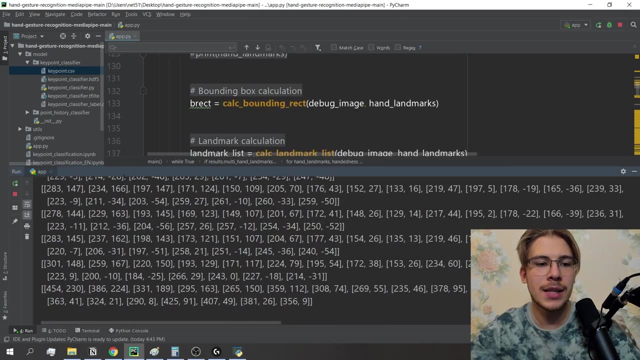 um left top corner, which is where, like in opencv, pixel life, like here it's like zero, zero coordinates, like zero x, zero y, uh, zero width, zero height. in other words, here it's like full width, full height, pretty much. so, as we, as we're getting like, let me actually do something, let's just print like: 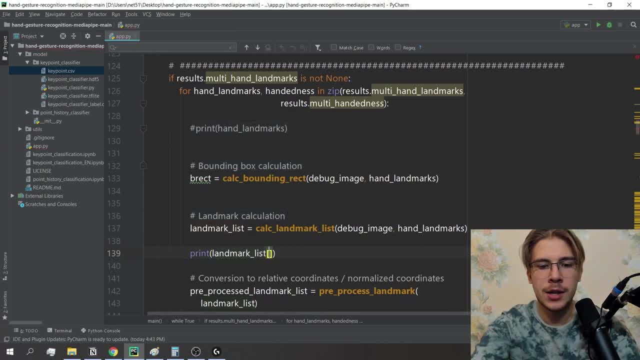 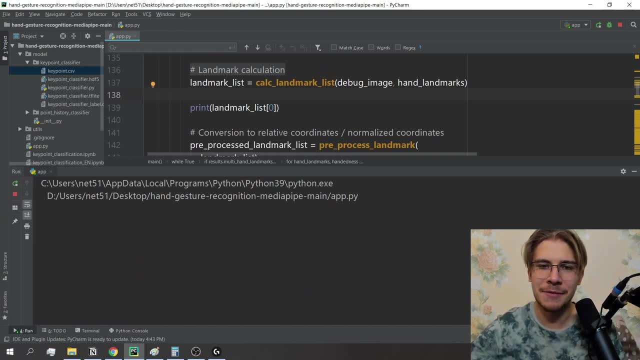 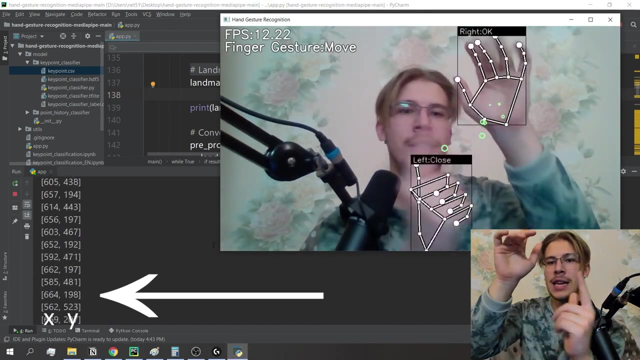 the first element, like this first kind of wrist point right here, so that like there isn't a billion of those on screen at the same time, which i get it. it's like it's confusing, um, so let's do that. so now i'm just printing, like the this, like zeroth element on that, like 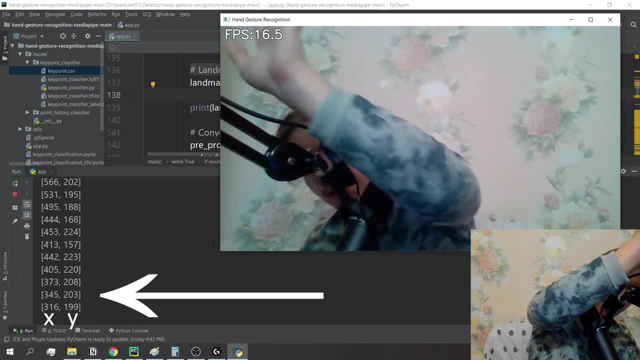 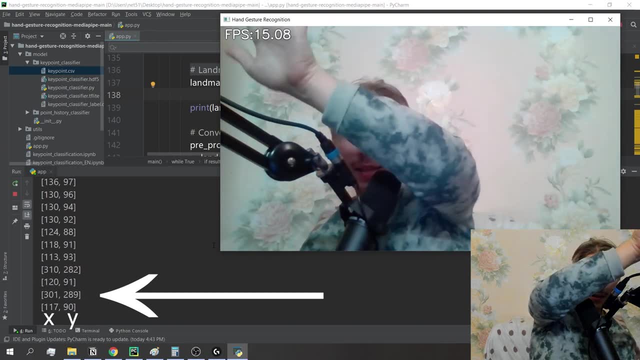 process list, which is like the wrist point. um. so, as you can see, like the closer it gets kind of to the left half corner, like the lower the values are. i'm just trying to get it like as close there as i can without losing it and like as closer it gets like to this place, the larger the values get. 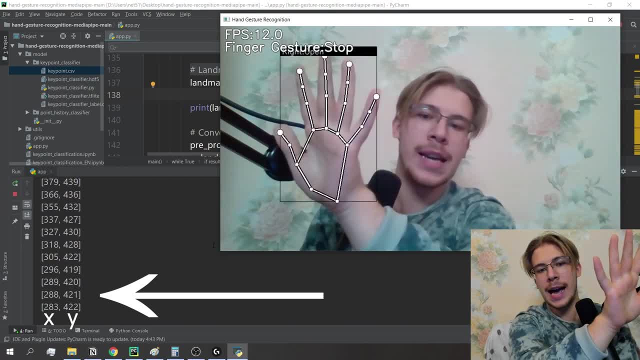 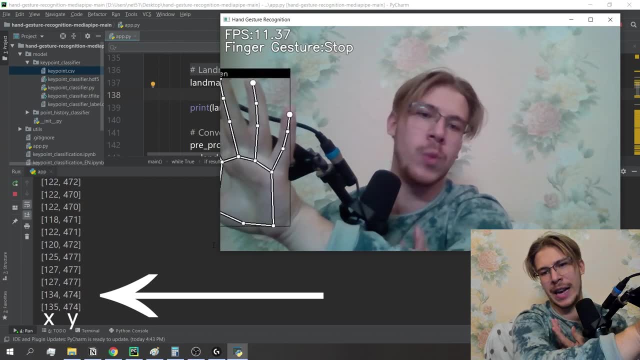 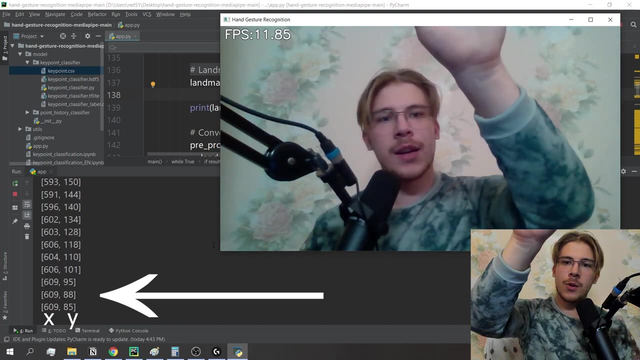 in general and if, if i move it here, then the x values get really, really small, while the uh like, while the y values, like the height values, like the- yeah, the y values, pretty much they stay in the same and, on the other hand, if i move it somewhere, like here, the y values are really 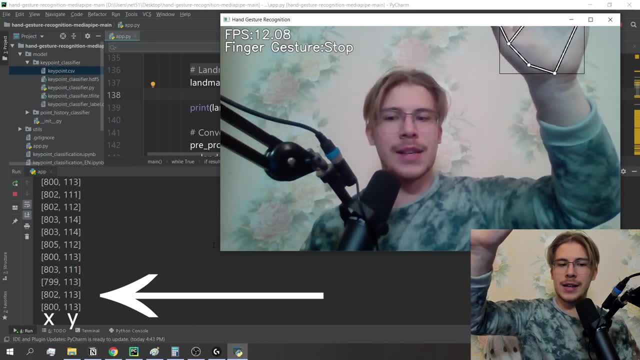 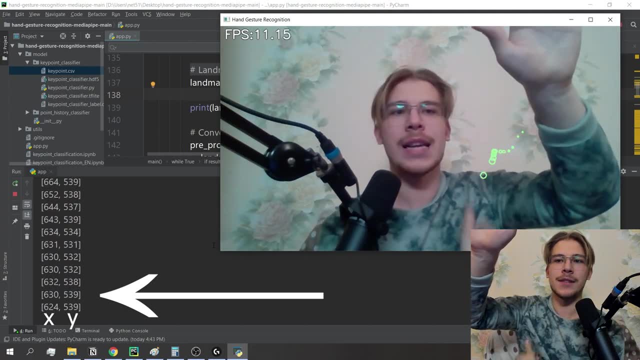 really low. as you can see, it's like 100, 115, 800, 120, stuff like that, in terms of the y values and the x and the x values in this case are like 700. so like you can see kind of how- uh, i'm using the 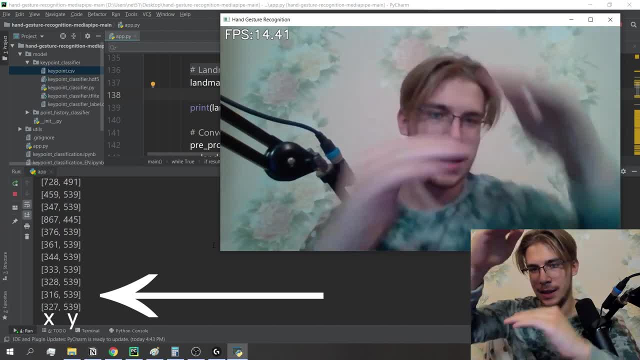 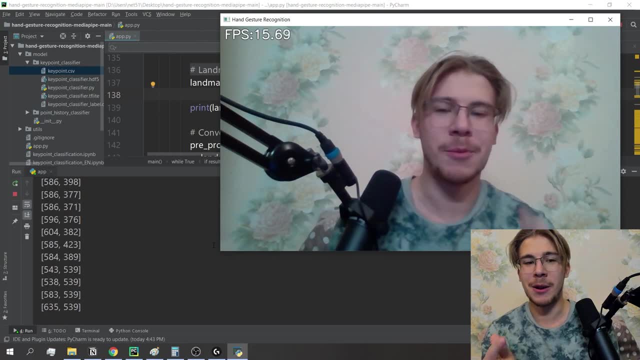 one point, how they're represented at this point in the like processing pipeline as like the absolute, like pixel values. um, there are a few more steps coming in terms of like processing them, but but it's like a cool intuition to know that like these things aren't just like. 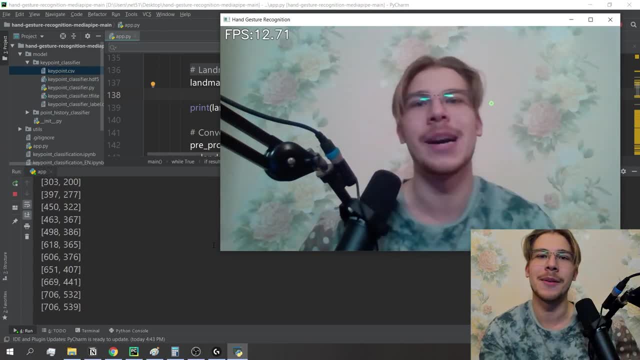 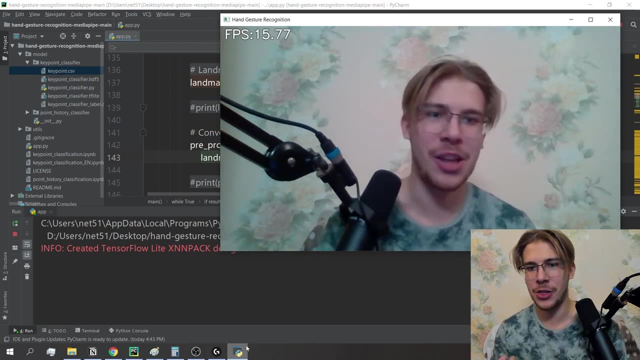 printed, that's they're like actual values that we can understand where they come from, you know. now the next part is really really cool, but behind the scenes i was kind of bashing my head for the last like 30 minutes because i was thinking like how do i best explain it? 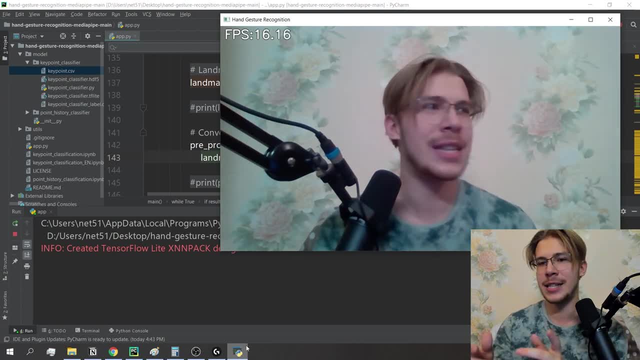 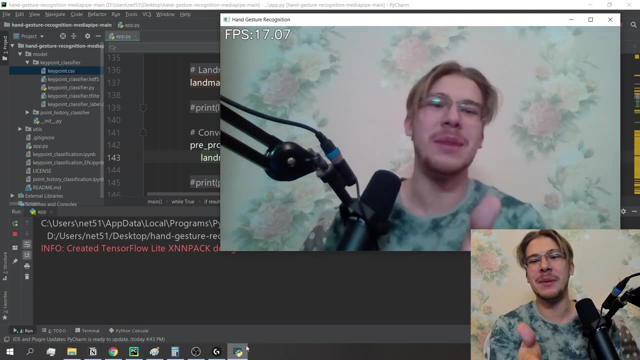 because, like it's, it's it's really cool to understand, it's really crucial to like understanding how that like final part with the feed forward neural net is gonna work. but it's like it's a little bit convoluted, but i'll do my best and you just please bear with me. 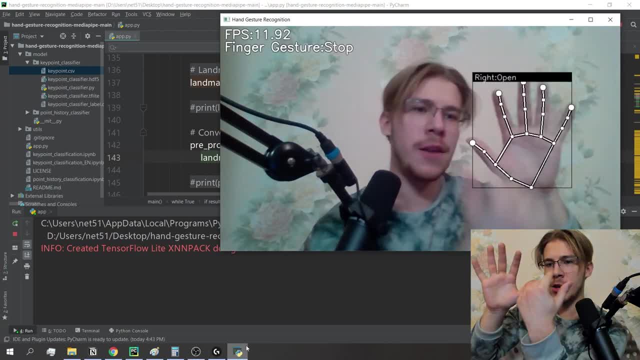 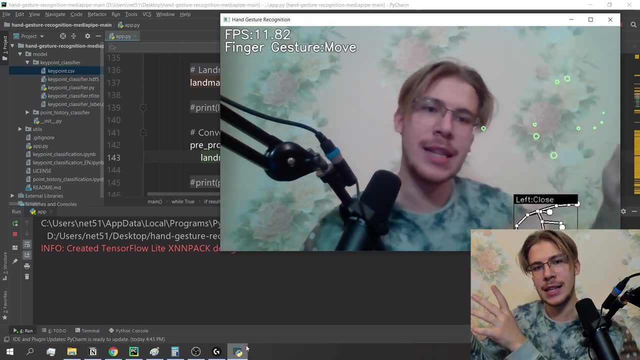 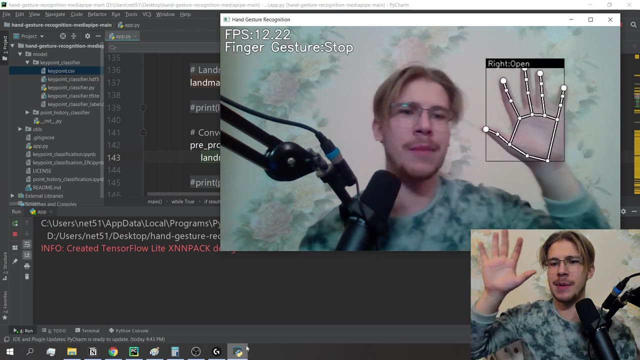 okay, so like the whole concept of a benefit of using like this, like landmarks approach for for fitting that into, like that feed forward neural network, you know, in in the last step pretty much for classification, is that, um, we don't have to worry about the position of the hand, like where it is, and we don't have to worry about like the i don't know. 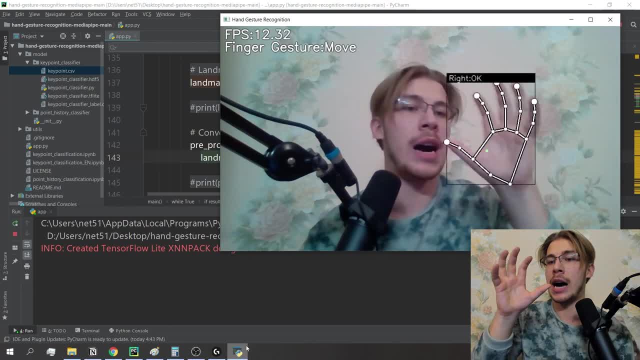 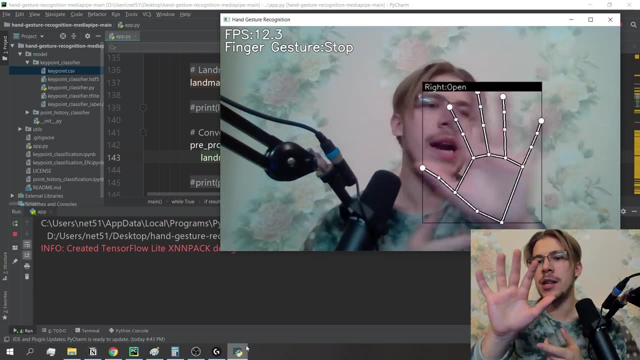 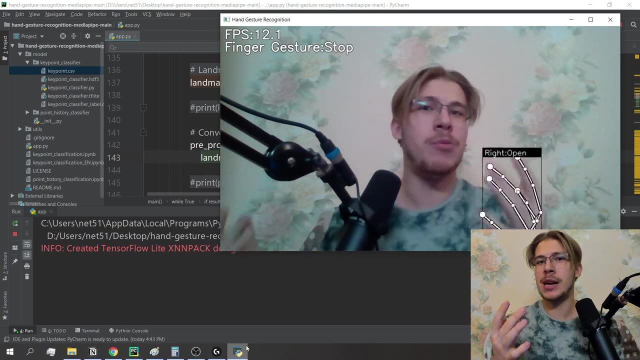 the individual, like shape or color or whatever of like of a given hand or like the background, you know. but with that we need to find a good way to pre-process the, this landmarks to be fed into a feed forward neural network, and pre-processing is, like it's like, a very crucial. 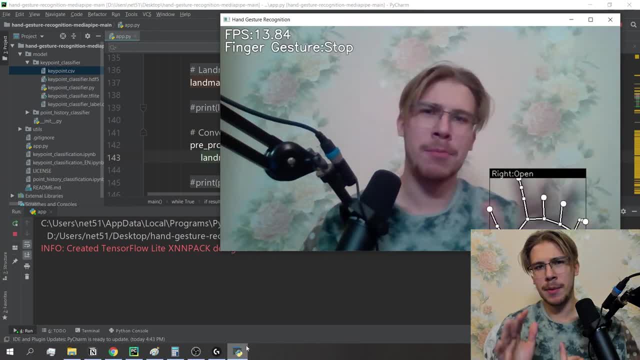 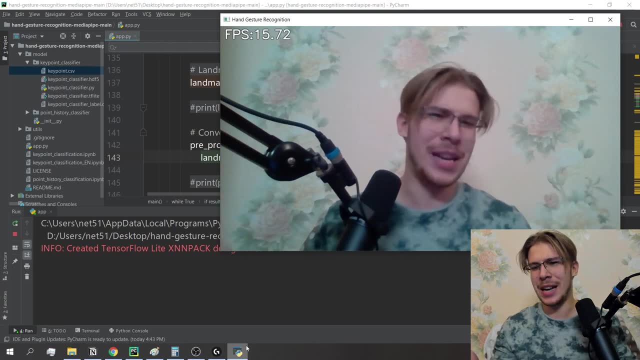 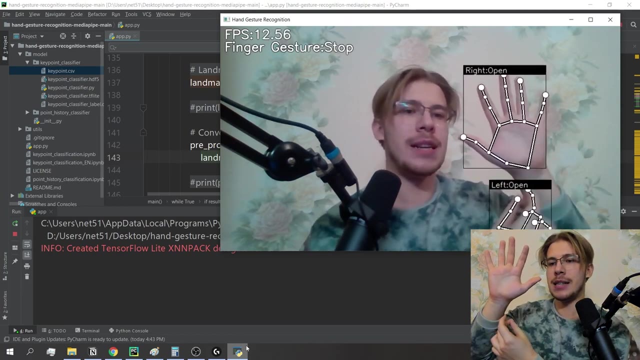 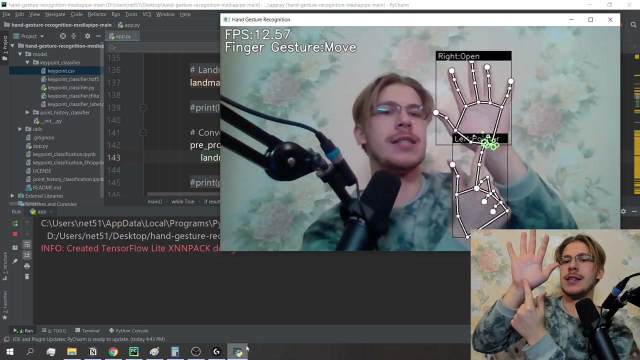 concept that pretty much thinking about how to like properly pre-process, it is like it's like half the battle many times, honestly, because really um the so right now we have a problem, as we have seen with this, values being defined as like absolute pixel values like, for instance, i don't know right now my the value of like this, this, like wrist point right, like on. 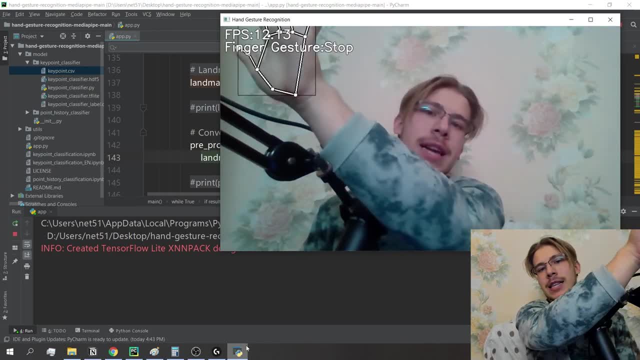 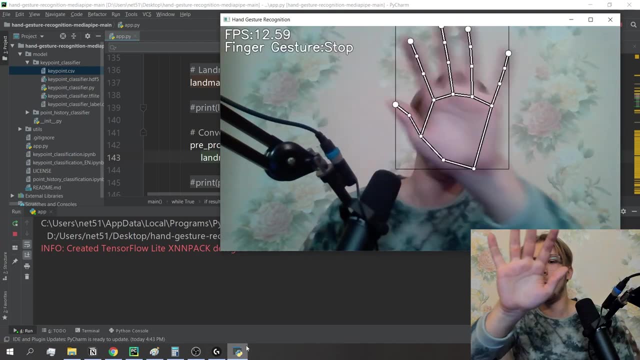 my wrist like the zeroth point. the value of this guy right here is like close to like i don't know. maybe it's like 50x 50y in pixels coordinates, right, but if i move my hand here right now it's going to be like i don't know. 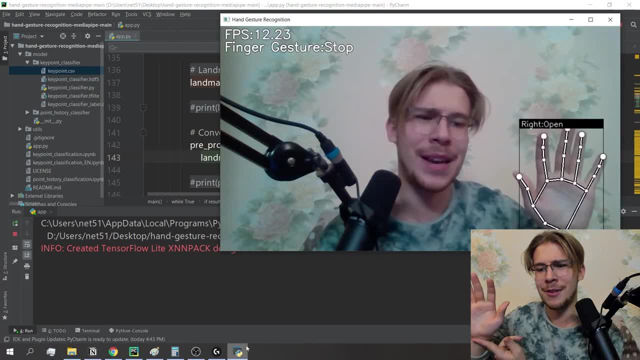 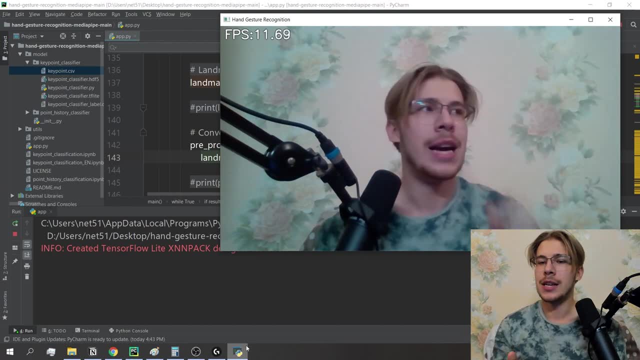 400x and 300y or something right. so same applies like all of this, like other um 24 points on the hand. so what's the problem here? well, the problem is that, like, if we feed that to neural network somehow, the is like. this is like a vastly different hand in terms of values. 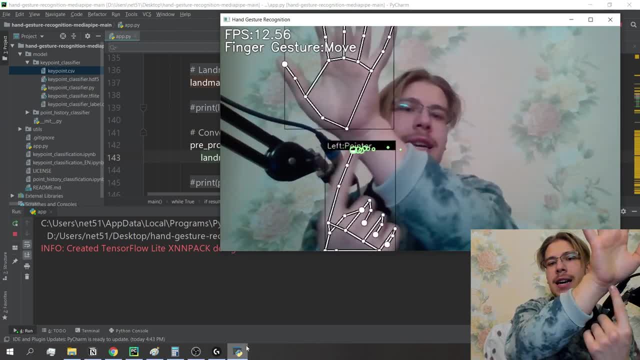 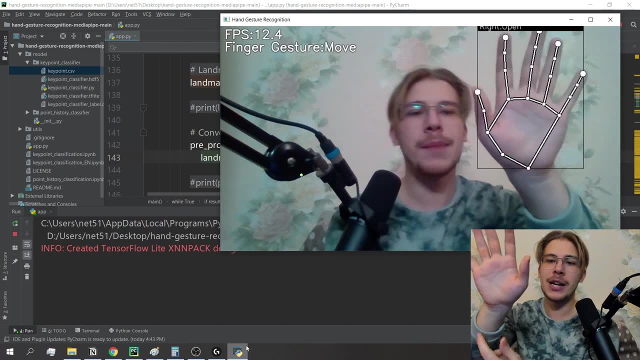 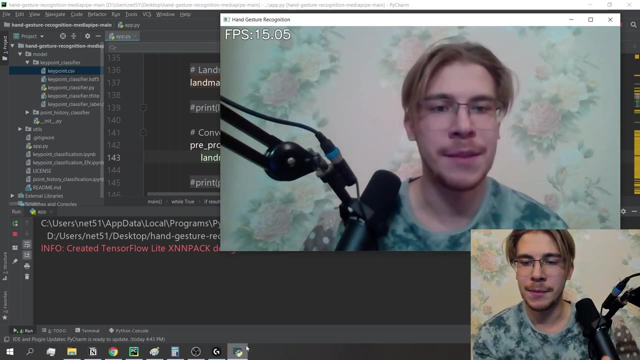 than this hand, like, if we just like focus on this point, like this wrist point and this wrist point, like, say, like these two points, right, like this guy and this guy. they're pretty much on the same distance relative to each other here as they're here, but, like, their values will be vastly different because, 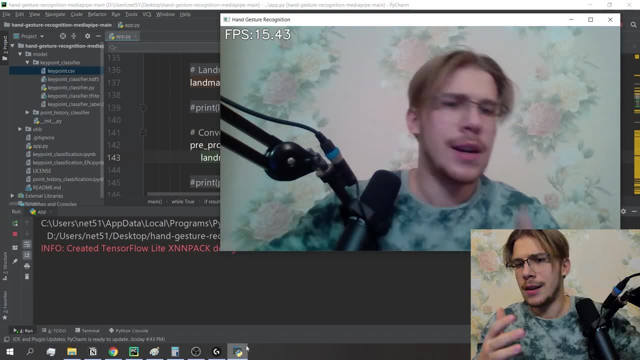 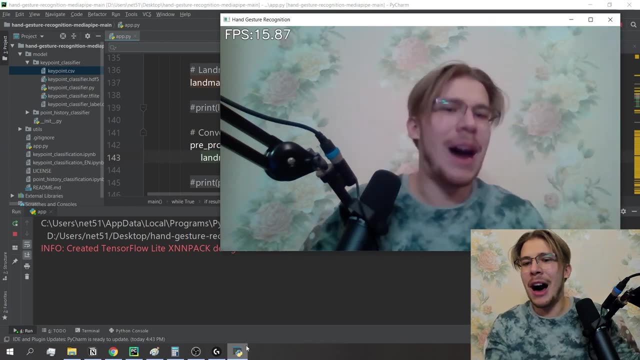 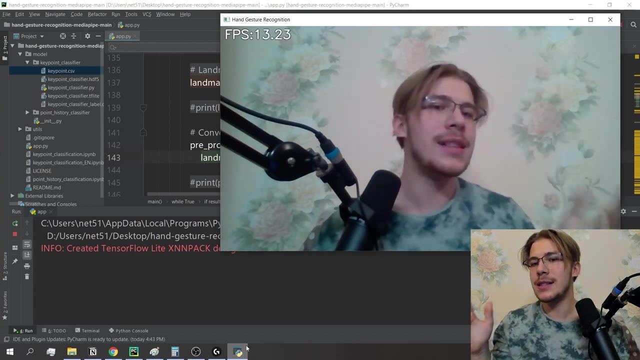 right now, the representation of hand landmarks that we have is, like you know this, like list that we've- we've processed- well, not we, the author of the repo, but you know what i'm saying- is heavily relied on, like the actual pixel values. now it's not just rely on them for the 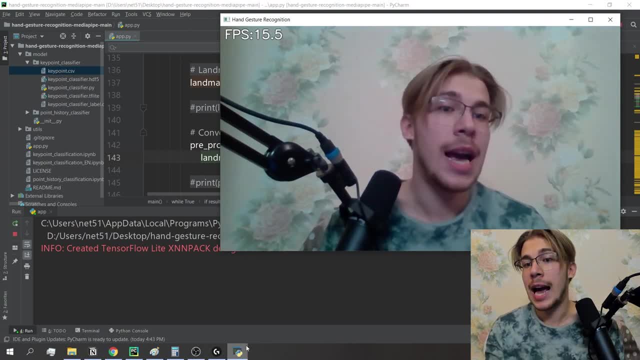 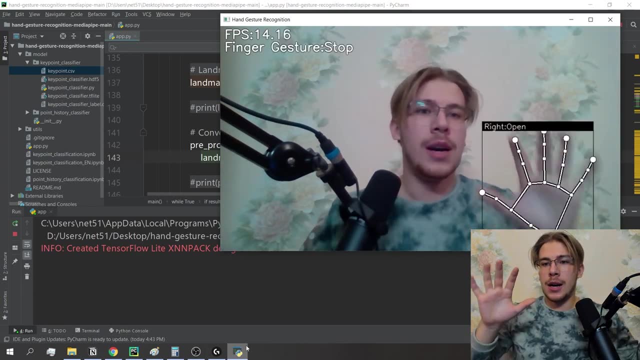 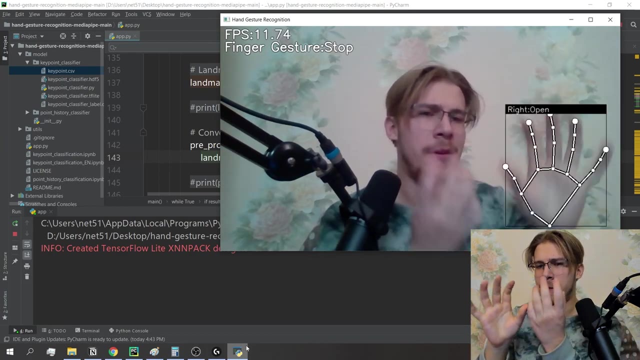 sake of being relied on them. it's right on them because, like there's a next step um coming up and that next step will pretty much address this very problem. so to to address it, we need, like some sort of system where this landmarks when they're going to be fed into a neural network. 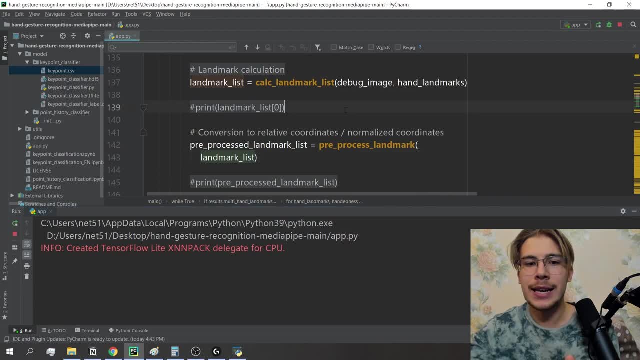 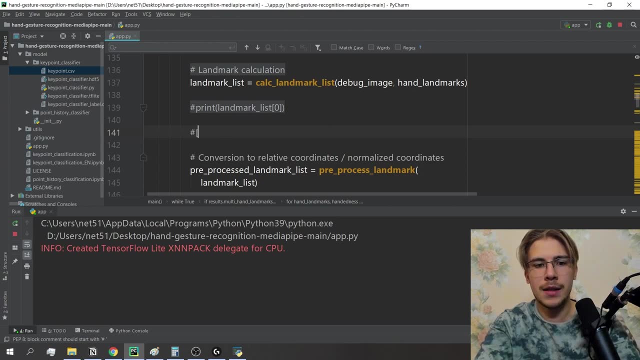 and they're going to be fed, by the way, as a vector, as a. as a vector which is like a value, which is like a one-dimensional list of numbers which will look something like this: like 0.5 minus 3.4, point minus 0.4, 0.1, you get the point where they're going to be like pairs of x coordinates. 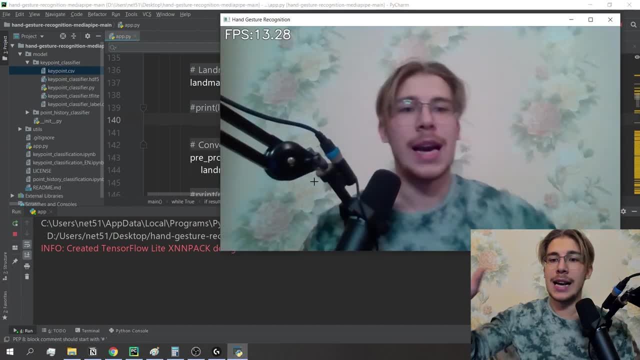 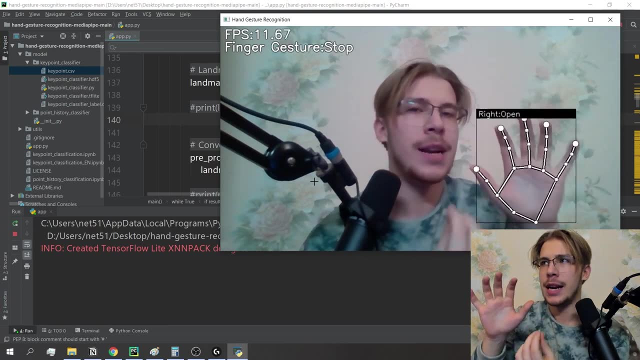 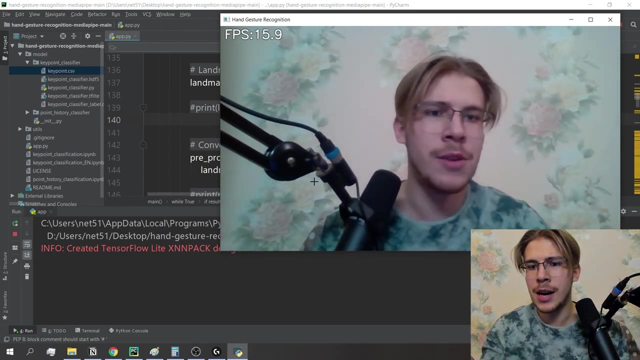 and y coordinates, kind of as we've seen with the uh, with the wrist point, and so we gotta somehow convert this like absolute pixel values in terms of the frame, into like some relative values where this hand here and this hand here will have roughly the same values, you know, and that's done. 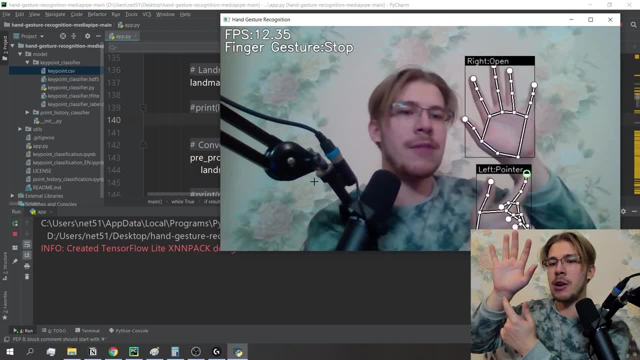 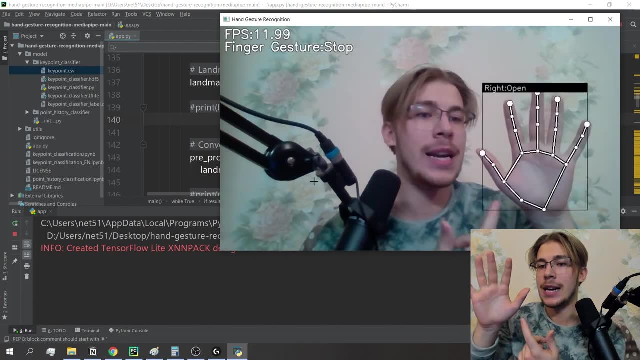 through a process called, you know, normalization. where we're like normally, where we're gonna like normalize these values, uh, between the ranges of minus one and one, and in this way, and i like, and then i have like the whole like little painting prep here for that. that i will dive in a second. 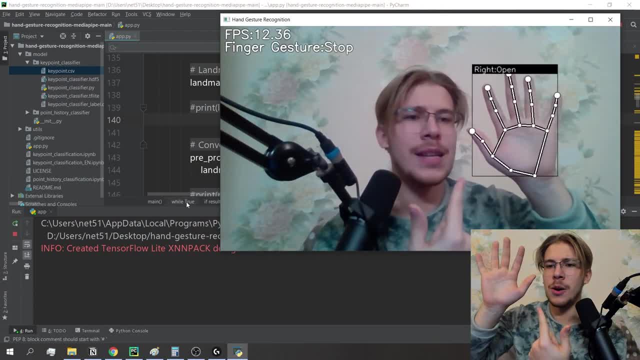 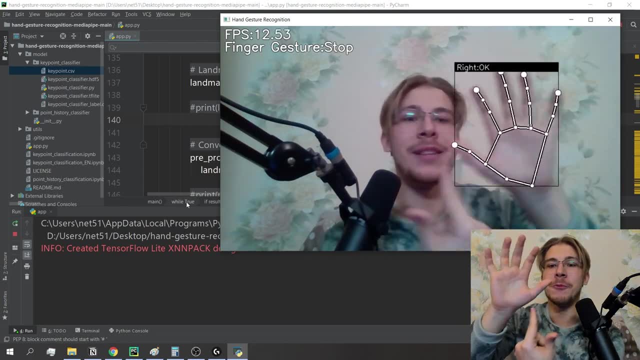 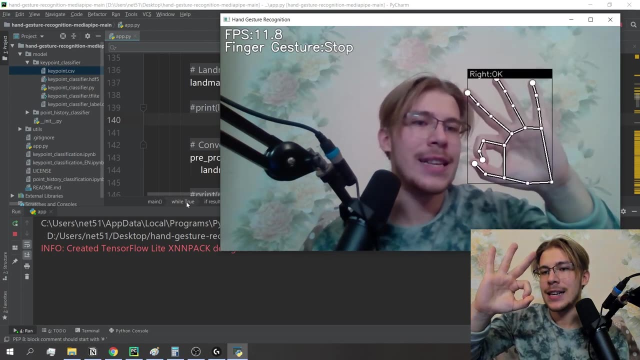 but for now, like basically, uh, you know, we'll, we'll follow the algorithms, we'll we'll dive into what they're doing and what are the actual like way that we can, ways that we can like normalize this whole thing so that it's like relative to each other, like this hand, which isn't just gonna solve the problem of hand being in all. 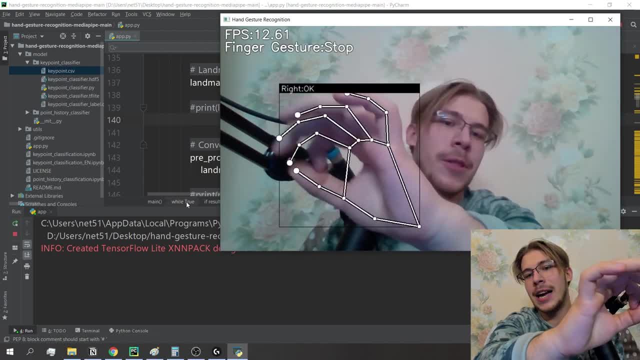 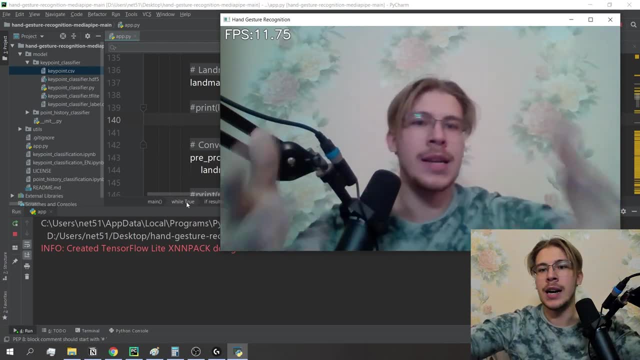 sorts of all sorts of different places, like it's also gonna help with. like you know, if my hand is a little bit farther away or if it's like a little closer, as you can see, like the distance has kind of changed, but like, if we normalize it to like the other way around, it's going to be a little bit. 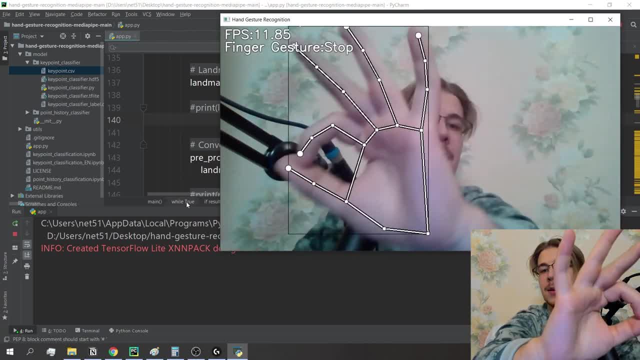 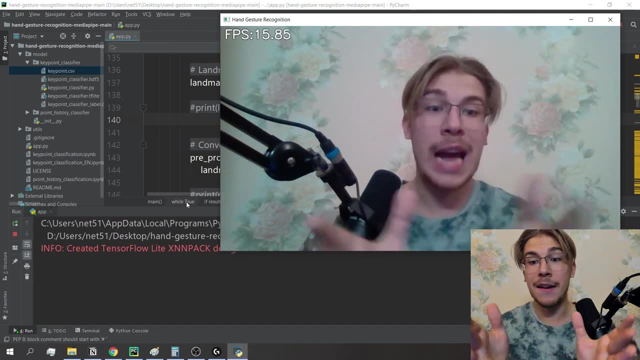 different, but it's not gonna be like the relative coordinates, like this thing will be roughly the same as this thing. so like the all the like scale problem problems will also be like handled in this way. so now let's dive into like the actually like what's going on, this like pre-processing. 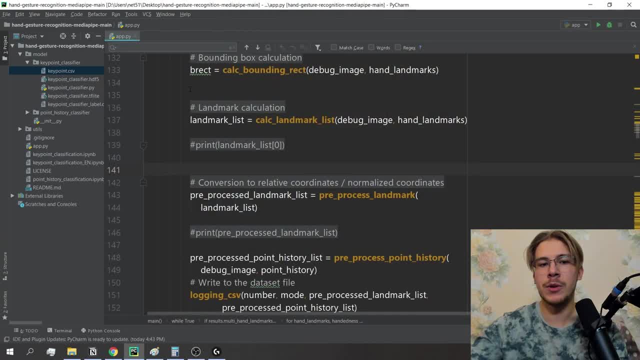 algorithm in this case, you know. so, next up in the code, this like listed the list that we've talked about of, like you know. uh, absolute pixel values, like in the frame, gets passed through a pre-processed landmark function. that's, that's doing like all the like conversions. 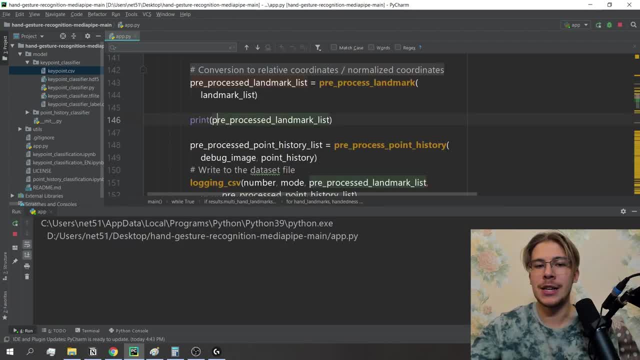 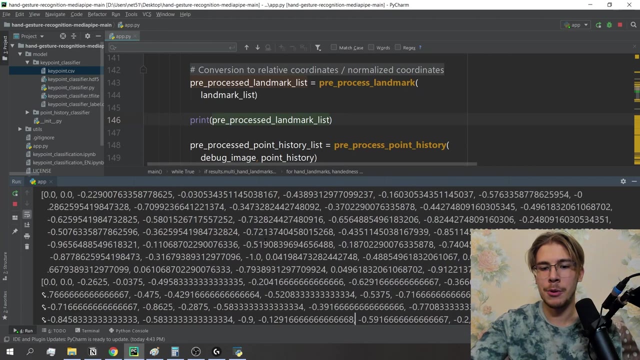 and upon the like output from that function, we can see how this values change from being like absolute pixel values, to being, um, let's give it a couple seconds to load, uh, but to being like this, um, floating point numbers, uh, with the values not surpassing, you know, minus one or one, in a way that 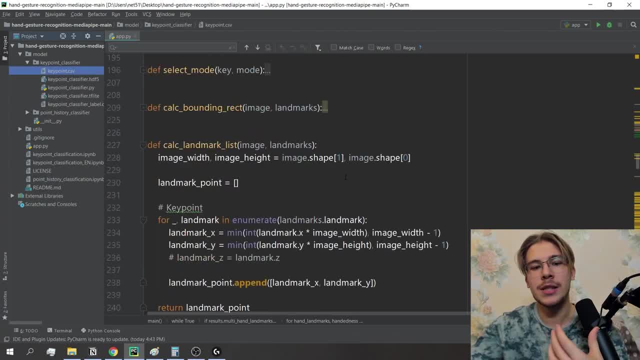 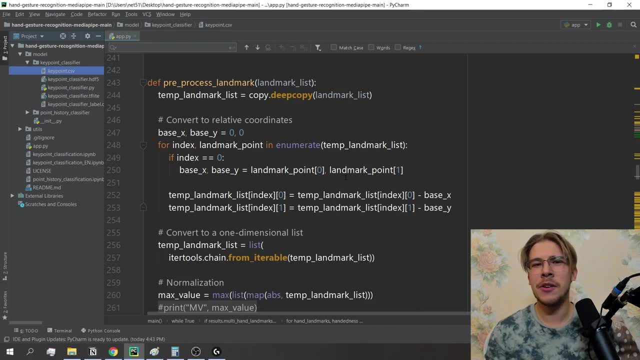 they're being like, normalized in this way, but like it would be really cool for us to understand, understand what's actually going going on behind an algorithm, because before doing this video, i kind of had, like, uh, an idea of what i was doing, but like when i actually 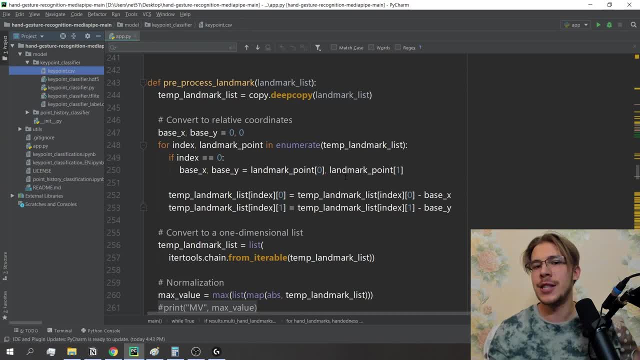 started like i kind of had like my idea, like how i would such thing. but the thing that, like the author of the repository did, you know, like it obviously does the job and i think it's pretty cool and it's not something that i would have thought immediately at the top of my head. so 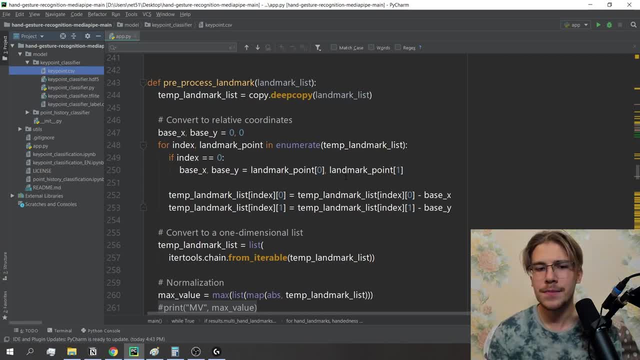 i think it's like worth taking a dive into it. so um first thing that happens here is that we create this like temporary landmark list, um copy, which is essentially like that you know list of, but remember, like this, like uh, pair values of, like pixel values that look something like this: 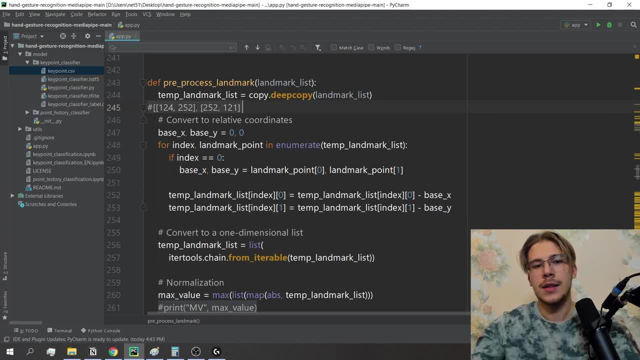 you know where, like x and y, and there's like 20, 24, right, oh, no, 20, sorry, there's 20 of them, yeah, of this like pairs of hand landmarks, and so the first thing we do here is like we convert this whole list to relative coordinates. now, what does that mean? relative coordinates? 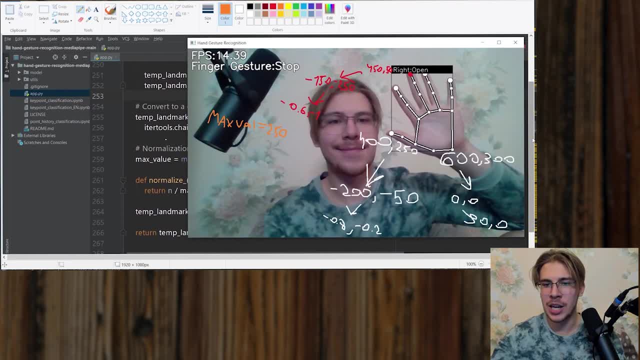 i kind of have like a little- uh, not fancy at all, i get a thing that i drew like in paint. but, for example, let's imagine that this is our wrist point, right? this is our like point, with the index zero, uh, right, so in this case, the process of converting everything to relative coordinates, 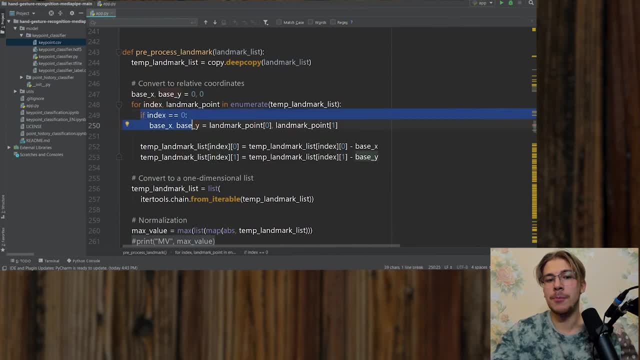 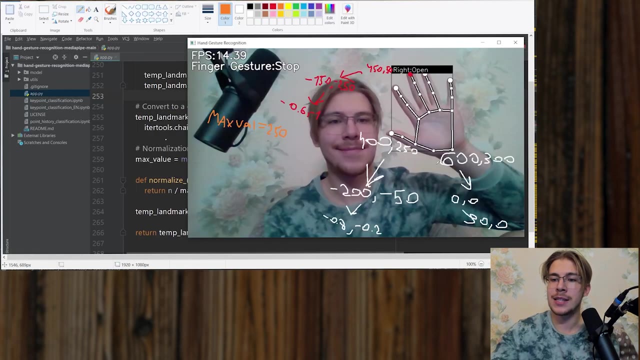 is done through um taking the point with the index zero, aka, like this, like this, like wrist point, and then subtracting that base point from all of the other points, and this is kind of what i'm doing here, for example. for example, like this is our um base point, like our wrist point, and it's the 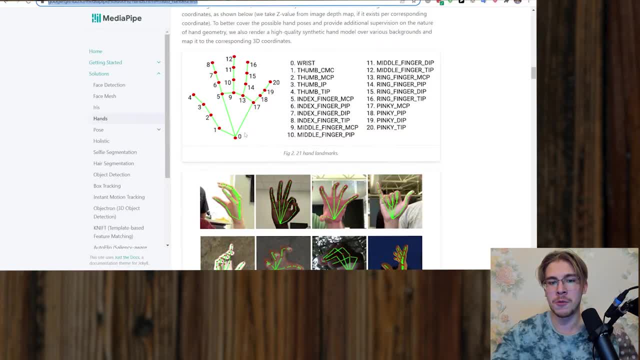 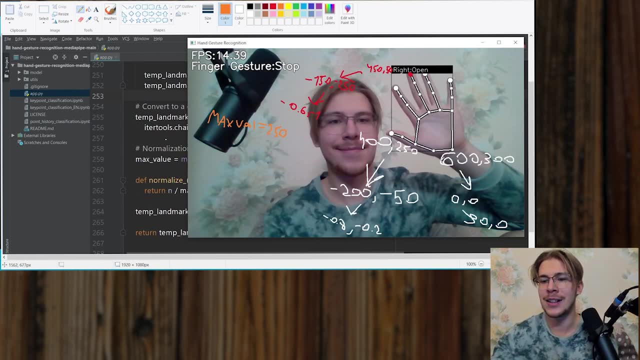 base point, because again it has the index zero, because again it has the index zero right here. um, we subtract from it and we'll subtract from every point we've got subtract like this kind of like base point, and if we subtract, like bass Auslan, from itself we get zero, zero, and so 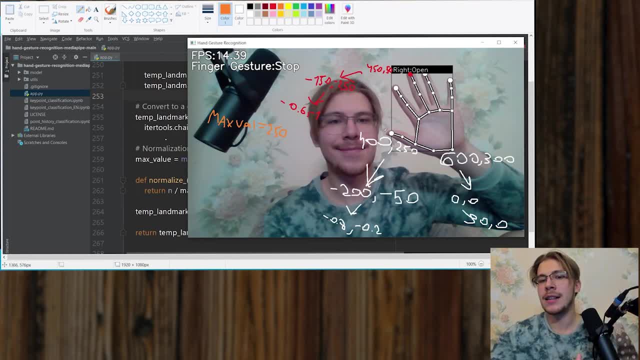 base point minus base point is like zero, zero, let's say. let's say, for instance, we're looking like at this point right here, right, uh. let's say it has coordinates like 400 to 50, like it's a little bit to the left and a little bit higher than like this guy right and remember, like this. 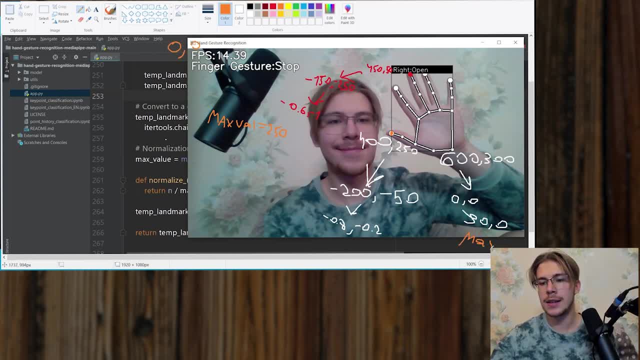 is like zero, zero, and here it's like max, max in terms of like x and y coordinates. so for this point it'll be like 400 minus 600 will be like minus 200, and 250 minus 300 will be like minus 50. so in this way, by performing this operation for each of the points here, we get kind of like: 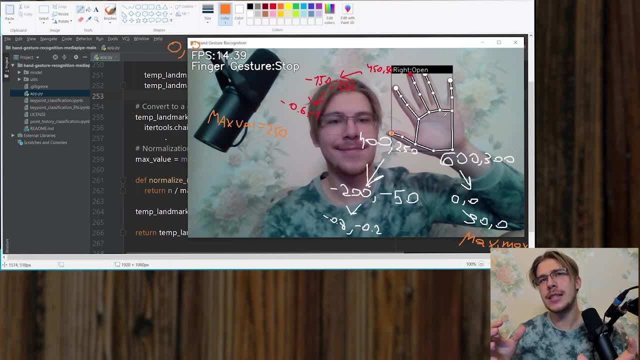 relative kind of like each points become represented as as of their distance to the wrist points. like you know, this point is like this far, you know this distance, etc. etc. like each point gets like represented as itself minus the base point and that's where get represented as like how, how far away it is from. 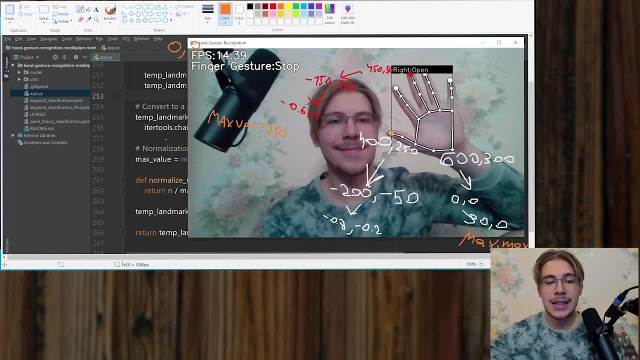 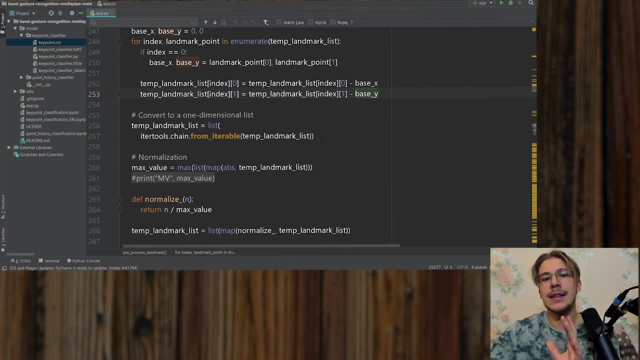 the base point, actually, you know what i mean. uh, then there's so like that's, that's pretty much what. what happens like here? um, then that happens for like every point in the list and it gets converted to a one-dimensional list because the input to the feedforward neural network it's, it's. 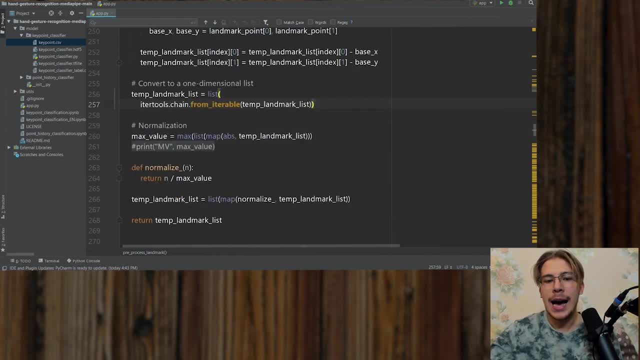 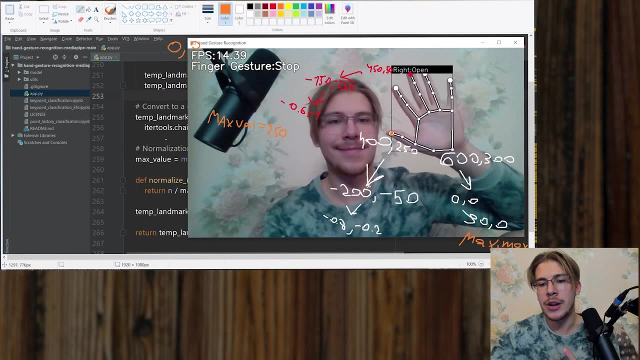 going to be like a vector, a one-dimensional list pretty much. and here's something another really interesting thing happens. we get like, like, like, we get this like relative values here, but they're still like minus 200 and minus 50 or like minus 100 minus 250. 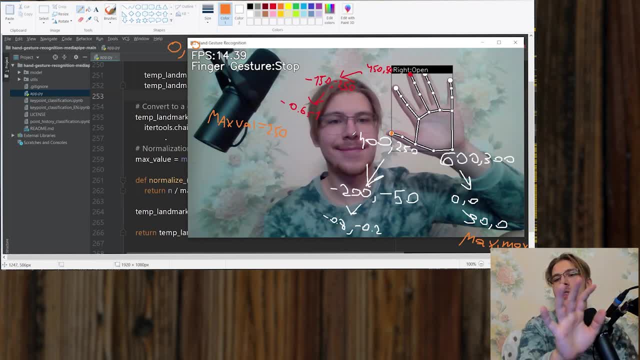 they're. they're dependent on, like, where the hand, the hand is in the frame. pretty much. you know what i mean. so, like, they're not relative, they're, they're. you know if a hand would be like, you know, if this hand were to be moved slightly to the right. 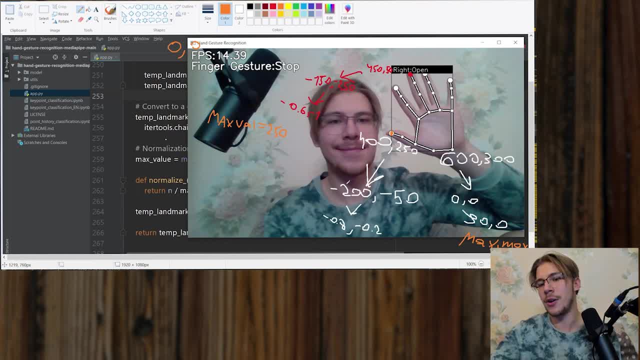 this value is get pushed like, let's say, this thing would be like 700, like this whole thing would be also pushed by like 100 pixels. you know what i mean? it's like we gotta normalize them between like this, like more floating points, like values between minus one and one, pretty much in. 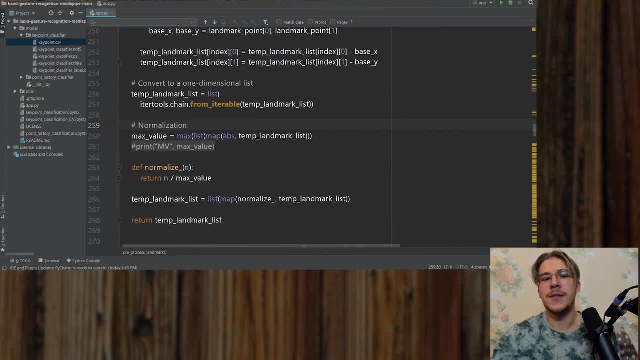 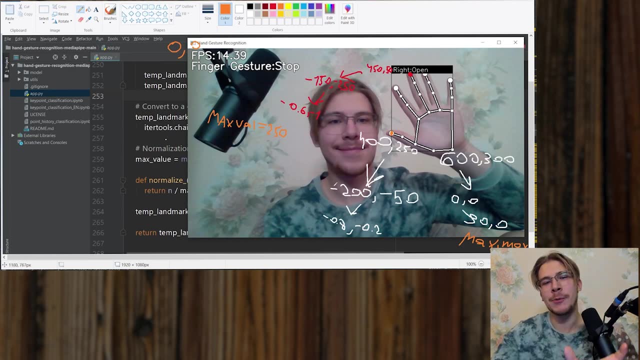 this case. so the way that it's done by the author of the repo is we take the maximum value, so like, so we end up with this like list that that's still like, expressed in like pixel values relative to the, to how far away from the. this like like. 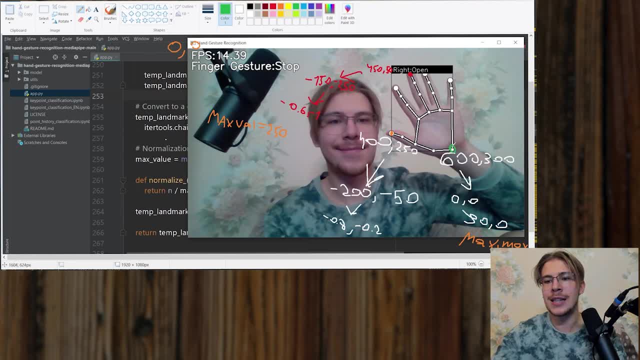 wrist point. uh, let me use like a different color. let's pretend like, let's pretend like i'm drawing something fancy in paint. you know what i mean? uh, yeah, it's like we, we get like a list that's filled up now with with like this value, so like zero, zero minus 200, minus 50, minus 150 minus 250, but it's 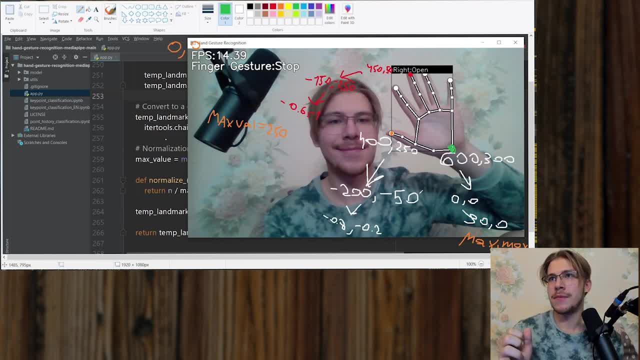 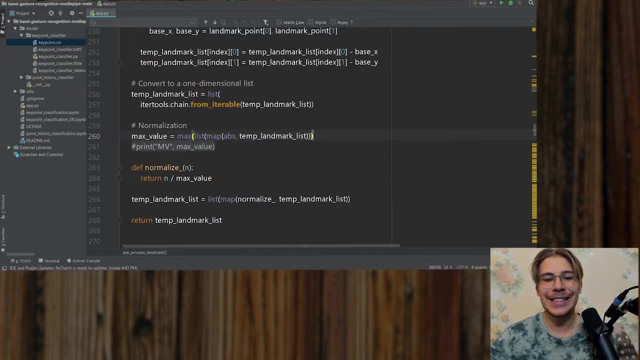 still like pixel values. you know it's, they're not like relative. you know normalized floating point values, you know, and we get the floating point values by uh, taking this list of like relative values and finding a maximum value, and then we get the floating point values, and then we get the. 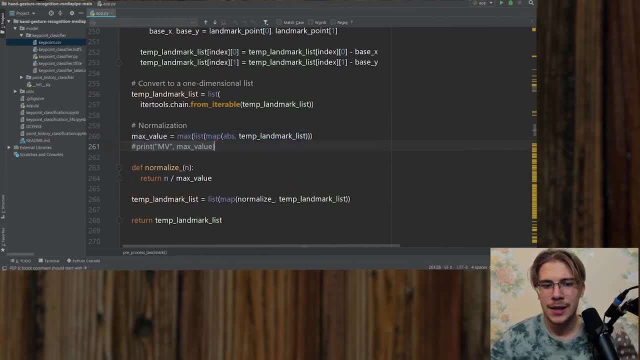 value on it. so what this expression here does is like: uh, abs, map, abs stamp, landmarks list. it's essentially like disregarding all the like whether a number is negative or positive. it's just getting like absolute distance. so, for instance, we have like a list that looks like this: like minus one. 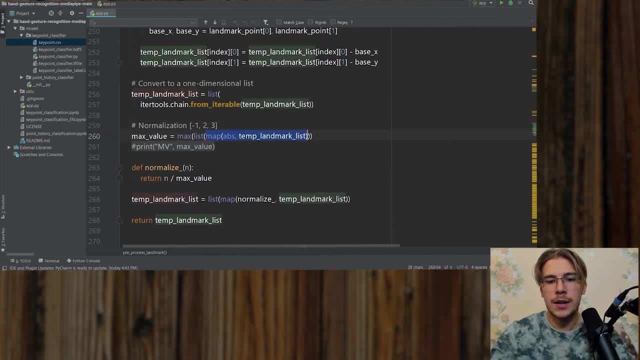 two, three, like this part here, would convert it into like: uh, one, two, three. pretty much it's useful in our case, because what we're doing here is that we're taking all of this values here and we're converting them into, like this, like absolute length, distance list. you know what i? 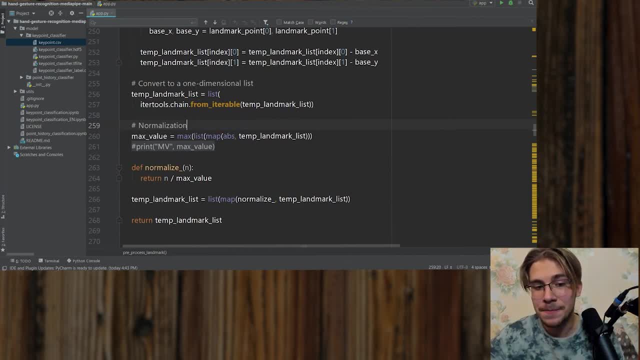 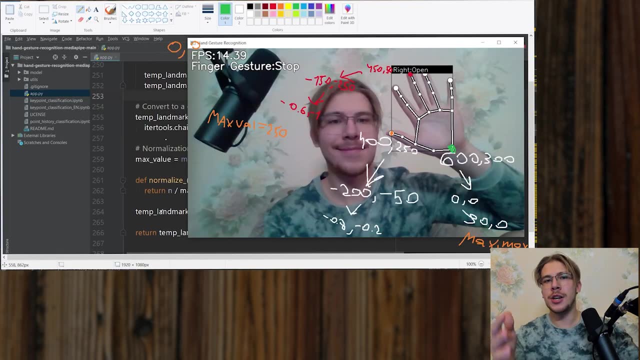 mean, and then we're finding like the maximum element here and spoiler alert- then all of them get divided by the value of the maximum element and so you may kind of ask them like, how does that look in this, like actual drawing? so the point that's like far the 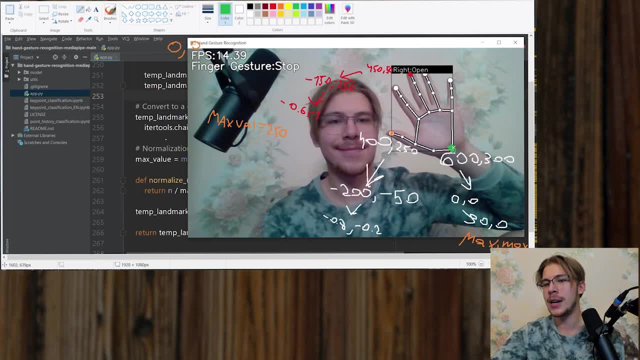 that's like farthest away from the wrist point here, from like the zeroth point is. i mean i kind of eyeballed it here but like i'm assuming that it's like this guy here and i'm assuming that it has values, uh, 450 x and 50 y, you know, uh, such that when we um perform this like subtraction, 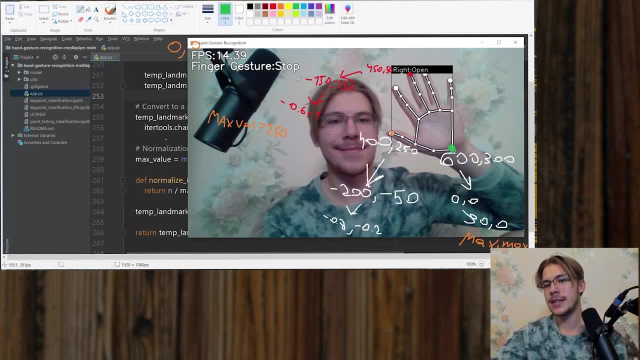 where we take 450 minus the base 600, in this case it's like minus 150 and uh. 50 minus 300, like minus uh. it's like. this is like our distances pixel values list, right, and we perform that for every single one of them and like minus 250. when it gets converted to like this absolute length will. 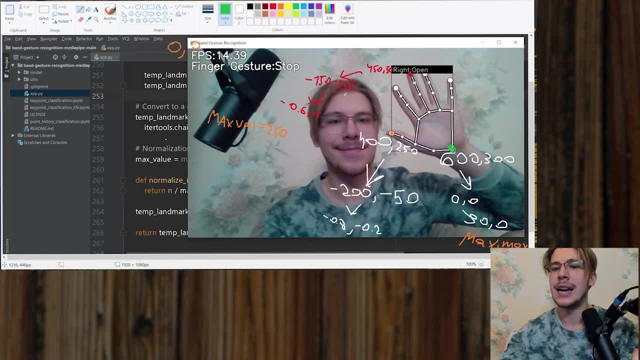 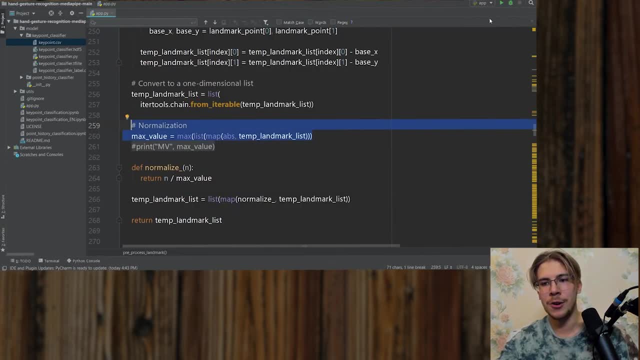 be just just 250, you know, and it'll end up being, in this example, the maximum value. i have it in here kind of like maximum value like 250, like we've identified it in like this line of code. uh, so then what we go ahead and do is: 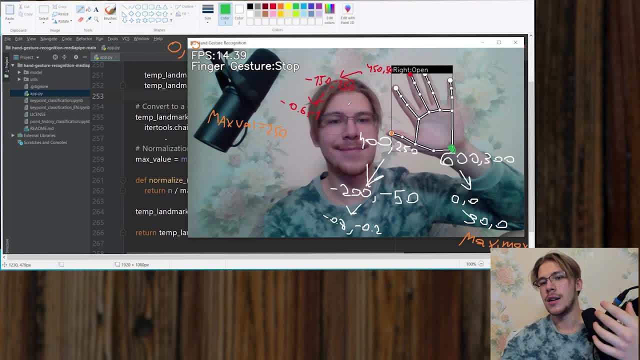 we just go and we divide every single value of this, like distance, pixel values. we divide each of them by the maximum value and we end up with something like this: like this thing will be like: minus 150 divided by 250 will be minus 0.6, and minus 250 divided by minus 250 will be just minus. 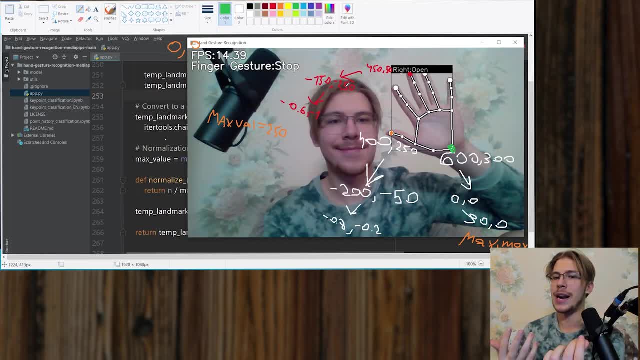 one, aka like the kind of furthest point away uh from from like the our kind of like base point relative to which everything is happening here. um then we divide every single value of this, like distance pixel values, we divide each of them by, and then for this guy it'll be like minus 200 divided by uh 250 will be minus 0.8. and for this, 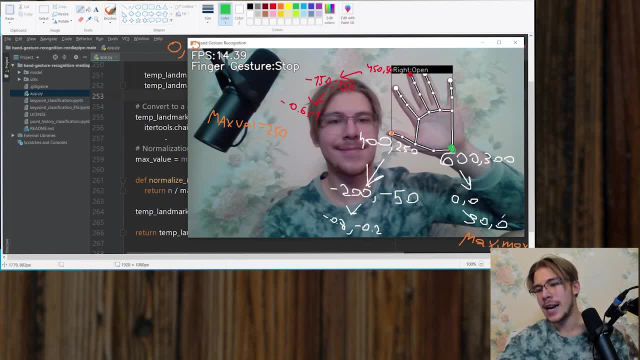 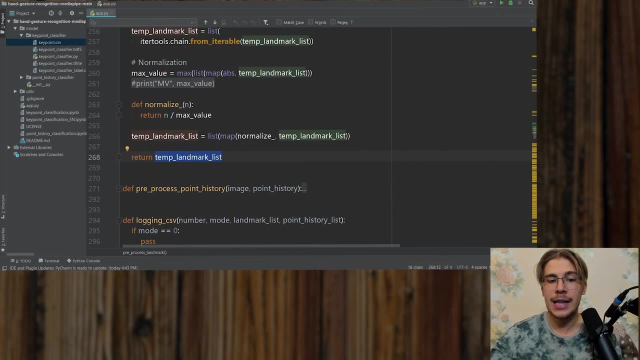 guy will be minus 0.2 and for the base point, as you may have guessed, like you know it'll be, it'll still be zero because, like you know, zero divided by 250 still zero, stuff like that. so that's, that's pretty much what we're ending up with here and that's pretty much what this function returns to. 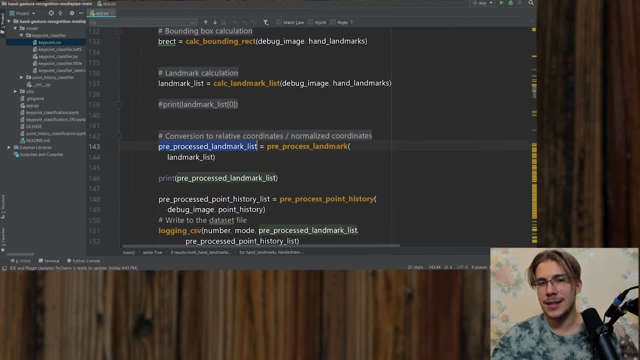 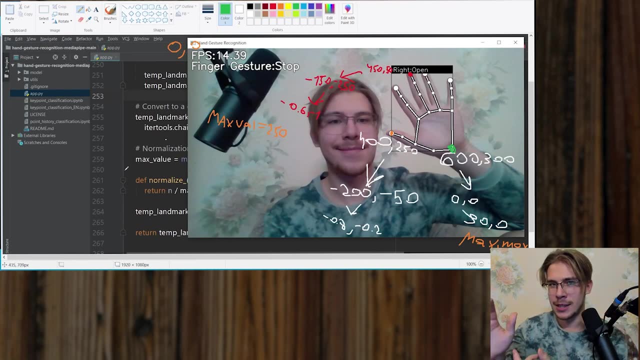 the pre-processed landmarks list, you know, and so, to put into like simpler words, the, the intuition here of the pre-processed landmarks list is that it's normalized values between minus one and one. they're determined by how far away they are from the base point, which is, in our case, like this, like: 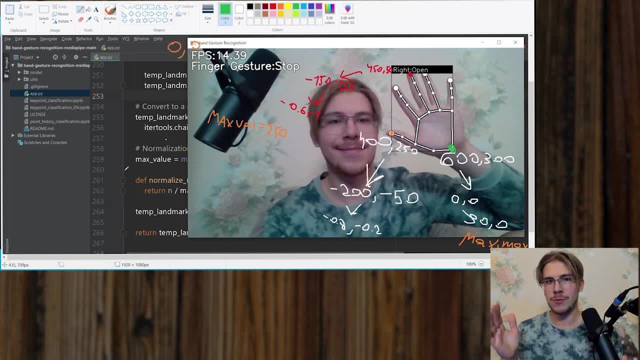 wrist point. you know it's like normalized values between minus one and one, with the values determined by how far away they are from the base point. pretty much it's it's like pretty cool. but it's like it's pretty cool if we've like gotten that, but then we've also like 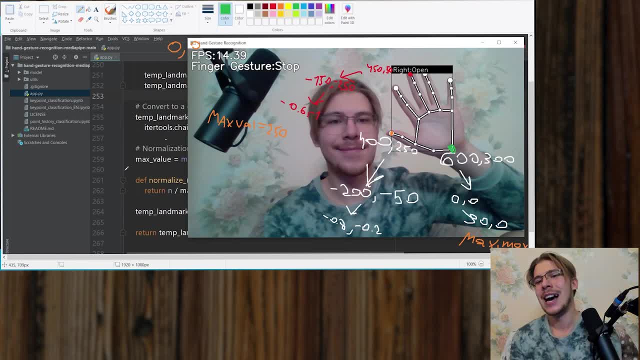 walked through the code, you know, like we see the code, we see like the intuitions. i really, you know, i really tried my best with this drawing, so that's why i'm excited for it, i guess. hopefully, hopefully, it helped with the understanding, you know. and so just like one last thing that i'll 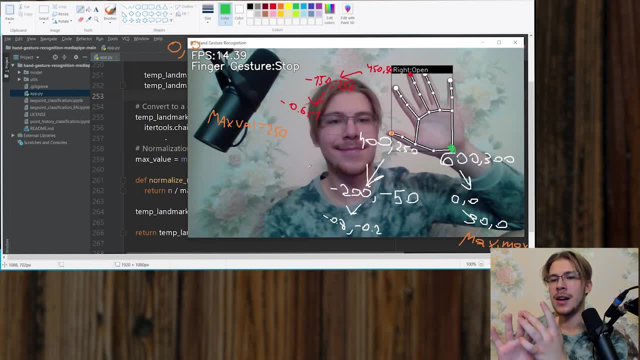 say about the drawing, is that, like in this case, for the middle finger? it's like the middle finger, the um values are like. they're like minus 0.6 and minus one here. uh, if the hand was pointed in the other direction then there would be. then there would just be like 0.6 and just just one, because 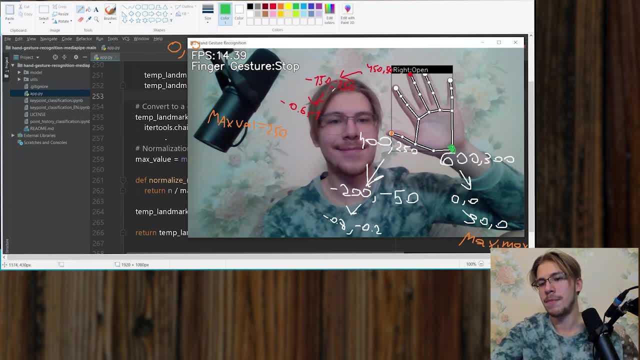 the value here would be. you know, it would be like a positive value now, because it would be like you know, like i don't know, 700 minus 300 or something. so you know, if it would be a flip, it would be like 0.6 and one just. 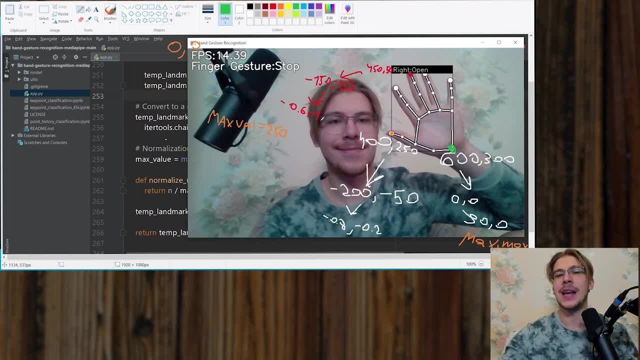 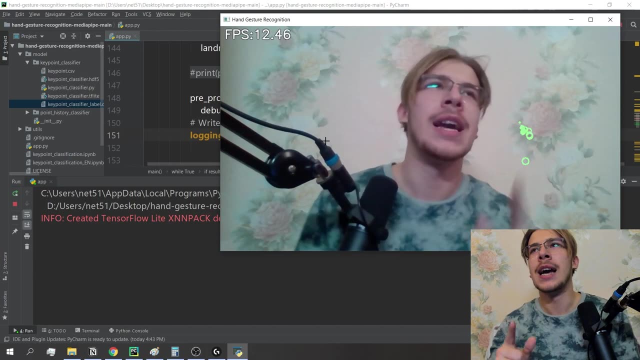 just another cool observation, okay, cool, cool, cool. now, after we've like talked about all this, we're actually like this close, we pretty much know all we need to like start training and stuff like that, you know. so one quick thing before we jump into training, just like actually really quick thing. 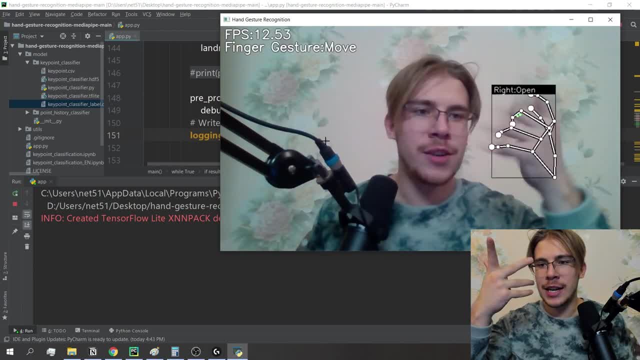 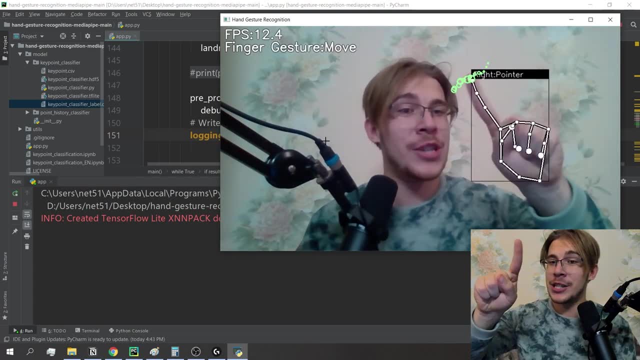 it's like, as i was saying, this report deals with like two things, which is hand gesture recognition, but also, uh, point history recognition. so, for instance, when it identifies that you're showing like a pointer gesture, it started drawing in the circles, like recognizing like i'm rotating counterclockwise or that i'm moving, or 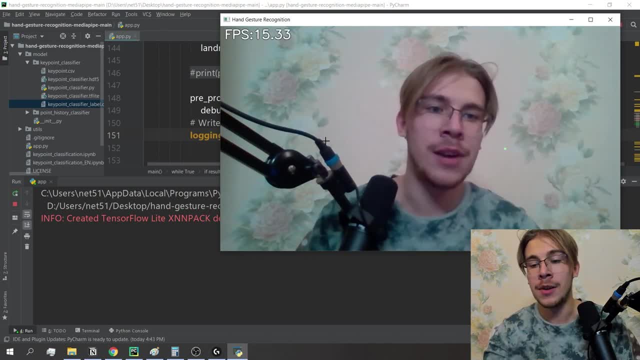 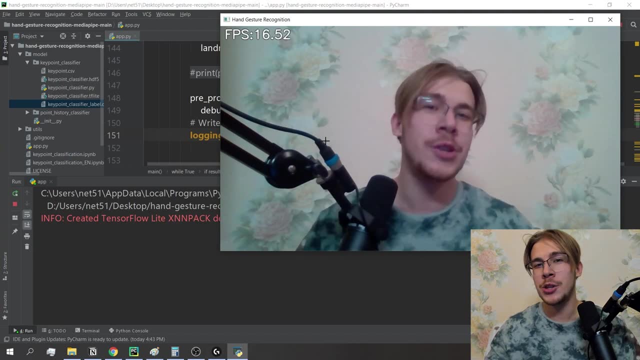 whatever it is that it's like recognizing right now. um, this is like awesome. maybe i'll make sound like that in the future, but like that's kind of beyond the scope of this video, so i just wanted to like really quickly show you how you can disable it, so the way it works, as i was saying, 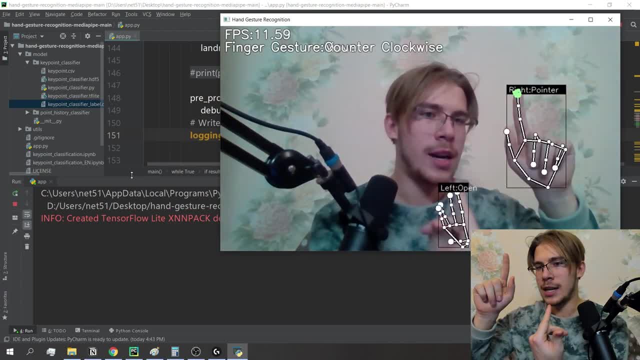 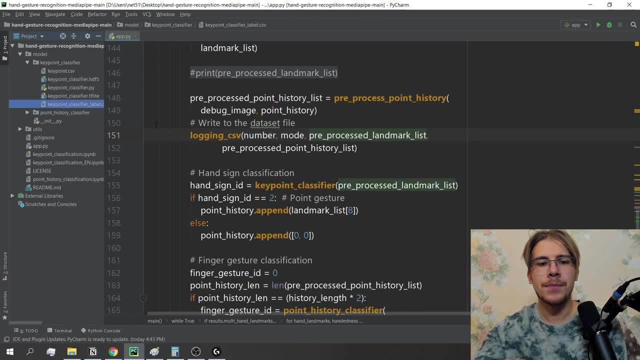 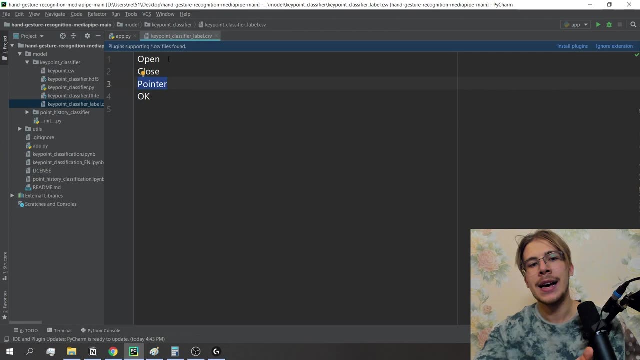 is that if, when the hand gesture recognizer identifies it as the pointer sign it invokes, like all of this, like point history functionality, um, we can go into the labels file, which we'll talk about in more detail very soon, and see that the zero one, two, that the pointer pointer index has, like the pointer kind of the label pointer, has the index. 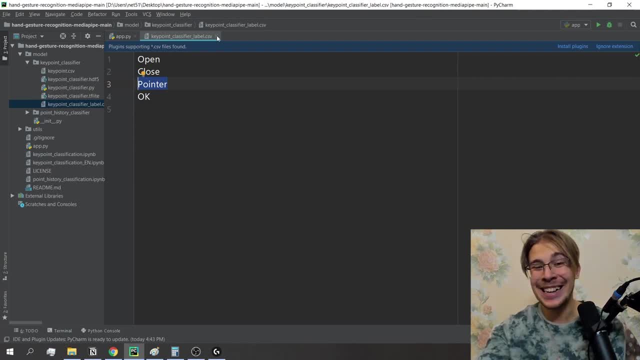 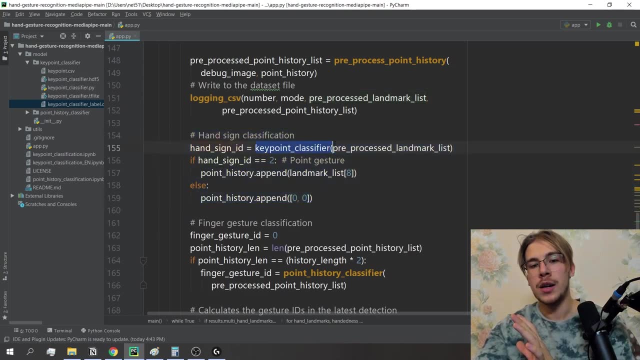 of two, which means that, like in the neural net, it also has has the second index and with that we can go here and check. yeah, it seems correct. like whenever, um, our uh key point classifier gives us and it equals to two, it invokes this like point history stuff. so, like the little you know not. 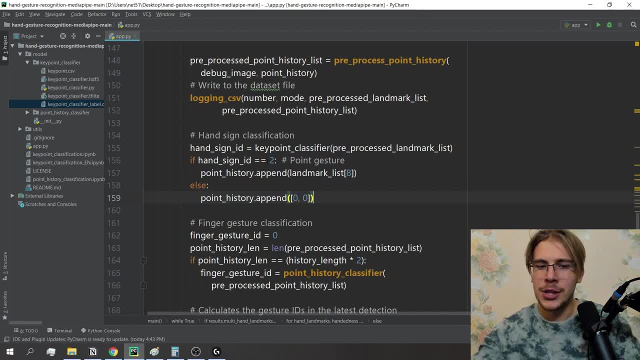 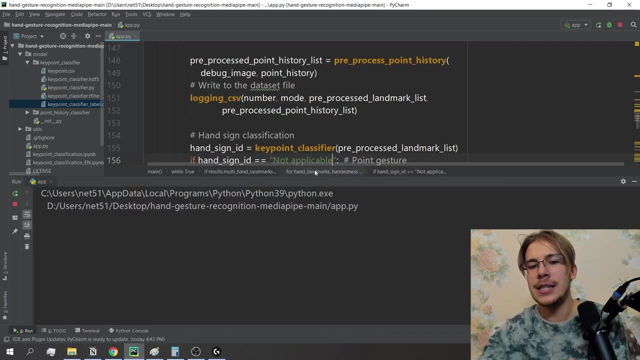 super fancy but like reliable way to disable is to just change it from like. if hand sign id equals from two to like sound like not applicable or something like that. you know, obviously a hand sign id which is like a number will never be that you know a string not applicable, so thus it'll. 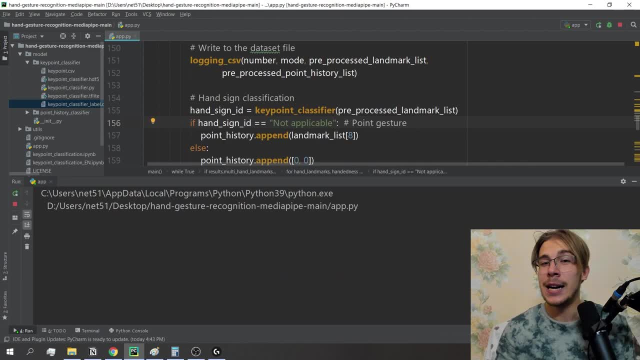 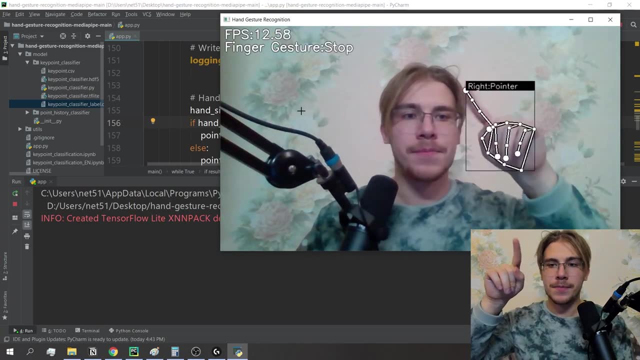 never really involve this like point history thing unless you know you want it in the future. in this case, you can like bring it back and uh. so, as you can see, like it's like disabled now nothing in terms of like point history and stuff like that, but in 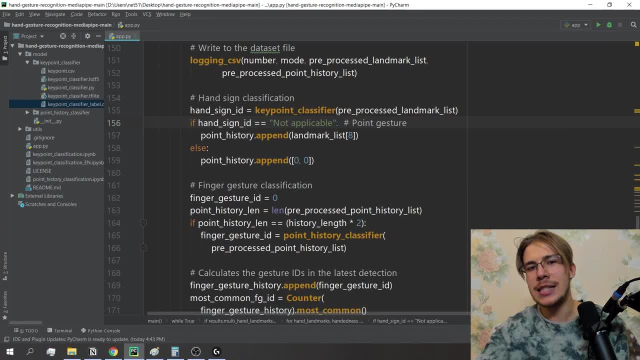 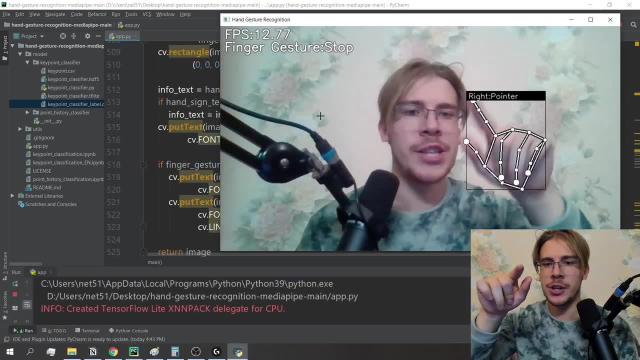 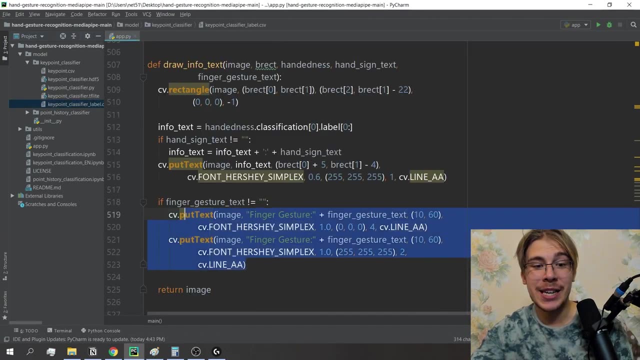 the future. you want to like work with it. you can like maybe train like a custom gesture and i don't know like put in the index of that here. and if you also don't want the like finger gesture writing right here to be displayed, you can just like go into the um, draw info text function and just like. 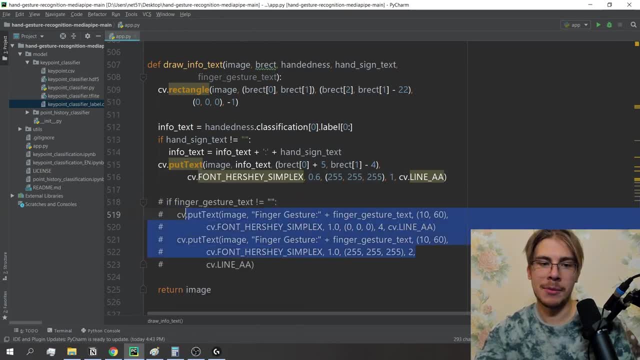 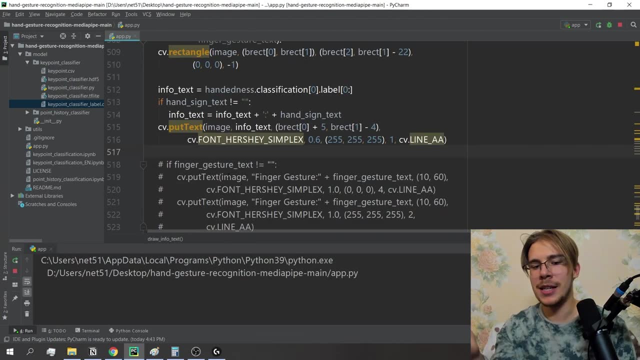 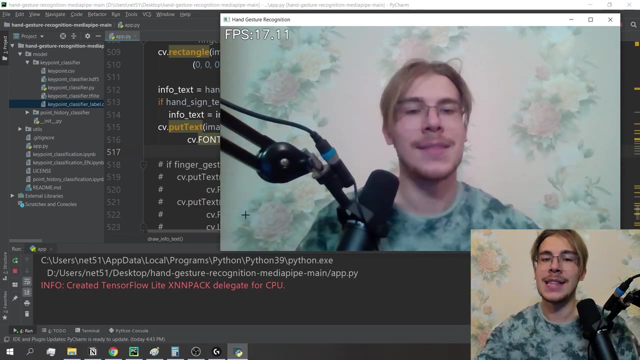 come on, this little guy out. i did that by pressing like control and slash in pycharm to do that, but it's not super annoying, but like, maybe if you're building like a specific application, you really don't want to include that stuff. so, uh, there it is gone, you know. now on to training for real. this: 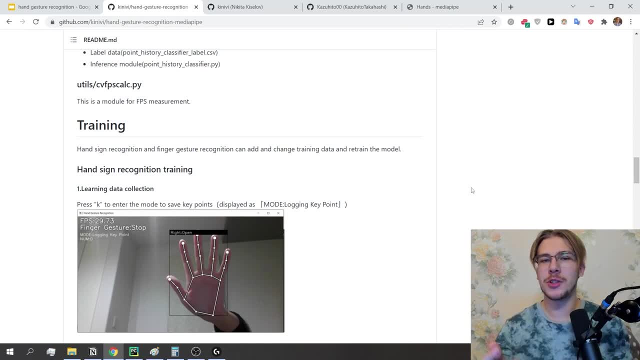 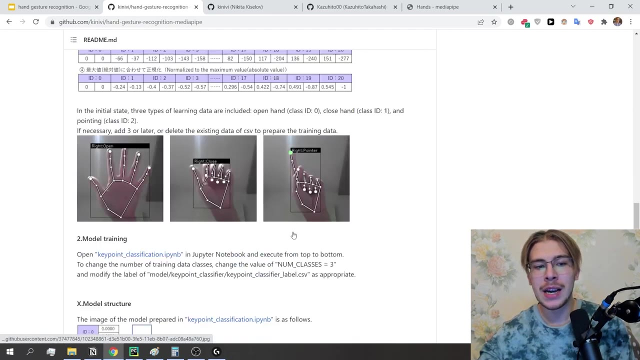 time for real. so now let's finally talk about training and how we can train, uh, the model and within, like this pipeline of systems to recognize our own, like custom hand gestures. in the repo we can see that there's like there are instructions that you know we'll be following to perform the 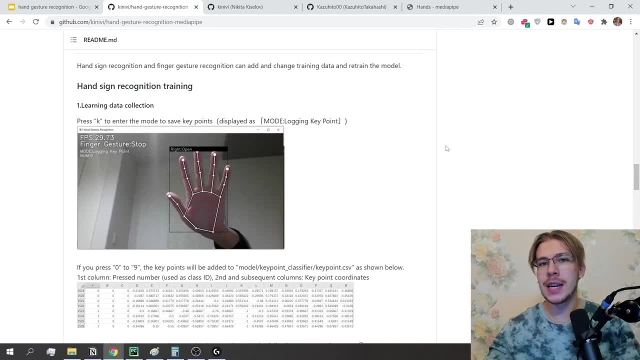 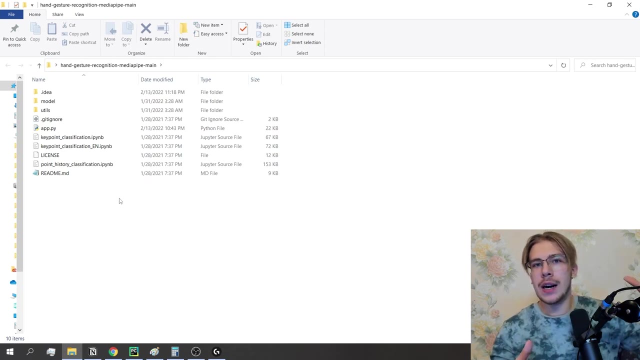 training successfully. but i suggest we talk about training in the context of three main things, which is, uh, preparing a data set, training a model and then testing. so let's dive into it. so first kind of interesting thing to understand here is like how the author of the repo 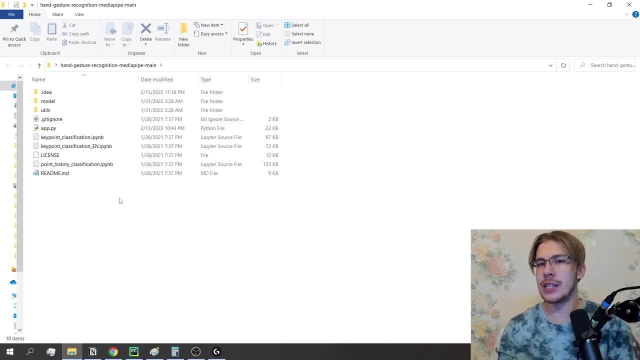 handles the data set collection and, like just in general, storing of the data set. so, uh, for the key point. we're interested here in the key point classification in particular. uh, same thing as like hand landmarks classification. on top of that, you know like kind of the thing is, we train on top. 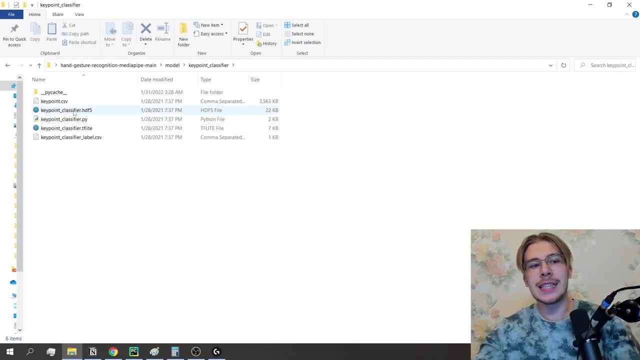 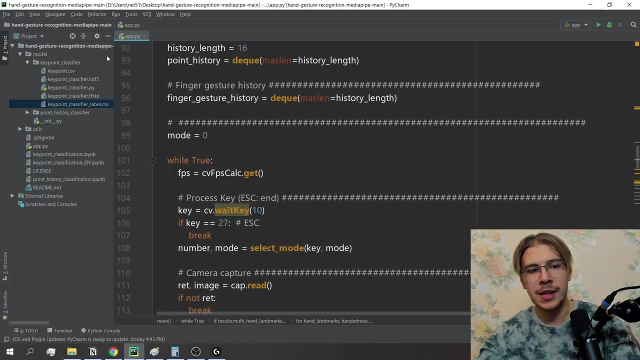 of hand landmarks, pretty much so. the training data is stored as a cc file right here and i'm opening here, like inside a folder, so that, like in case you're not using pycharm and you don't have the same layout that you also know like where to kind of find, uh, those, those files, but i can actually open and view them in pycharm. 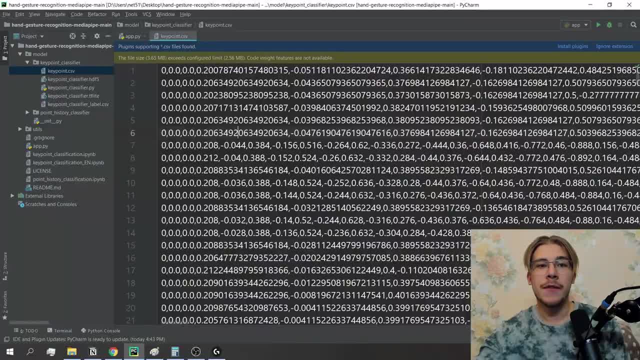 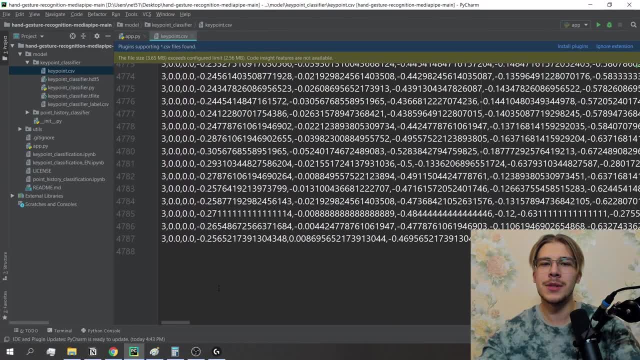 like this, and here you can see the keypointcsv file, which contains like the training data that, oh, at this point, is what the author has collected. that's kind of what the repo comes along with, and the labels. so here we can learn that the first column here is a class index. so, for instance, 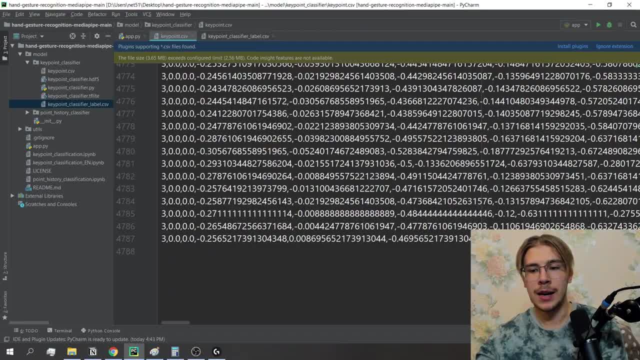 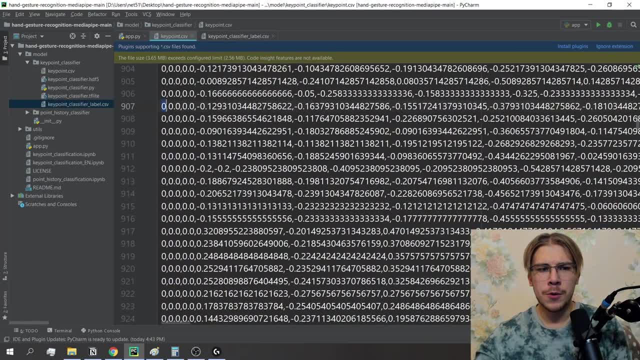 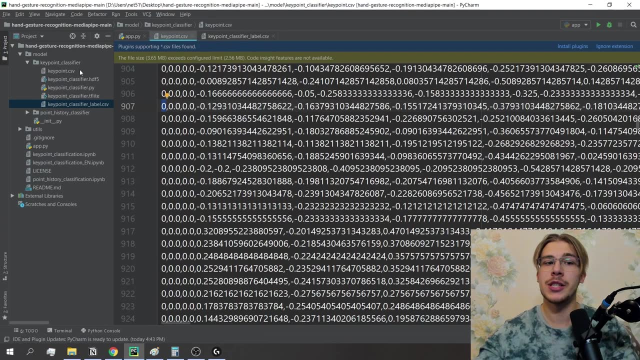 the class of this is: these things are like three um. here's like two. the class index here's like one um, here's like zero and etc. etc. etc. here's just like four classes that it comes along with. but you know, we'll start creating them in. 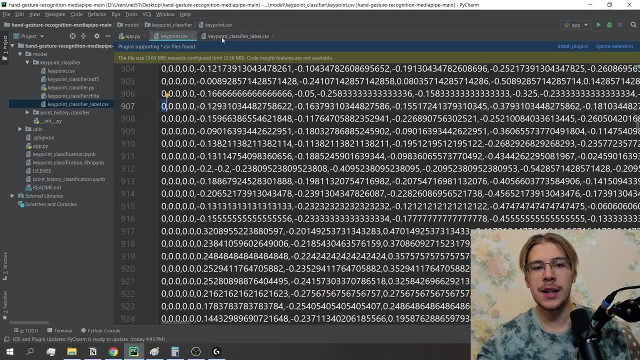 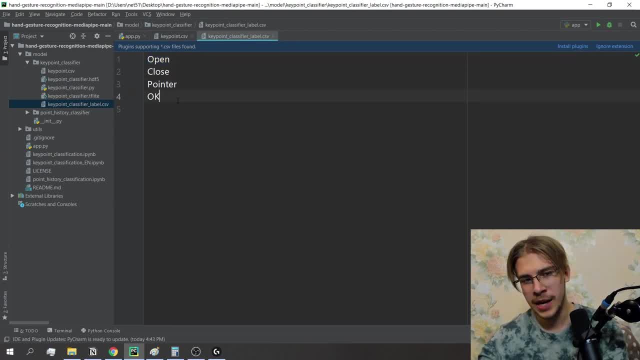 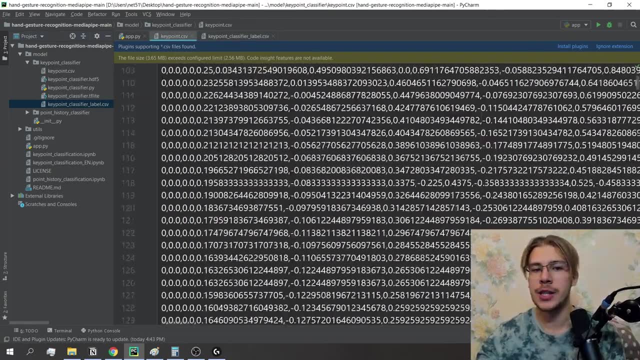 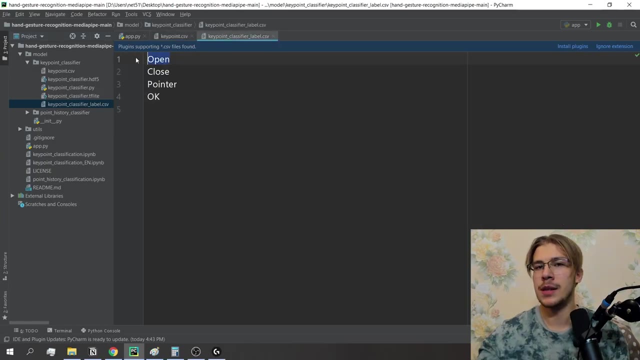 just a few moments. the thing about classes is that they're matched by a label file where, for example, the class with the index zero. so they go like zero, one, two, three, uh, so pretty much all of these guys are with like the zero, as the first column are the landmarks for the class named open. it's like 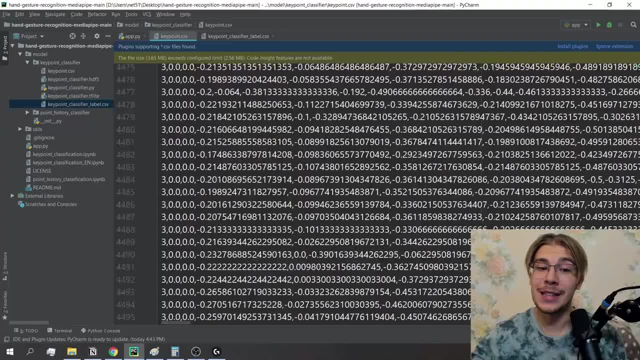 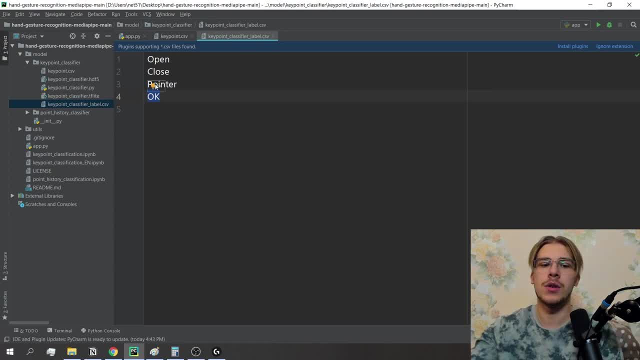 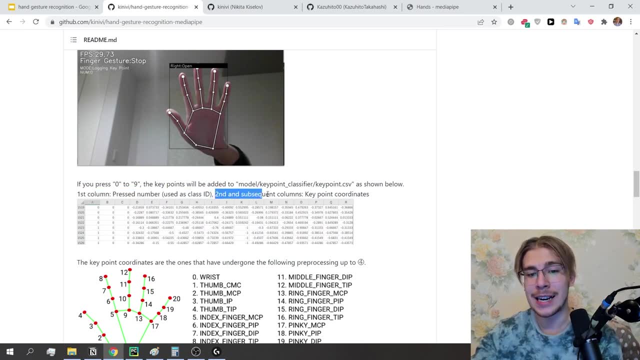 open palm in this case, and all of them, for instance, with the index three. here are the landmarks for the class within, for the class. okay, pretty much so. uh, as you can see here, like the author says, like you know, pretty much, first, column press numbers is like uses a class id, and second subsequent columns: 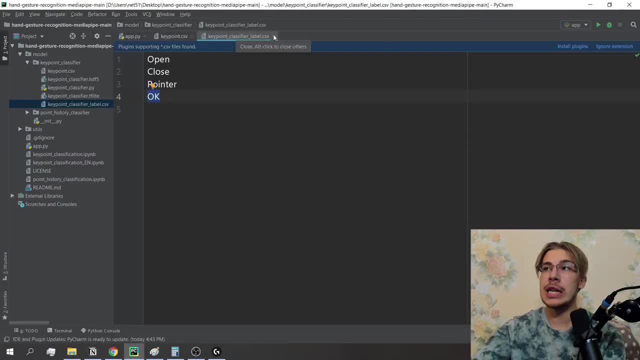 and coordinates. now, how do we actually, uh, collect kind of like new training data in this way? so that's, that's a great question. let's, let's, let's, dive into that too. so let's first, as an example, say that i want to keep this for classes. i just want to add like one new class to them, so for. 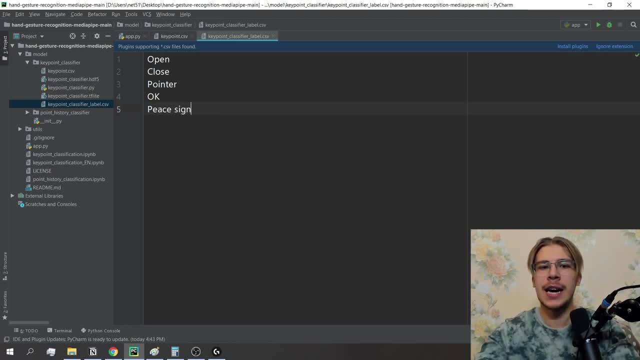 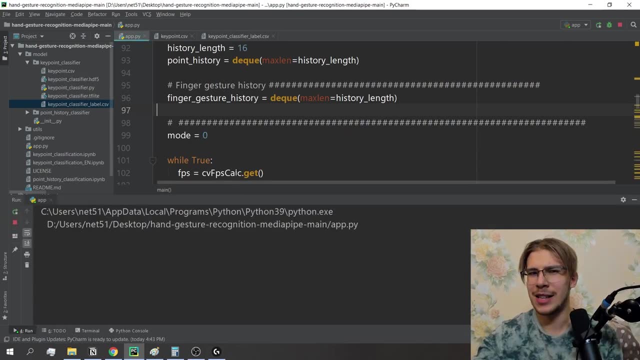 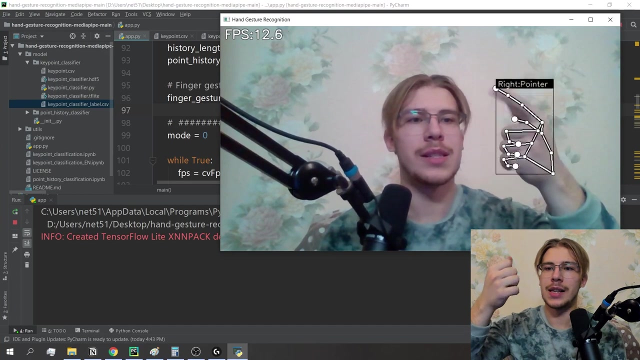 instance, i want to add the peace sign. so i'll say here: peace sign in the labels file. and right now, when i launch this thing, like you know, obviously we haven't done any training, haven't collected any data, so like there isn't gonna be a peace sign, uh, you know. so you know it's like, but it's. 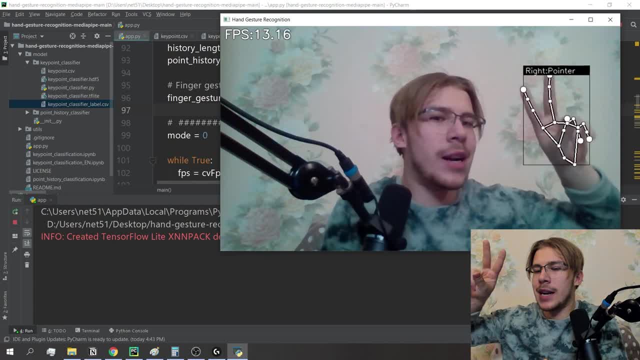 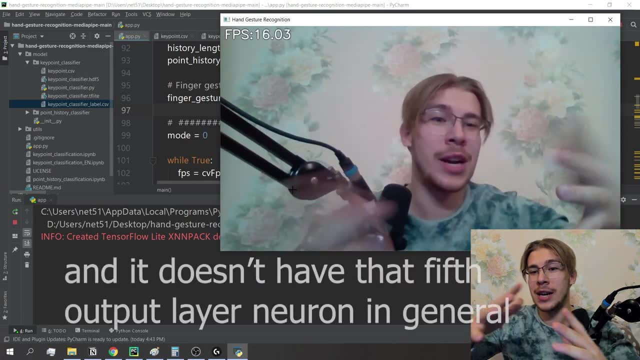 also not gonna give us an error because, like, it's just simply never gonna guess the class index four, which should be the peace sign, but it's just neural network never gonna go there because it wasn't trained on that data. but we can actually start training it and start collecting a few. 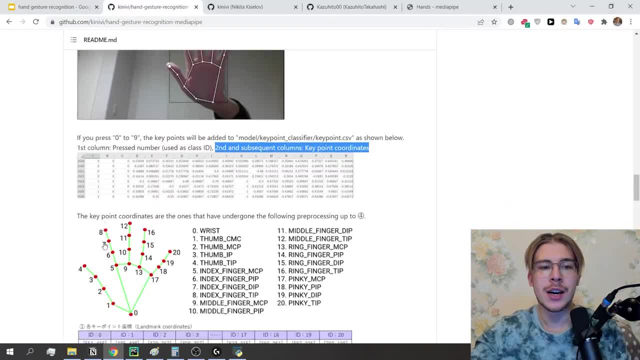 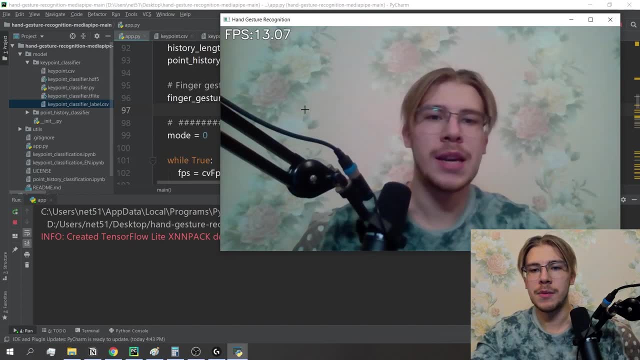 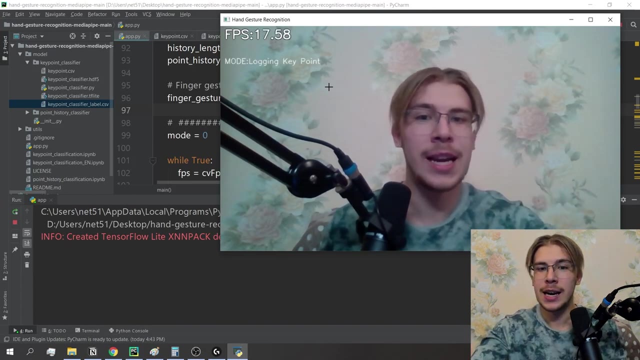 samples of what the peace sign looks like. let's check it out here. uh, it says that. here it says we press k to enter the mode to save key points, which means that, like we press k inside the openc window, so i kind of click here, my uh keyboard is like in the english language and i press k. 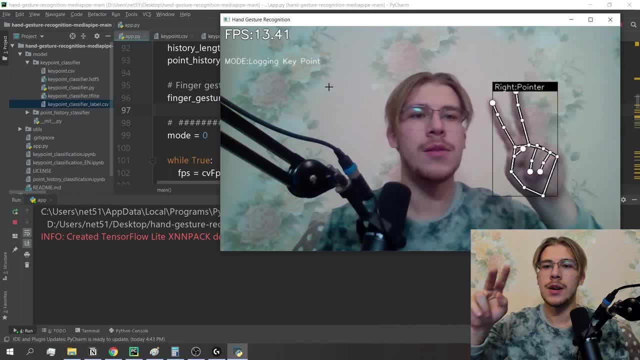 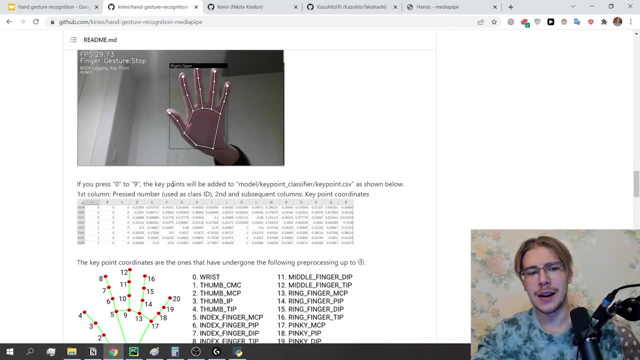 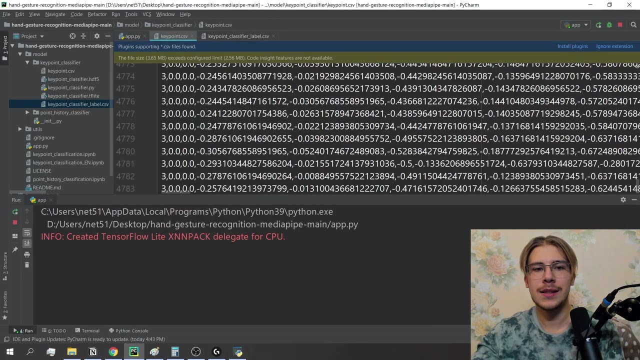 and it says mode logging key point. so now, uh, when we're in this mode logging key point, you know we can press from zero to nine and it'll kind of add: uh, the classes with this index of the number that we press will be added to this like data set that we have here. so let's say that we have a key point. 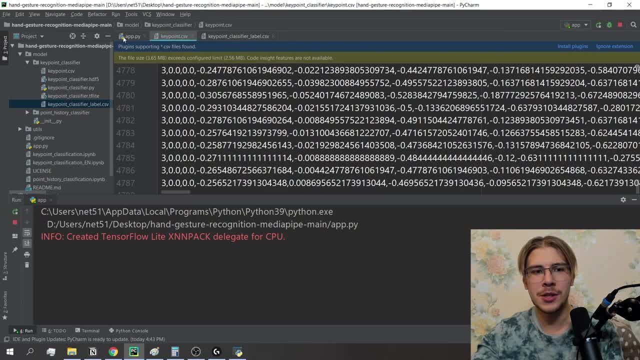 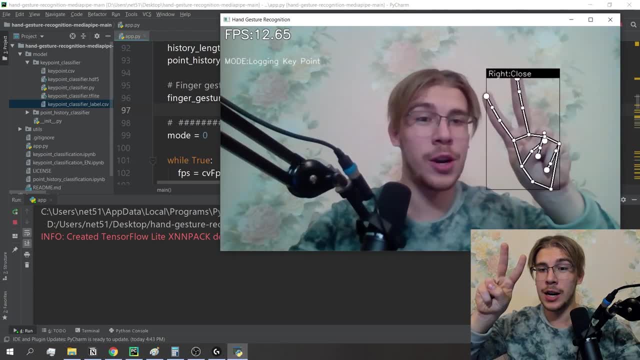 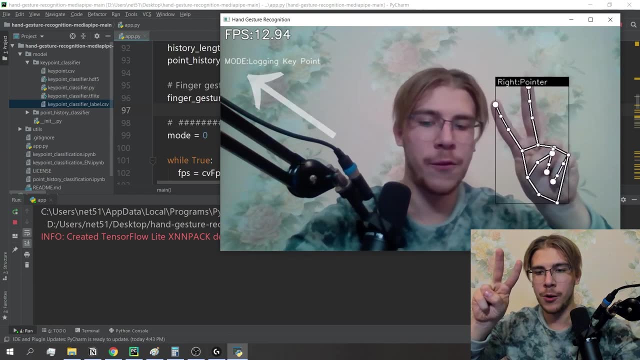 here. um, i'll, i'll, i'll show you right now. so, for example, i'll go and i'll say peace sign, and it's gonna be a class with the index four. and what i'm doing right now is like i'll literally start clicking the key four on my keyboard and be like four, four, four, four, four. and as i'm clicking it, 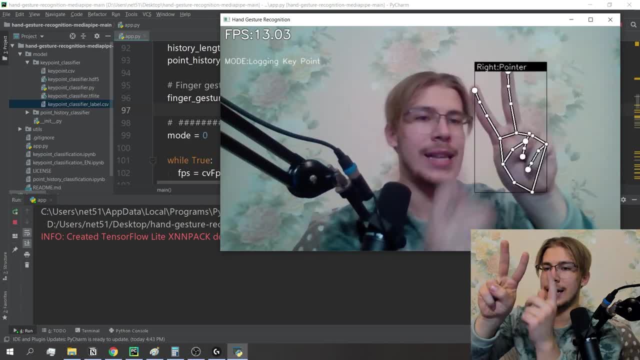 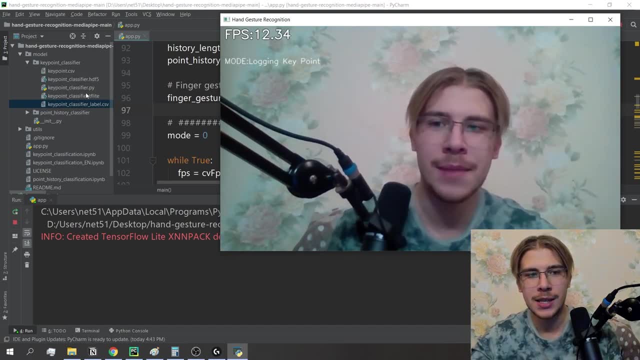 it's taking like a snapshot of the image, uh, and like it's. it's like saving this. you know this. key points under the label four, so i've clicked it a few times. i can go here. key point at csv, as you can see here a few new. 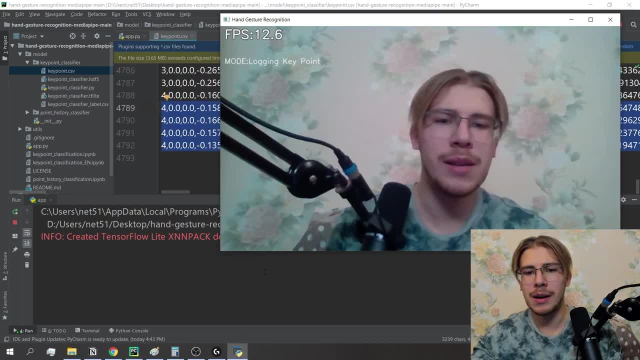 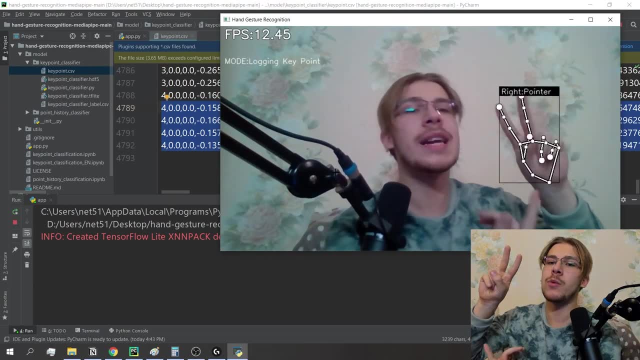 classes appeared with the index four. now, uh, i wanna, i wanna add like more like that's. you know, i think you know probably want to get like. you want to get way less than you would have have to get, where you're just like doing the pixels first approach, but you still want to get like. 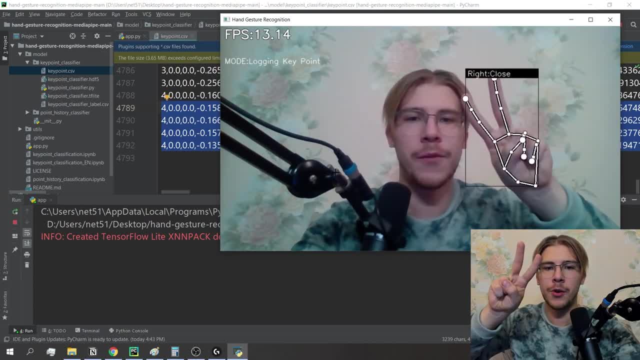 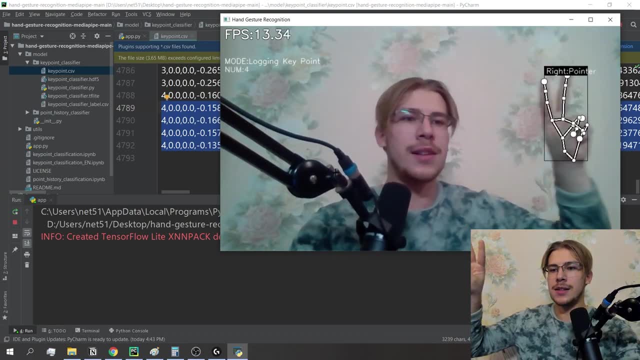 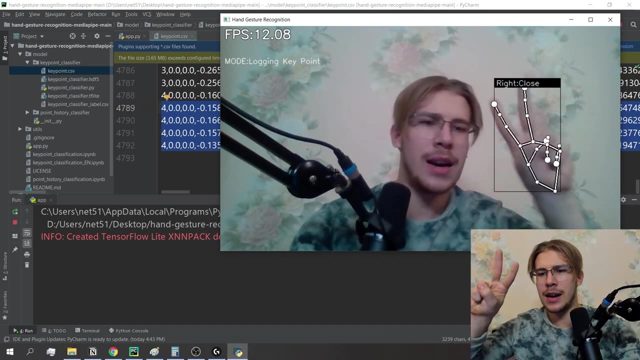 maybe i don't know, 20 or 30 or something like that. so i'll go and be like four, four, four, four four. maybe i'll still try kind of a bit bit of them like different scales, even though it's not again as sensitive to that, because we've like normalized that stuff. still i think useful some, uh, some like rotations. 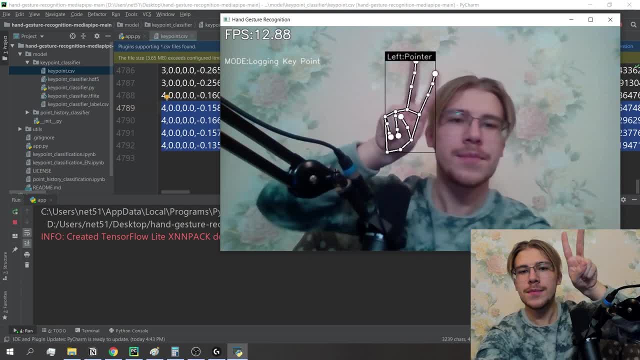 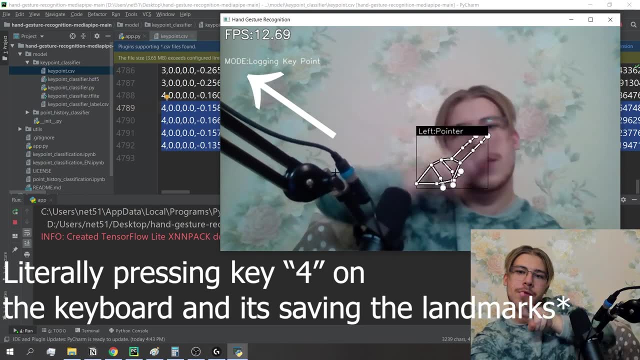 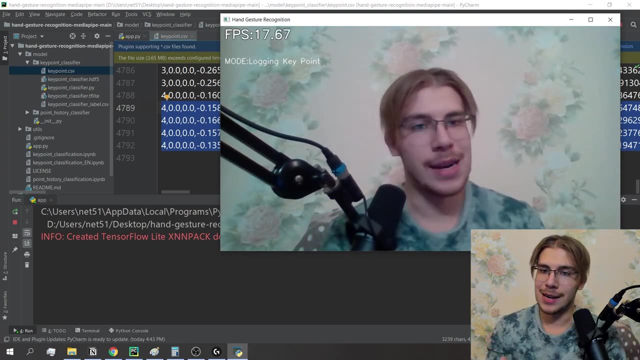 and stuff can be useful too. then i'll go and i'll do them on a different hand: four, four, four, four, four again. the cool thing here is that, like the background doesn't matter, uh, the again, the, the, any like specifics of what fingers are doesn't matter, like you know. so like if you train. 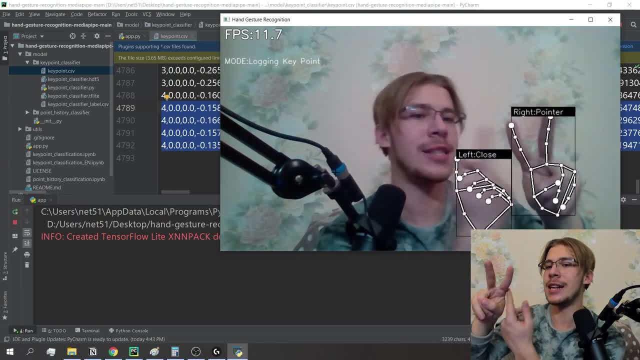 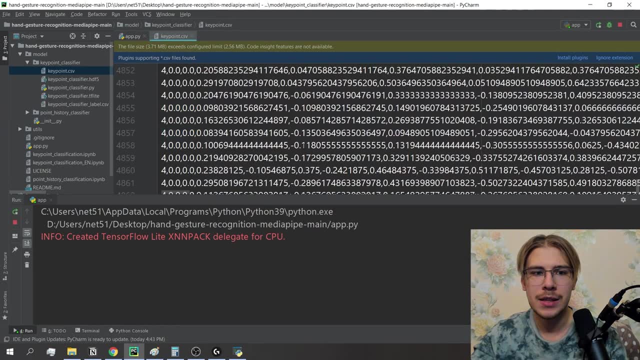 these things like her, my zp sand in your hand, chances are like on somebody else's hand with this, like landmarks, it's also gonna be recognized. but yeah, let's say we've collected. let me update the yeah, this guy. so you know it's not a lot but it might do the job. let me add in a few more. 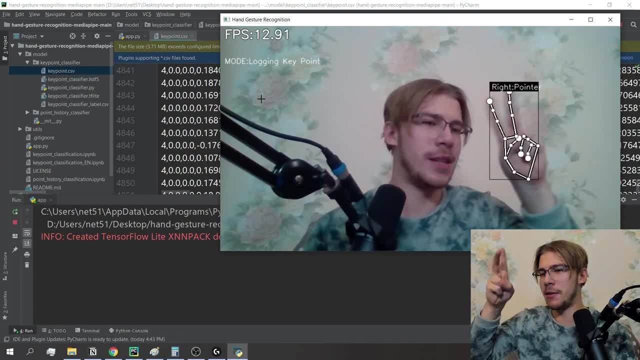 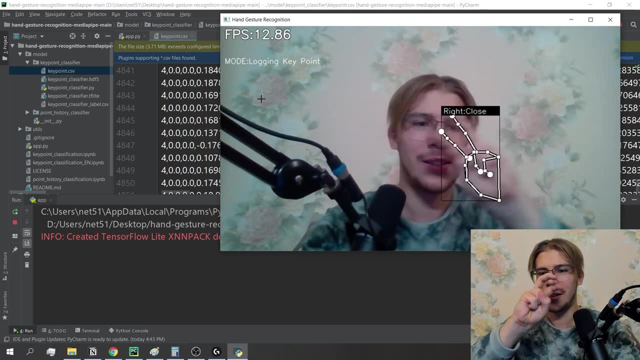 just, maybe i want to like. maybe i want to like squish my fingers- if you know that like scales isn't the biggest deal here, because it's really maybe i want to like try some of them, like you know, like a little more. you know i'm gonna squished fingers. peace signs. 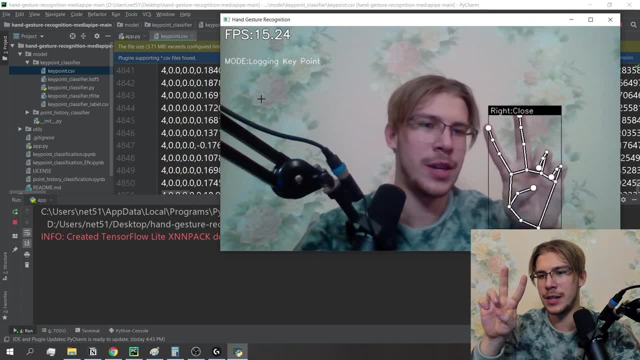 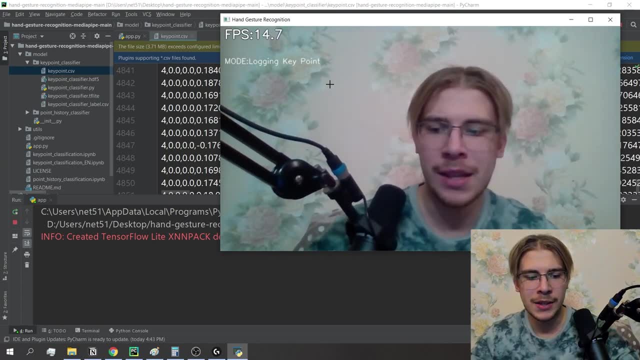 or something like that. maybe, like these fingers can be a bit differently orientated like this. like depends on how much i want to like go with it really, but yeah, let's see if connecting enough data, i'll press escape to like exit this window. now the training was. that was like the first step. 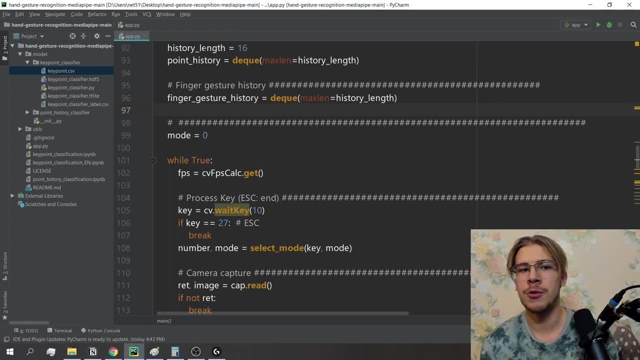 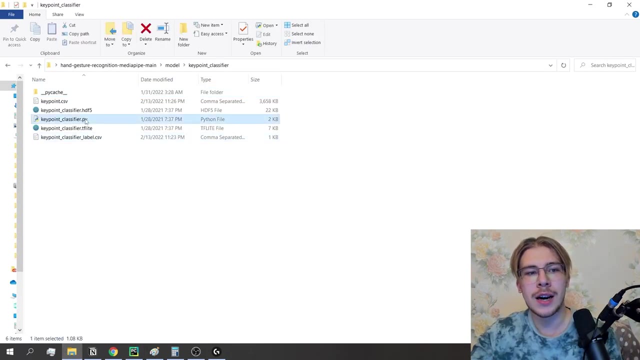 the second step. it's gonna be really easy. thanks again to the author of the repo. the training is gonna be like so like we'll be able to do it like literally without even thinking about it, but we'll still kind of look at the code. so for training, there's this um, there is this jupiter notebook. 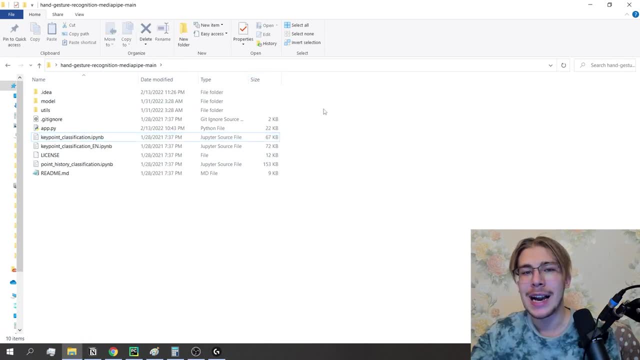 for training on a key point classification that we, we can run, and if we run, like all cells in the jupiter notebook, though pretty much you know, do the training for us. yeah, so what i'll do is i'll open the console in this folder and i'll say: 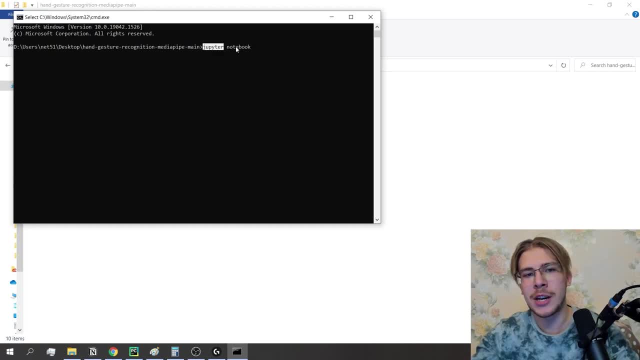 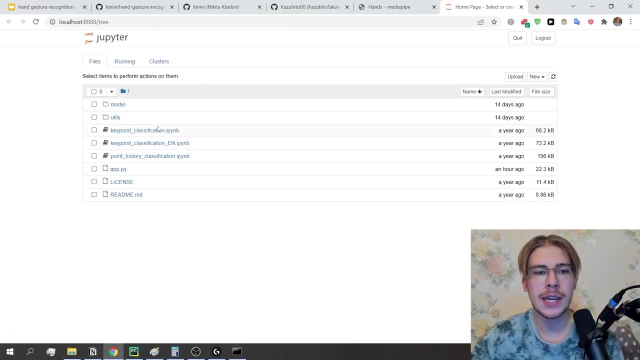 jupiter notebook. jupiter, in this case, like, is a python module that i've installed, which you can people install, jupiter, and you'll. you'll be able to open it too, and here i'll open the key point classification that ipy and be pretty much the the jupiter notebook. so a few things. 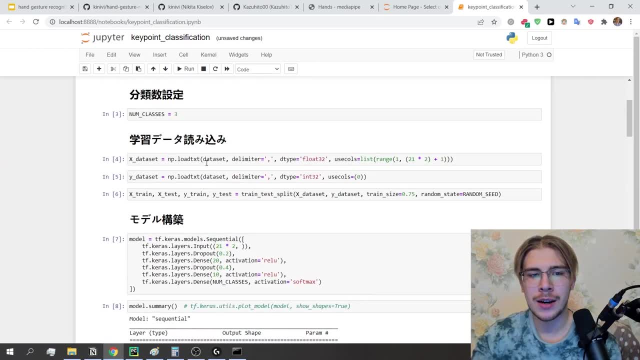 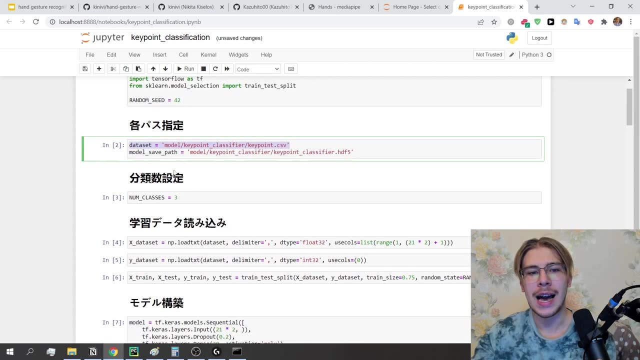 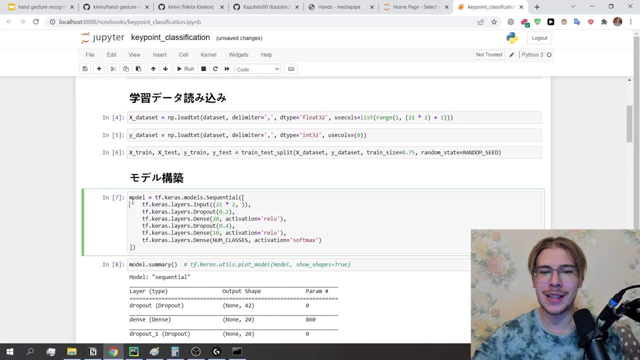 that we want to note here is that essentially the um. what this thing is doing is that it's um, loading the data from the that csv file and, uh, it's defining a model which, like. so, as you can see, it's a very simple, like curious, neural network architecture here with um. you know this many like. 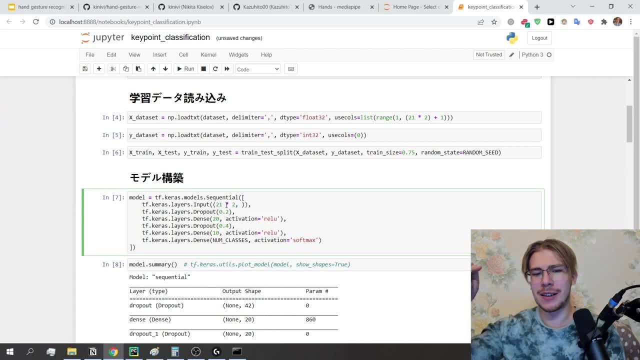 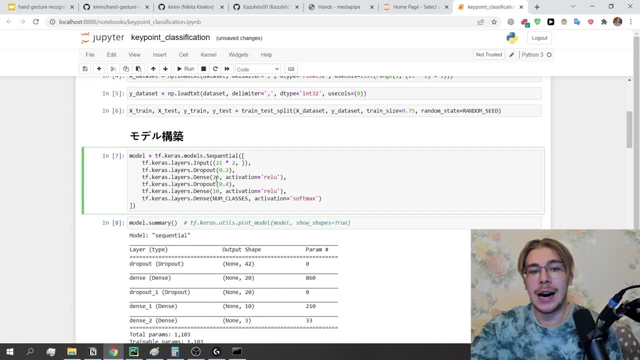 with like 21 times two input neurons, which is gonna be like a vector of values for for like this, like landmarks, pretty much, that are pre-processed here: um, followed by followed by some dropout 20 dense neurons, some more dropout, some more dense neurons. a very simple architecture and with the output layer having the 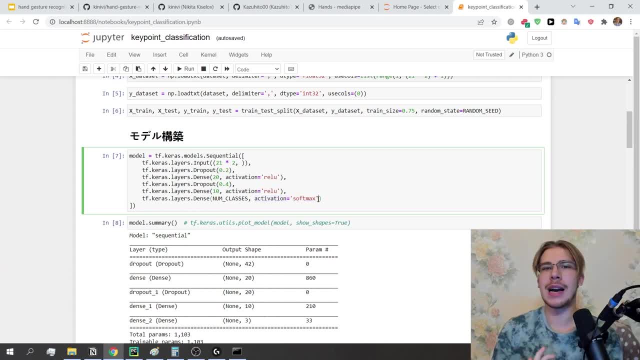 um softmax activation function. because you can have, because a hand gesture can be both like a p-standard and a k-standard at the same time, which is what this guy is useful for. and the num classes is determined by you know like how many classes we have in our data set. you know, in our case we 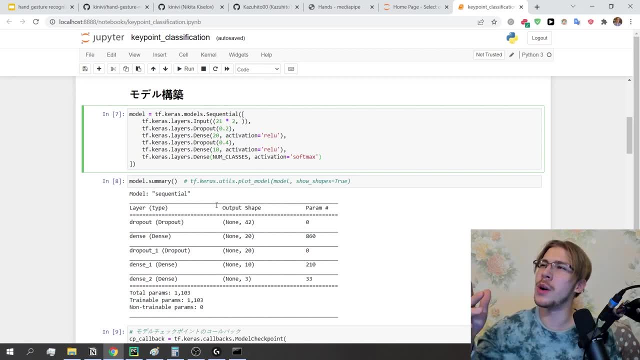 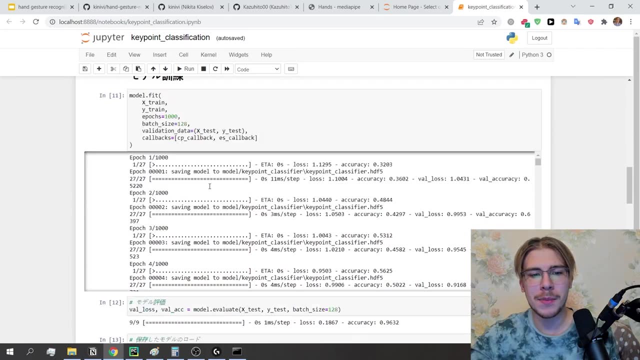 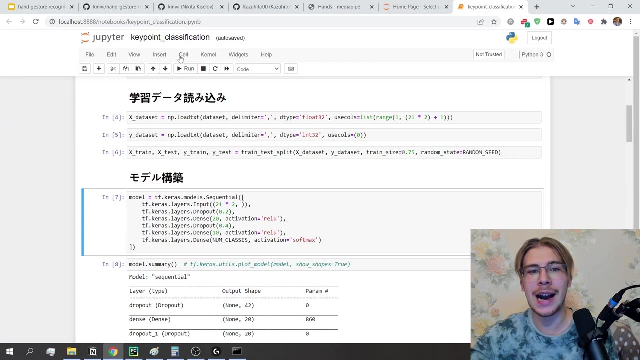 have. we'll have four by this point or no. i think we'll have five. right, it'll be like open four, close pointer, and okay, um, and then i pretty much just like, save, this transit model saves it. the whole training happens like really, really quickly. so pretty much i, what you can do here is just like: 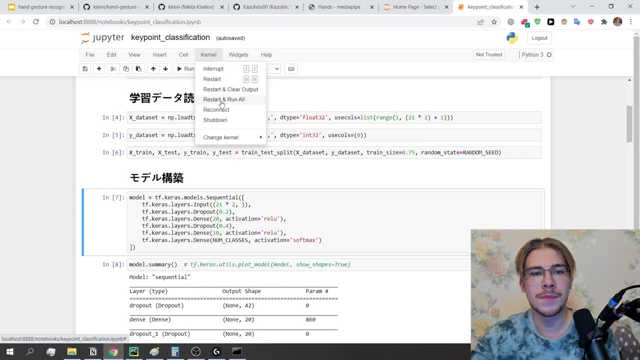 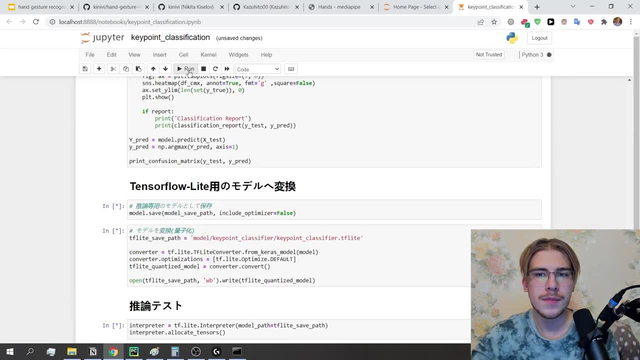 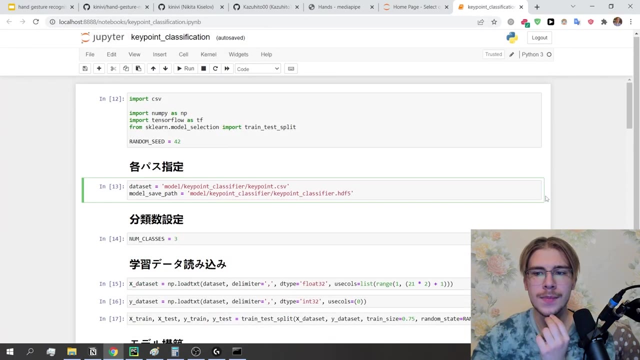 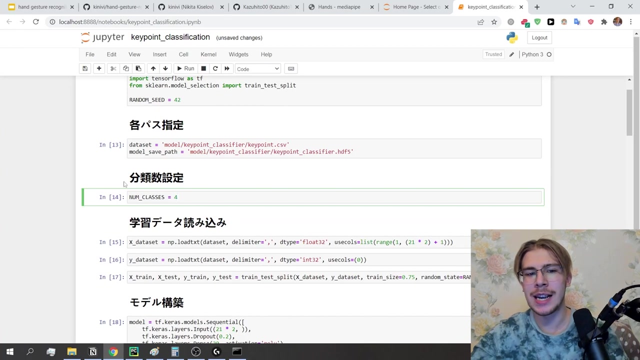 go and be like kernel, um restart and run all. it'll just like run all cells. okay, i see what's it saying. uh, i forgot to modify this variable here: number of classes, as i was saying. now we have, now we have um five classes, so it'll be, it'll be five and now go sell, run all. 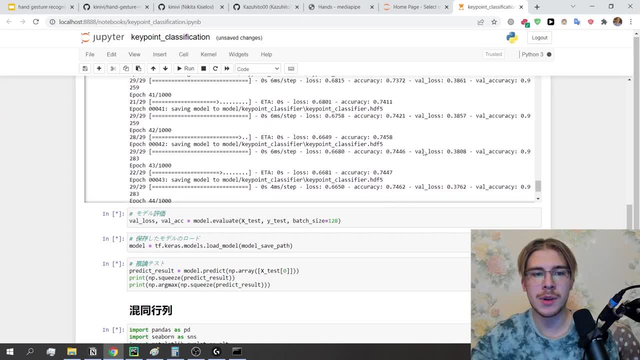 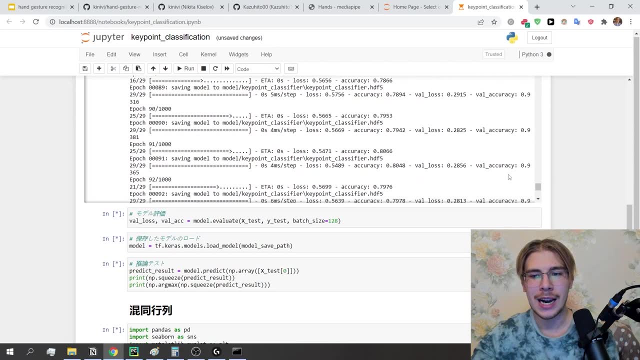 so you can see it's training and it's training like really, really quickly. it looks like you know it says here that it's gonna change for 1000 epochs. in reality it's gonna do like early, stopping anytime soon. but, as you can see, like the whole training process is like really, really quick in. 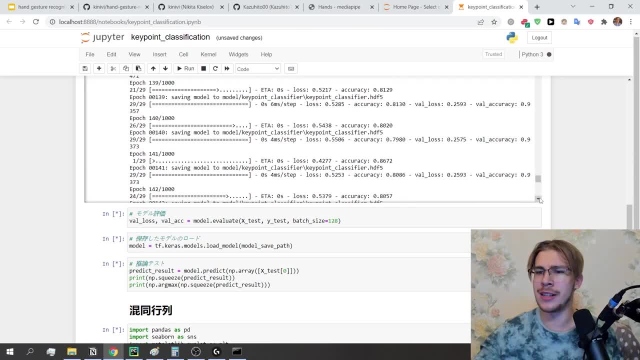 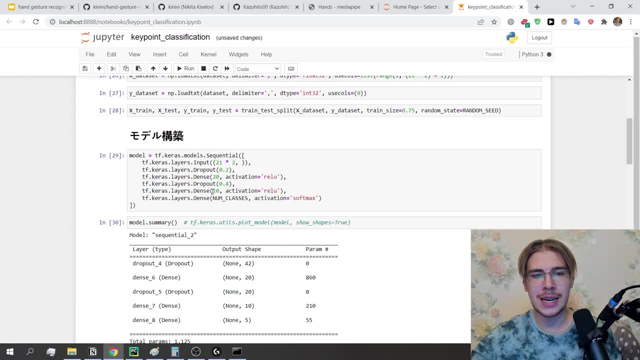 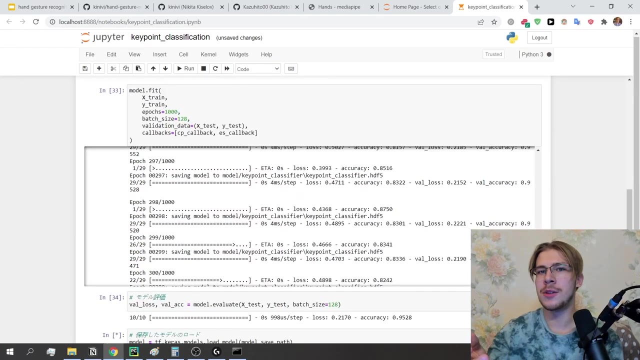 this case, and it's not gonna get much longer, honestly, because, again, the whole neural network architecture here is, like you know, 20 neurons, followed by 10 neurons, followed by, in our case, five neurons here. a really small architecture, but what's it doing right now is it's learning to map. 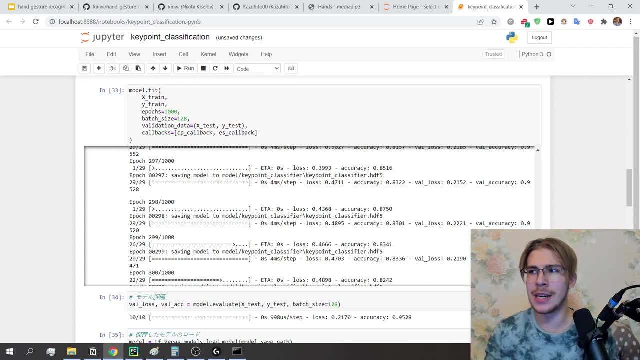 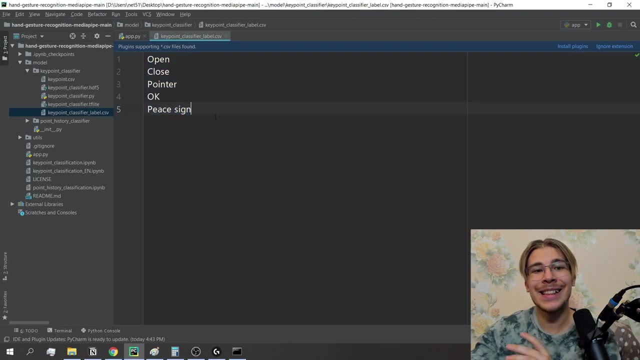 like the input vector and that input vector being the uh hand landmarks for all sorts of different to, to, to like its label, class, right. so it's like learning to map this like relative landmarks, to to a number, to like an index, and that index represents according to like that index, like 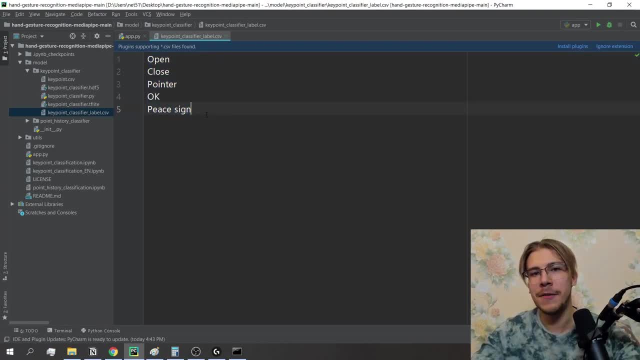 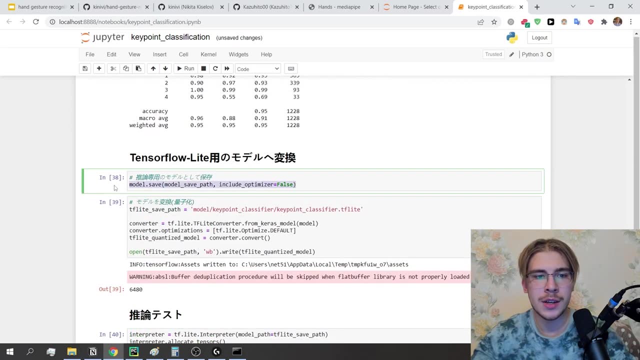 we make it say that it like corresponds to this, like label file. you know what i mean? um, so now, now that it's finished training, it'll save the model automatically. it'll save it here with the model save path, and so pretty much, yeah, all you do is, like you say, sell, run all, run, all the. 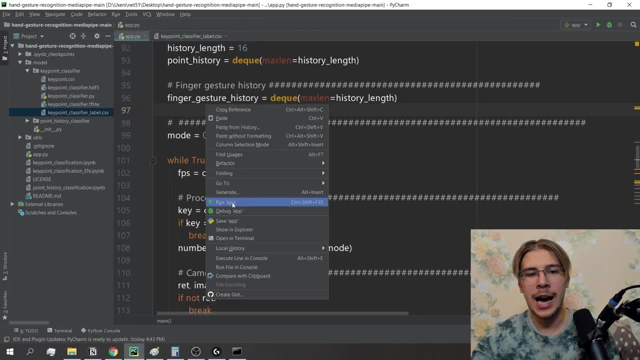 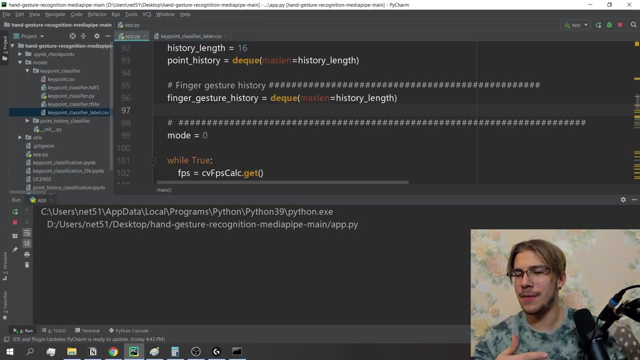 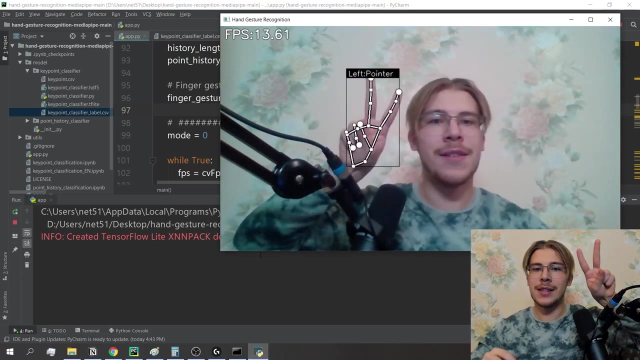 it finishes running, then you can go and you're gonna like click up and, uh, if your label file is all right and if, like you're, if, if everything went smoothly there, then you should be able to start recognizing a new hand gesture, so like peace sign. there you have it: peace sign, peace sign. 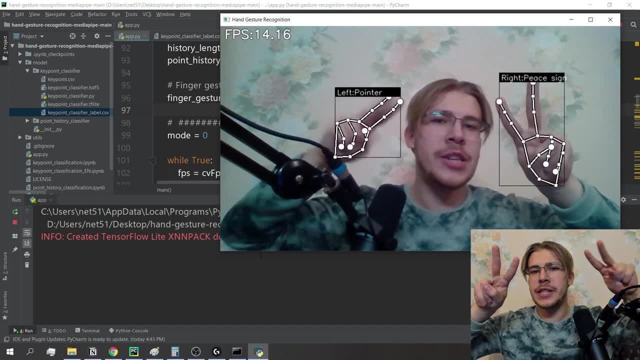 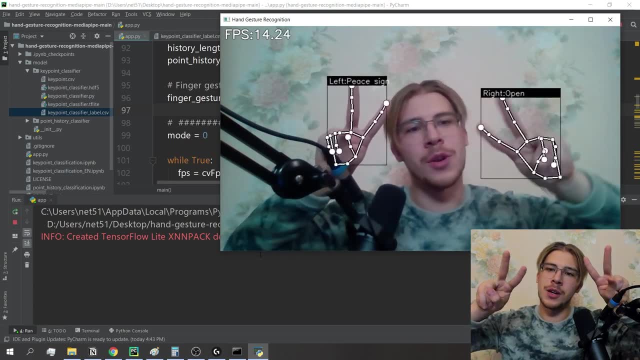 it thinks that this thing is a pointer which, when i see this, it's just a signal to me to like: add more data and i'll not think that anymore. potentially it'll also that kind of looks a bit more reliable. i don't know with this guy, uh. but as you can see, 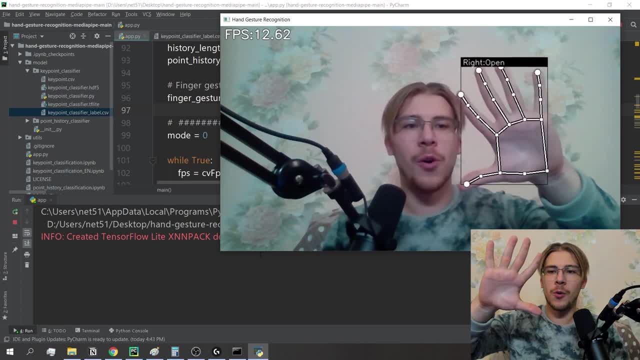 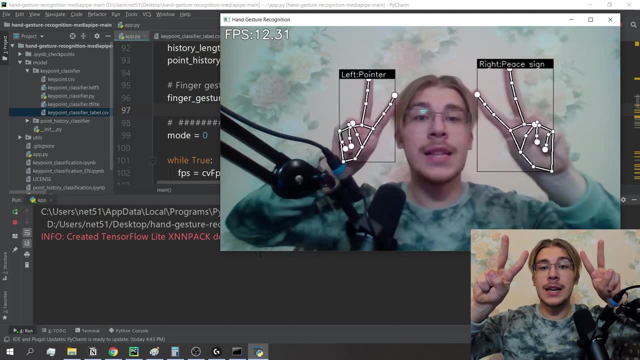 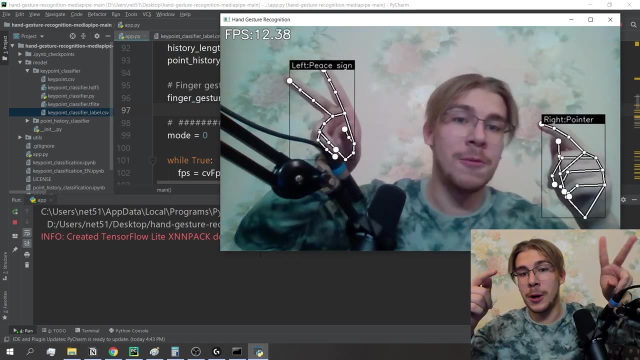 now it's, you know, we can have still the okay sign, the open, uh, palm sign, the closed sign, the pointer and the peace sign, right, uh, and so now, um, yeah, pretty much these things, you know, if it's like not working correctly, like in certain orientations, like when you train it, just like add more data. 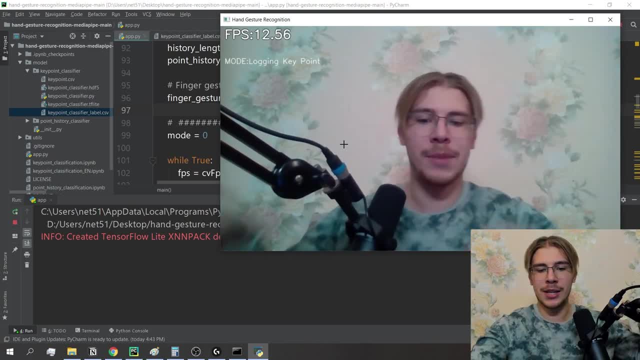 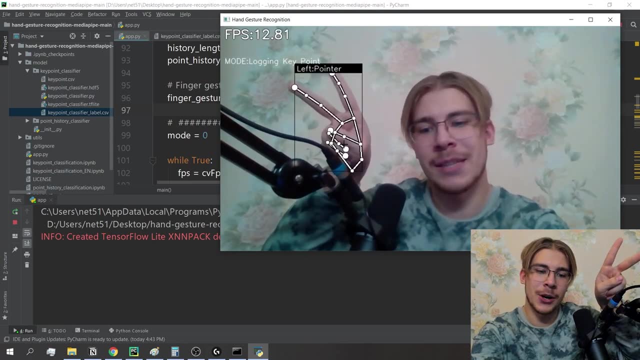 you can do this thing again, like press k under the logging mode and be like, okay, like it's struggling on my left hand, like this is a, this should be like uh, you know this should be a peace sign, but it's saying it's a pointer, let me press four. so i'm like literally like pressing my keyboard again. 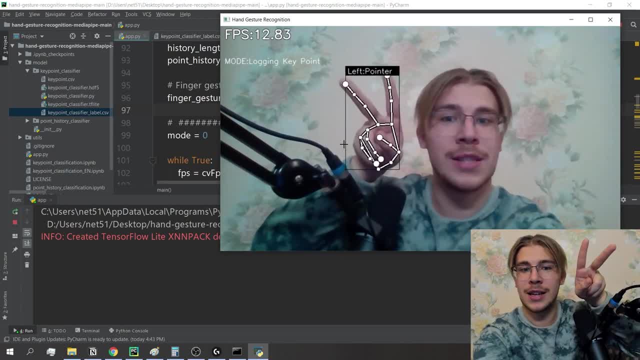 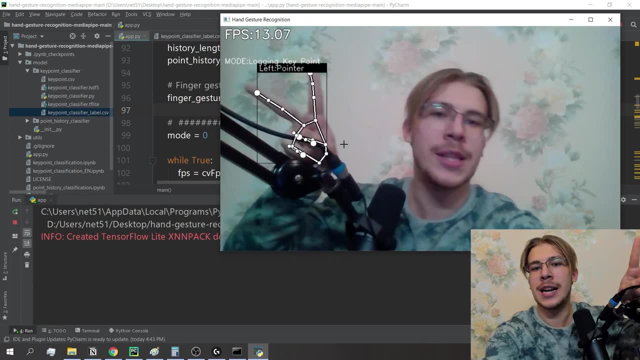 like just like bashing you like four four, four. as you can see, i could press like number four four, four and then train with that data and that that that should help because, like you know, you're feeding it more data. um, last thing that i want to show you is: 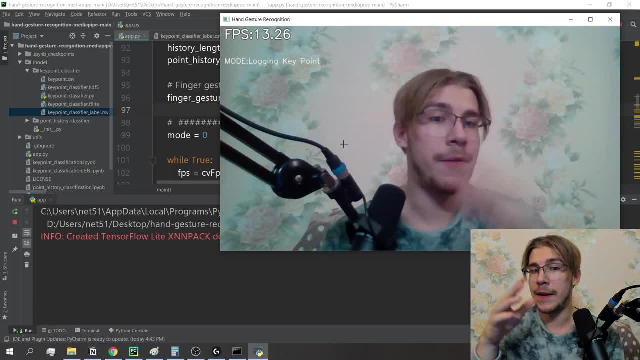 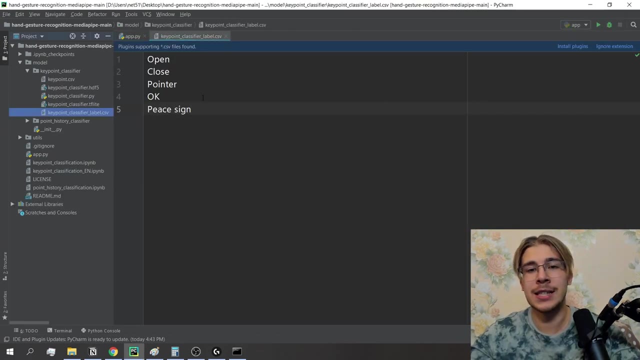 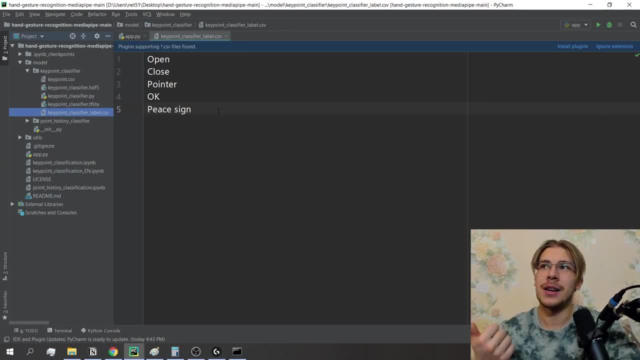 like, do something completely new, like, let's say, we want to have the, you know like thumbs up, thumbs down, and a rock and roll sign like the horn sign, whatever it's called. i associate it with the rock and roll sign, so we'll just roll with that. so, as you can see, training, that model is. 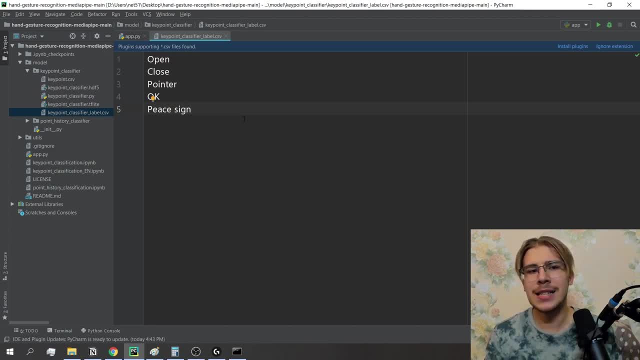 like really, really quickly, and the main kind of bottleneck in this case is is like the data. so, in order to do that- like we actually in this case, by the way, we we haven't like when we've added the new class, we haven't like kept an old model, we've completely retrained the model from scratch. 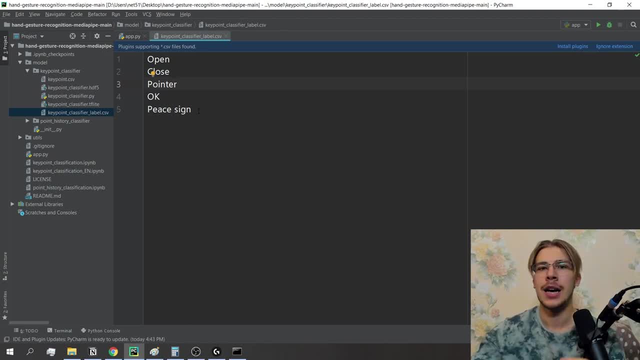 just the new data set that like included the new examples. so to add, like these new classes, we kind of have to do like low key the same thing. so first thing i'll go and do is i'll go into that csv file here and i'll just delete everything here pretty much. 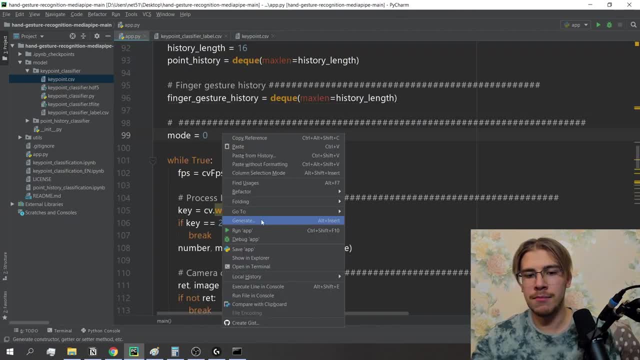 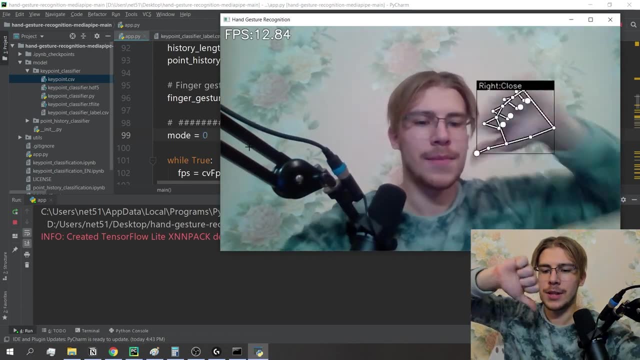 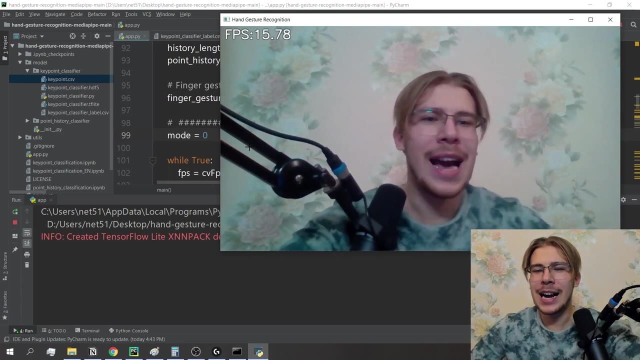 so it'll be completely empty. then i'll launch the training script again and i'll and i'll collect some training data. um, so let's say we'll do like thumbs down. hopefully this video is like a thumbs up, but like they're just for the playing around with it. actually, i don't like. i don't like thumbs. 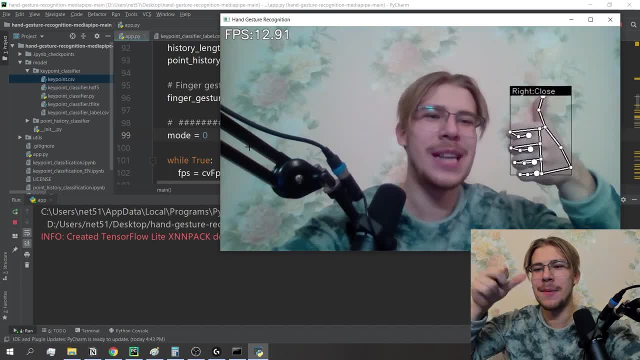 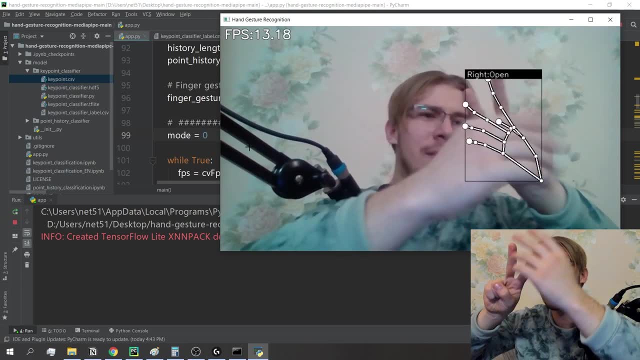 down. i don't like the sound of that. let's just do peace sign, thumbs up and the rock and roll sign. can we do that cool? so, uh, i'll say, okay, let this be like the peace sign, but never mind that it's already saying that i'm collecting like a new data set, so i'm keep pressing like zero, zero, zero. 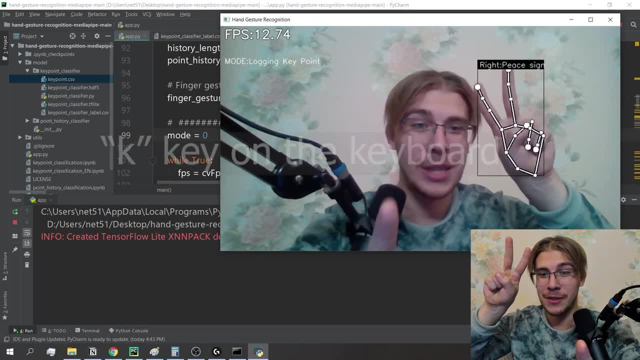 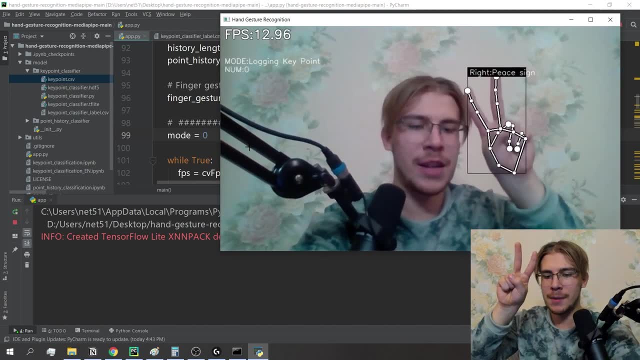 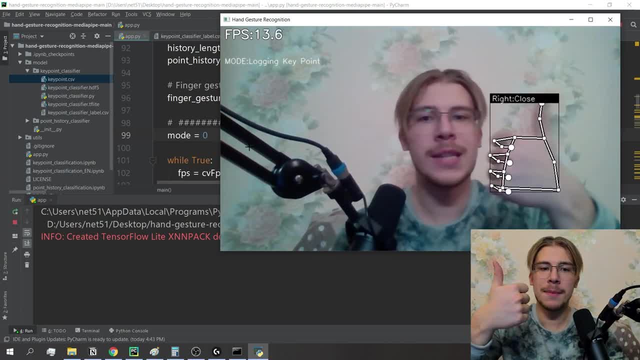 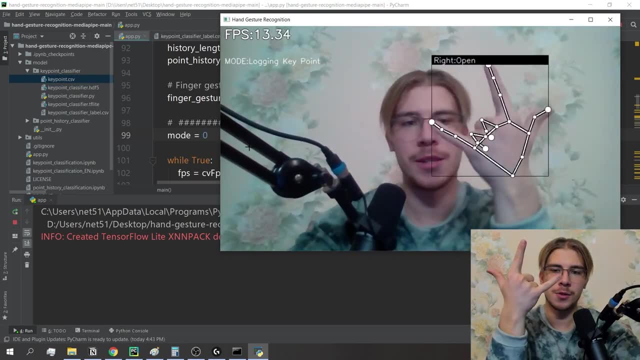 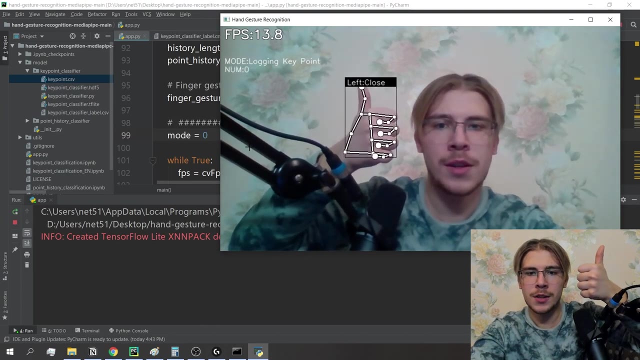 sign. now let's do thumbs up like i'll start pressing one. now let's do the rock and roll like horn sign, i'll start pressing two. and for more accuracy, you know you may want to add like the left-handed examples, also i'll press. i've just added a couple wrong labels, as you can see. 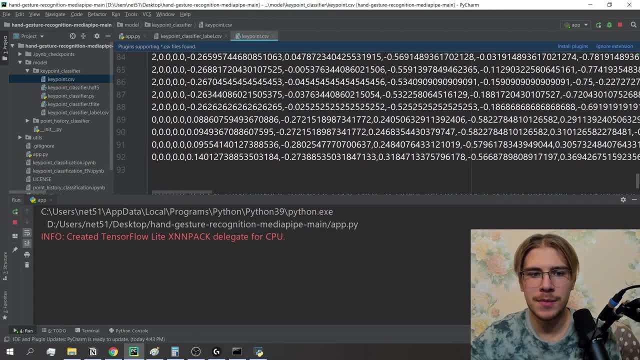 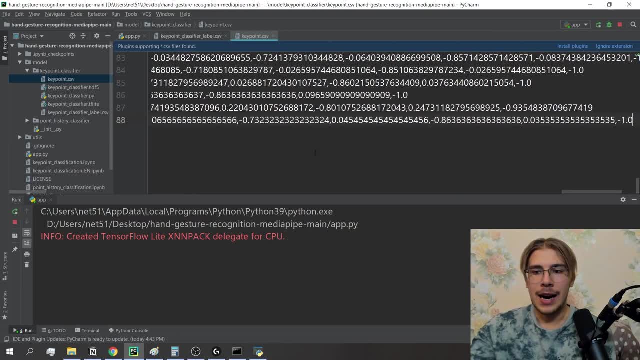 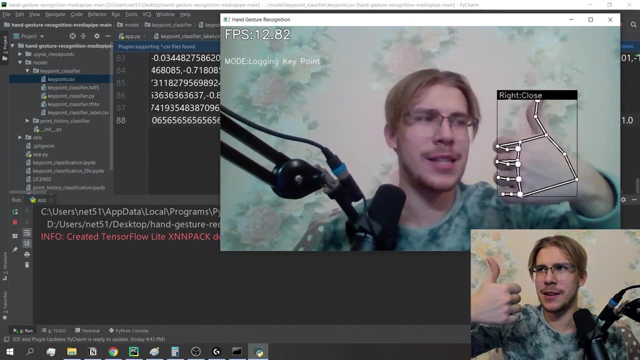 i have. yeah, but that's not a problem because i can just go and erase all of them, because i did the- uh, i did this thumbs up with an actual index. you know, i did like this thumbs up with the index of zero, but that's for the peace sign. you know what i mean. so let's do some more like left-handed, like. 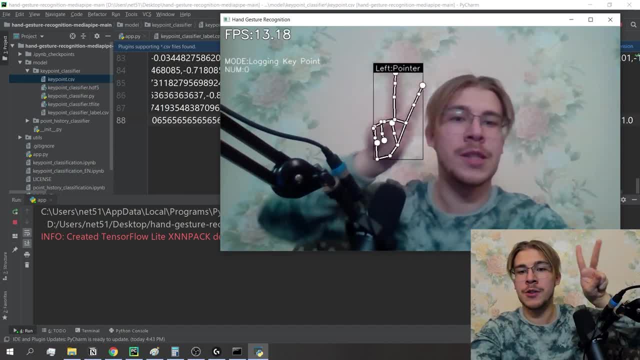 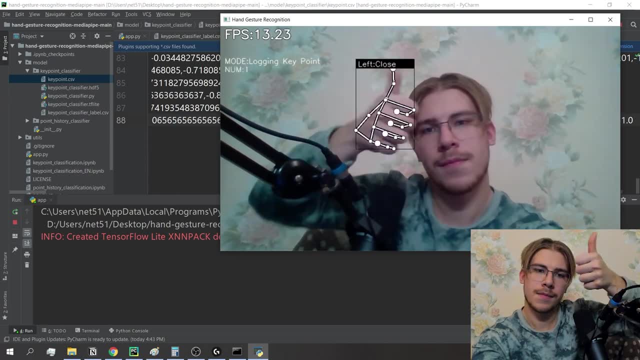 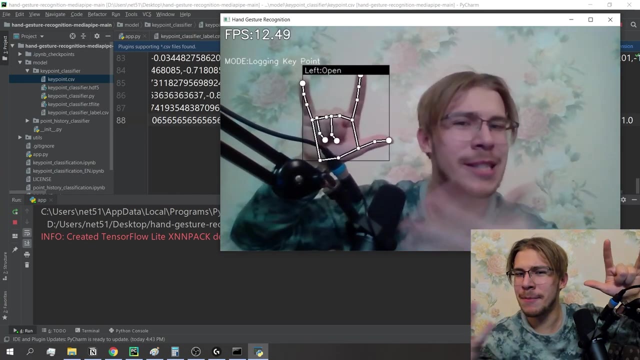 peace sign: um zero, zero, zero, zero, zero, zero, zero. left-handed um thumbs up and uh, the left-handed like rock and roll sign. by the way, if any of these signs like mean something different, like in your part of the world, like let me know. like i'd be curious to know what they mean to you because, like 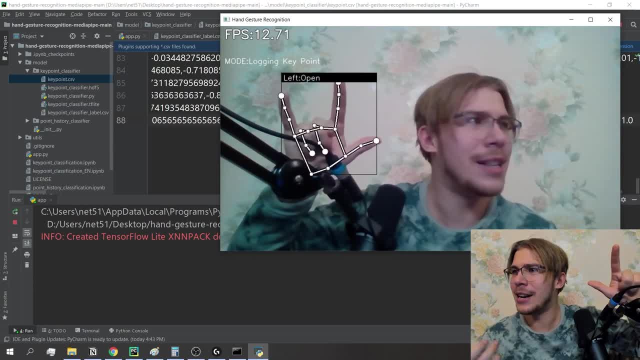 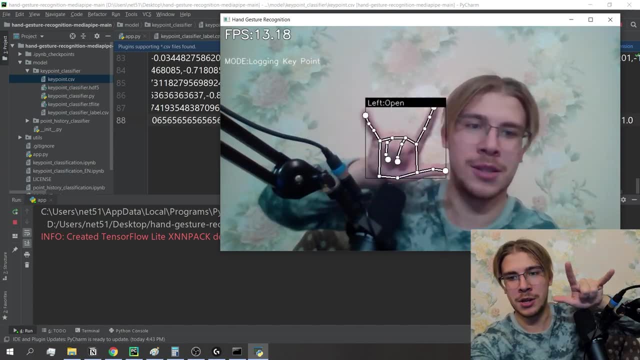 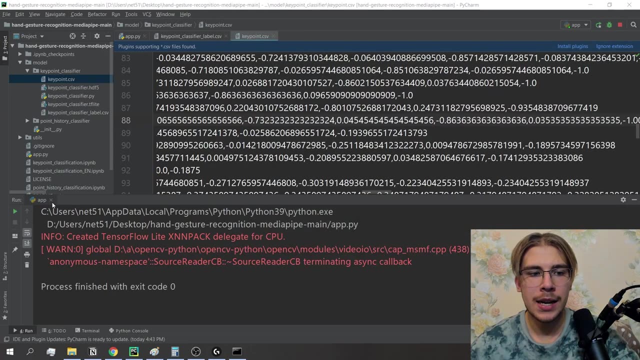 i kind of did some googling before that and, like i don't know, it's there's, there's a lot of hand gesture info, uh- that this video does not need to be longer than it already is. i have a feeling. so okay, um, so i've collected the data. okay, um, go and check out, like our training file, as you can see it. 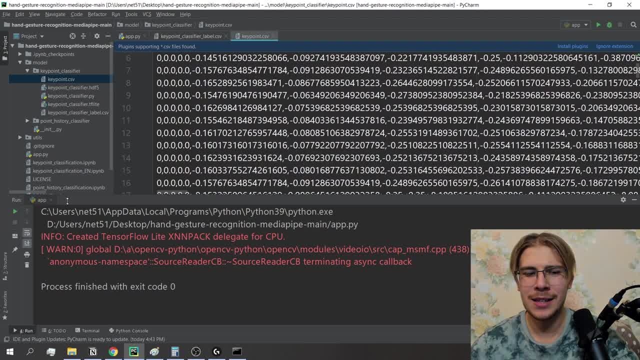 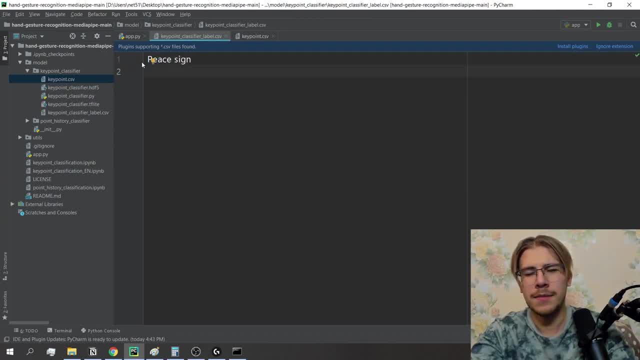 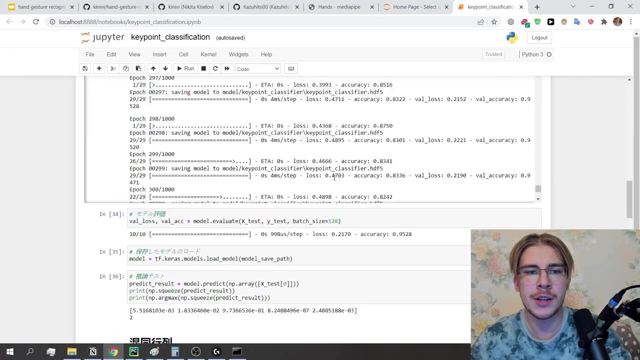 takes me a lot of time at all. it's just like takes being, kind of, takes some attention and stuff like that. i'll edit the labels file now for peace sign, um, thumbs up, rock and roll sign, and then we'll go into the jupiter notebook here again and just press, sell and run all cells again. 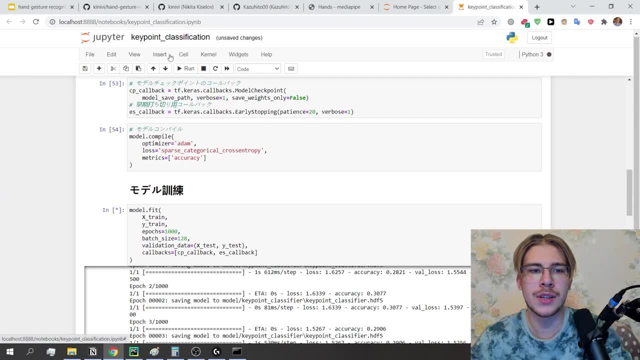 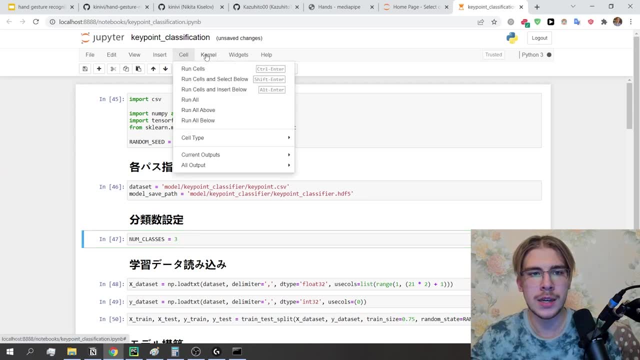 oh no, actually one, just one thing. one thing we need to edit here is the number of classes. so like i'll go and i'll say, uh, kernel, um, restart and run all. so yeah, just like, don't forget to edit the number of classes. that's, that's a good one, for sure. okay, so you can see it's starting. 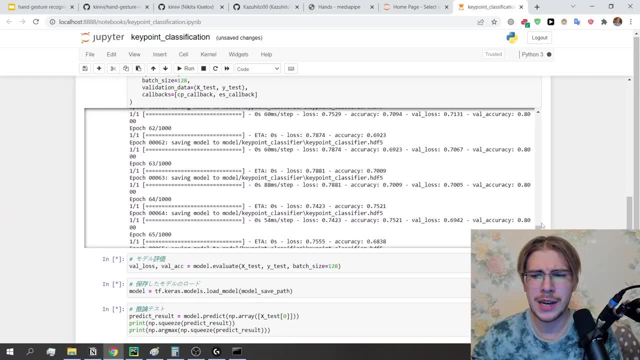 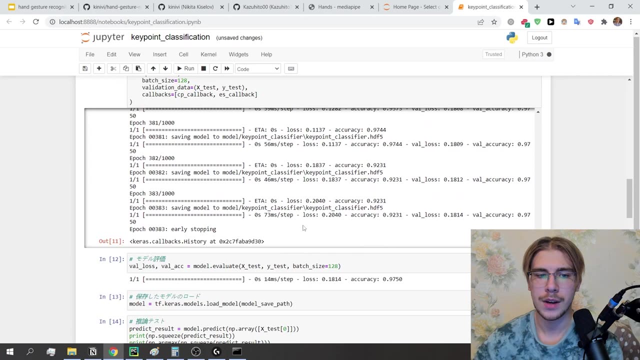 training. um, i have you know we haven't collected a lot of data, so i'm assuming that it's gonna go by pretty pretty quickly again. all the training i think is also happening on the cpu might be wrong, but, like, i'm pretty sure it is okay. so you did the early stopping and it saved the model. and after, 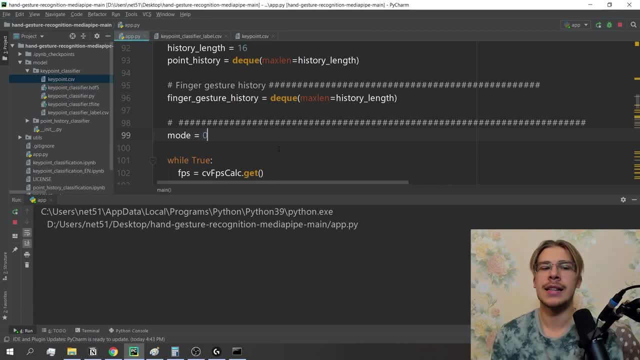 that is done, we can just go and launch the app. uh, again, like this file. because, like, the model file has been updated, so which is like this file right here? so now it should be able to do all the new detections. so like that's the peace sign, thumbs up sign. 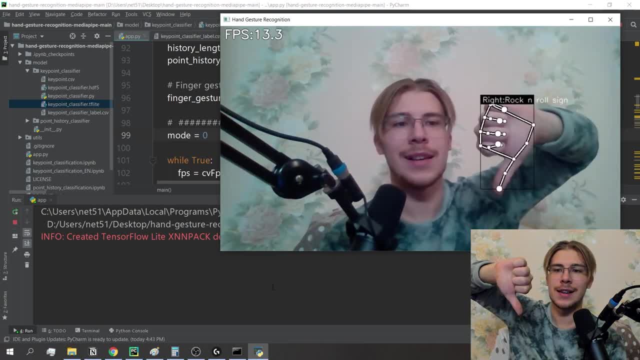 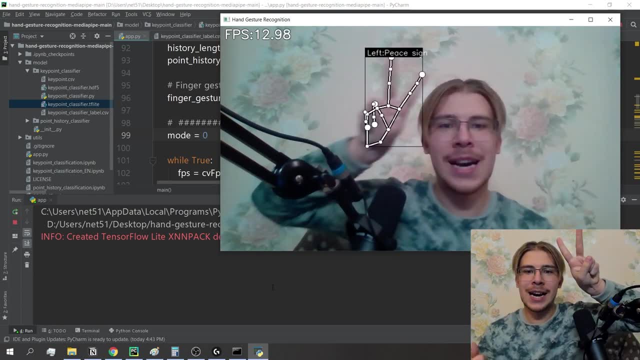 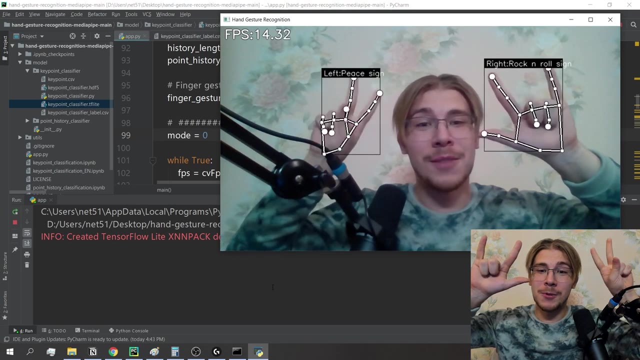 rock and roll sign. as you know, we don't have a thumbs down, so like even that's a rock and roll sign. um same thing on the left hand: peace sign, you know, peace sign, uh, rock and roll sign. brock roll sign and thumbs up: rock and roll. peace sign and rock and roll sign. 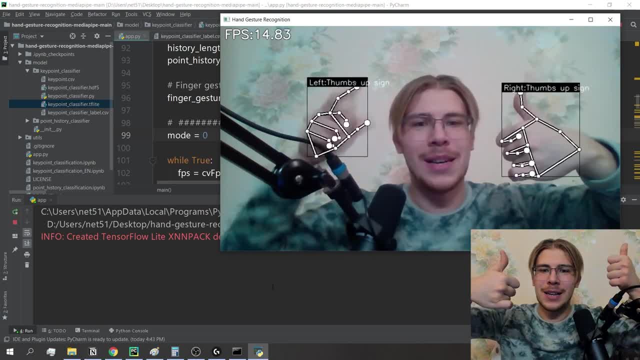 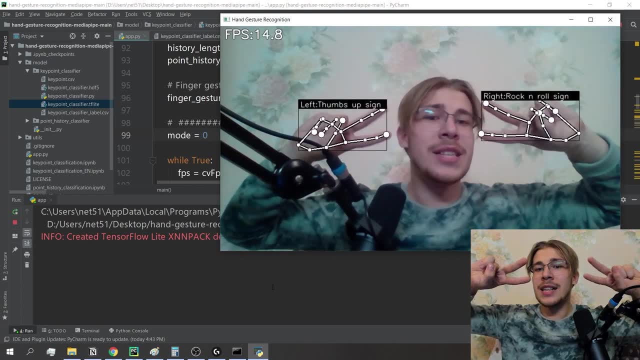 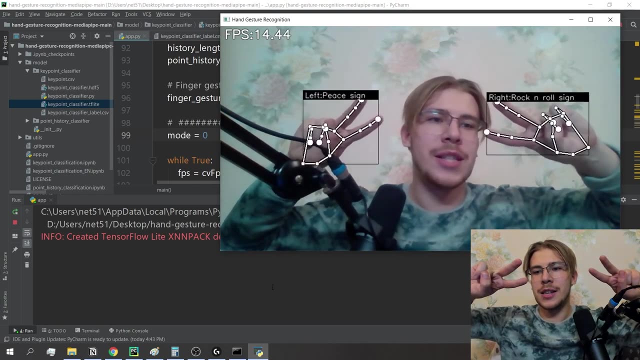 peace sign, rock and roll sign, thumbs up, uh, thumbs up sign, uh, peace sign. and you know, whenever you get like this, edge cases and like problems, any problems with like accuracy and stuff, um, you know you can just like go and again do this whole thing or like, hey, like 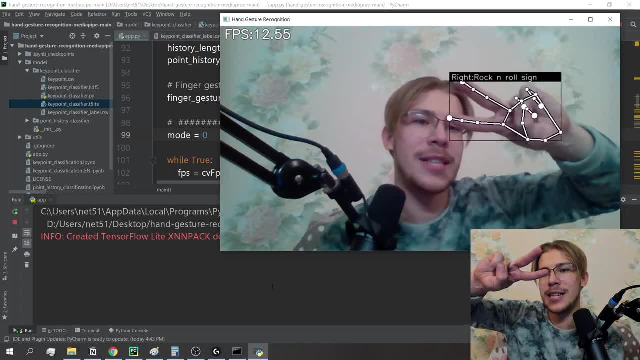 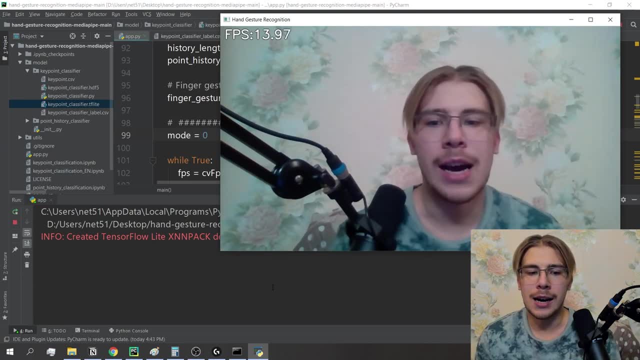 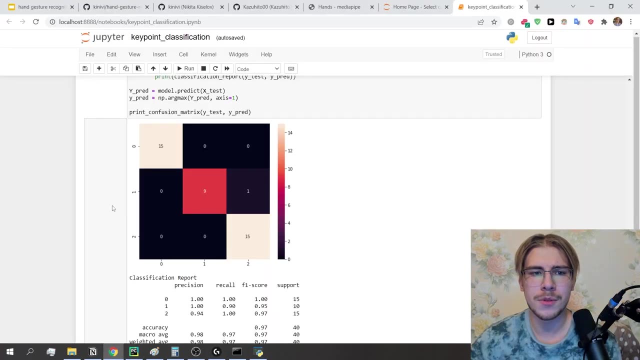 let's train it like this, is this like that, that's like i don't know, like the piece sign and just add more data that looks like this, but with the index of the piece sign, and, uh, just run the training again. uh, yeah, pretty much the only thing that i've mentioned here is that, like to you know you. 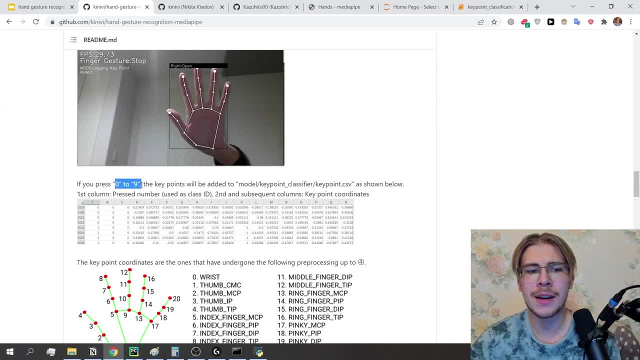 may just like use some. there's um. if you want to have like more classes than 10 here for your hand gestures, you can just like write some python conventions in the code to just be like you know the number of the key pressed, say like plus 10 or something like that, you know. open up the whole new. 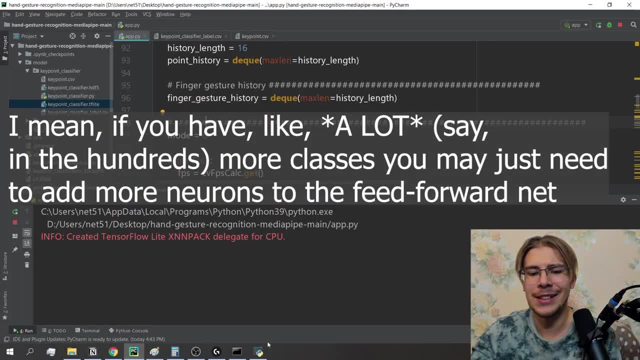 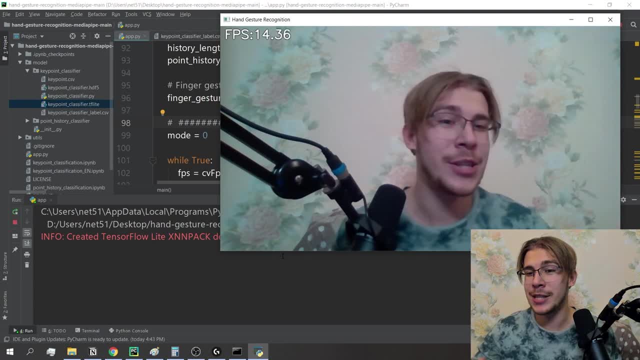 array of numbers, but i don't think there's any like a limit to how many gestures you can have. as i was saying, the person whom i was helping did like that for the russian sign language. i don't think there's any like a limit to how many gestures you can have. as i was saying, the 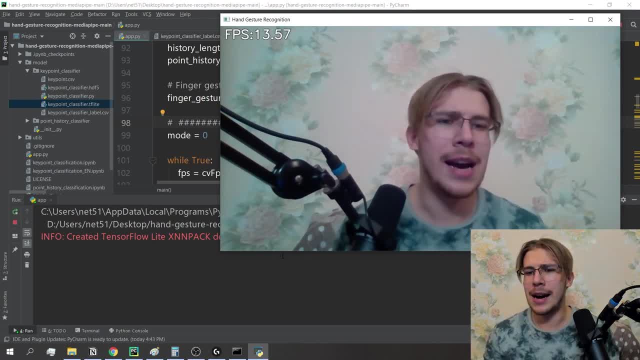 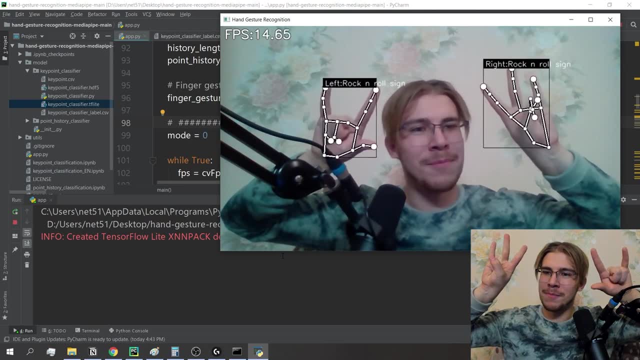 russian language is like 33 letters or something like that. uh, so you can really do a lot with it and uh, yeah, as you can see, like it's like pretty cool. we're like rock and rolling and piece signing and thumbs up in here. i'm kind of like hinting at something here, guys, you know. 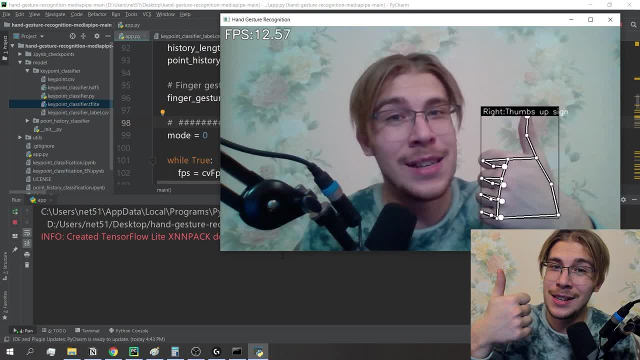 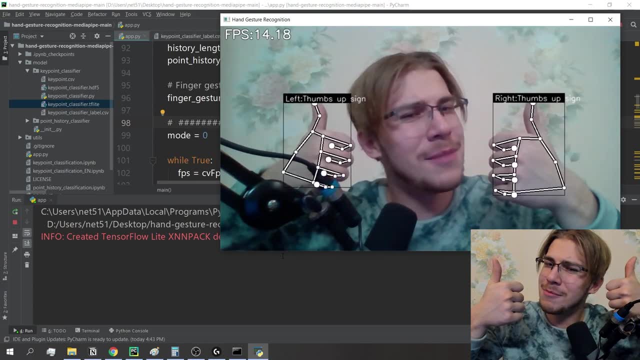 i don't, i don't know what i'm hinting at, but i'm hinting at something. what, what can that be? i don't, i don't even know what i'm hinting at, but can you guess that i'm not just subtle, you know? 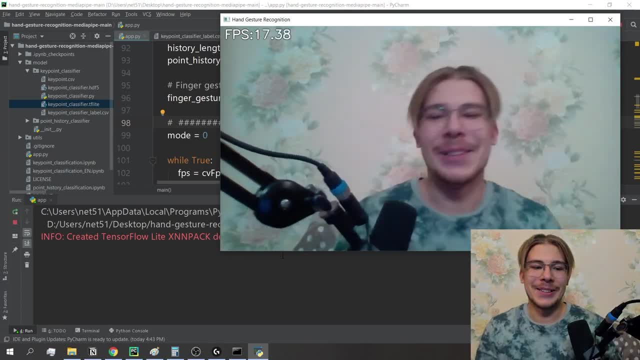 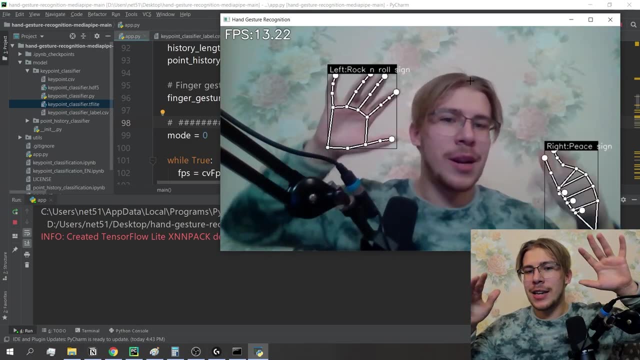 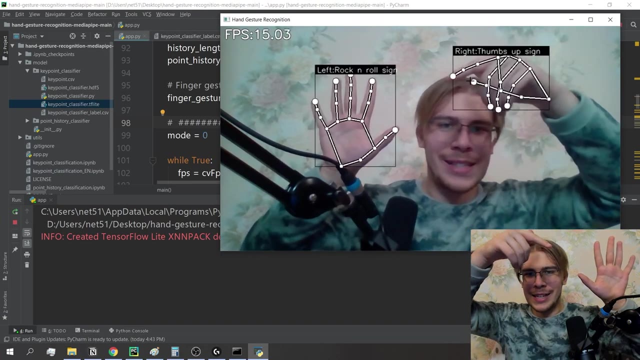 you know, okay, okay, fine, uh, but yeah, that's pretty much. so. a few more things that are valuable to here. is that, like, if you want to like incorporate this into like your own project, like, yeah, some ideas? is that you know, uh, what what the former student did is like she kind of she, she did like 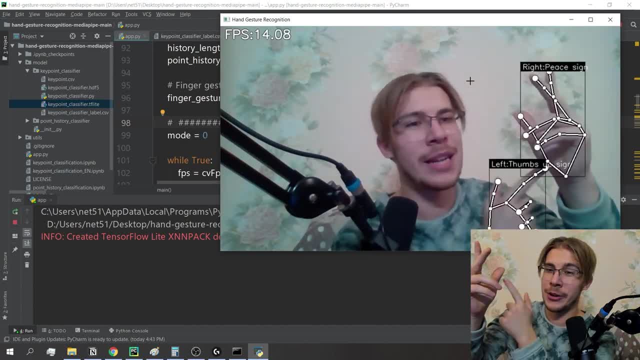 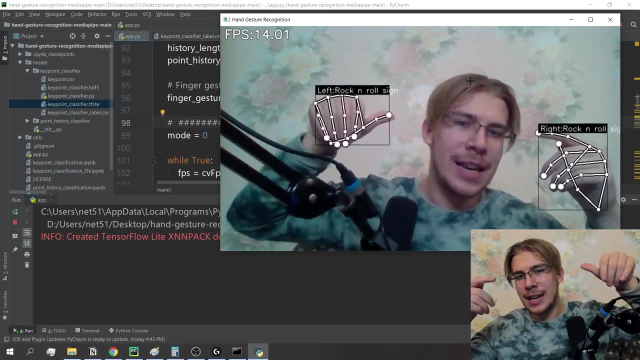 you know, she focused, like, as i was saying, gesture recognition, like on one hand, for instance on the right hand, and for the left hand she like hard-coded some rules that like: if you move your palm on a certain way, then it does like, or like, if you move your finger in a certain way, then it does like the.